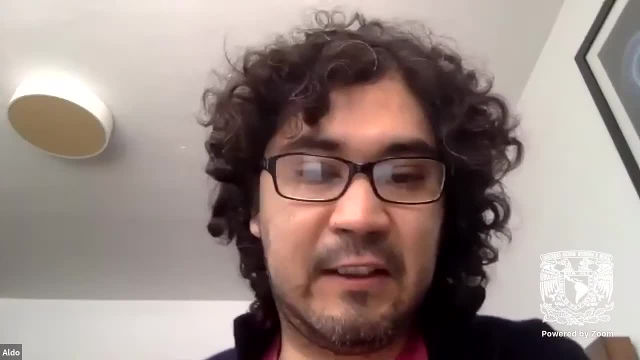 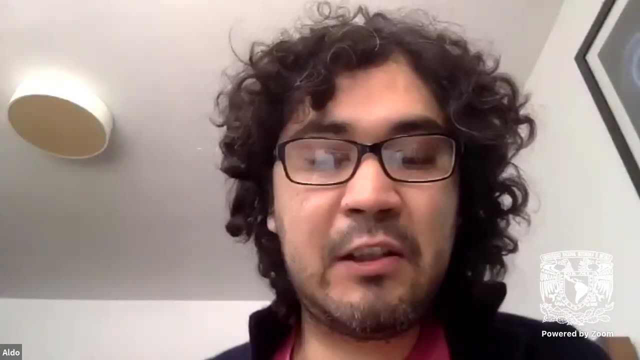 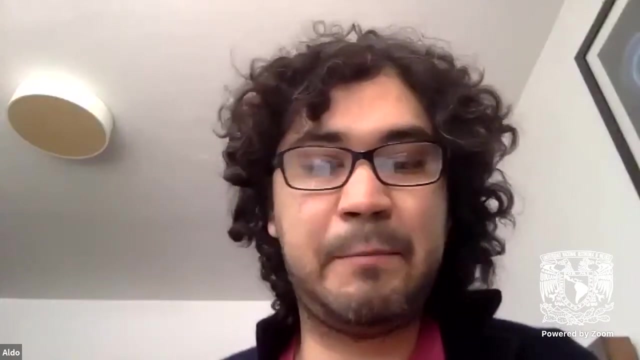 of early-type galaxies by studying the evolution of the stellar mass-velocity dispersion relation in early-type galaxies. He also has been collaborating a lot with the people in the University of California, Santa Cruz, with Alexei Litov and Kevin Bundy, And they've 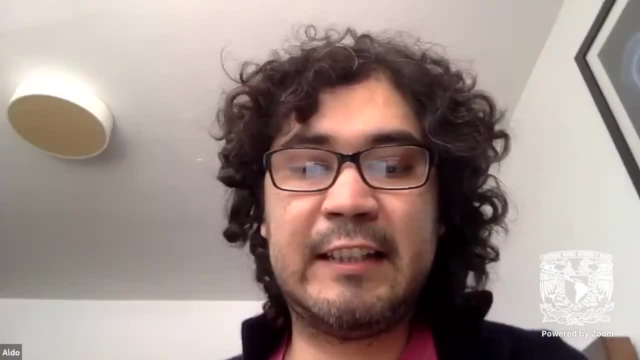 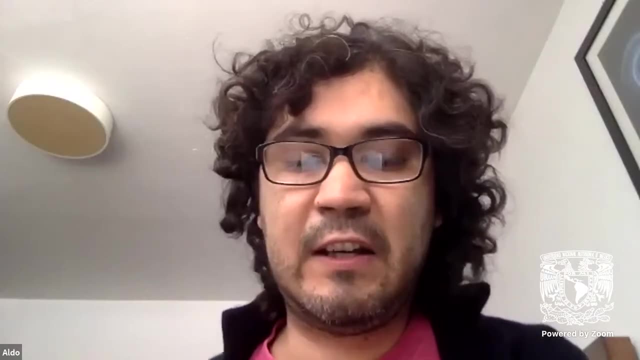 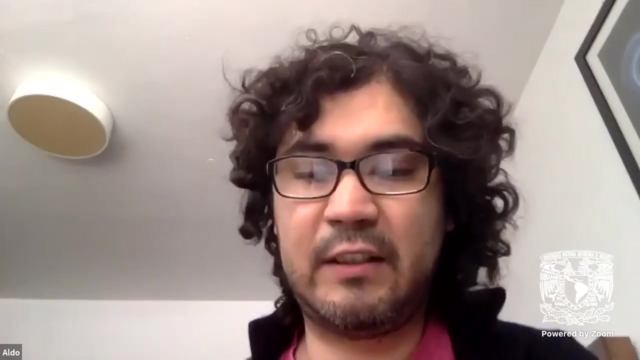 been doing an analysis of the radial distribution of the stellar properties, such as the age, metallicity and velocity dispersion, And also- this is a просpecture dispersion- iB35,, for example, of early-type galaxies comparing Manga, and so this is a survey that everybody knows that we are also working. 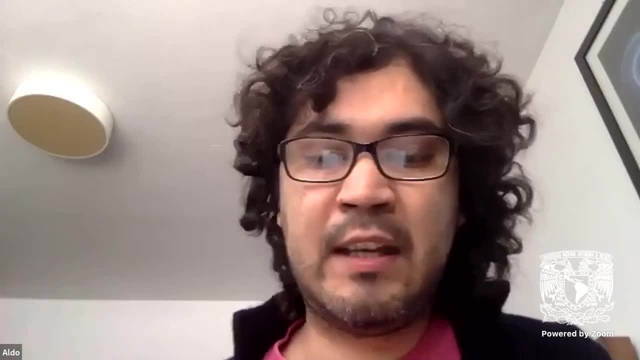 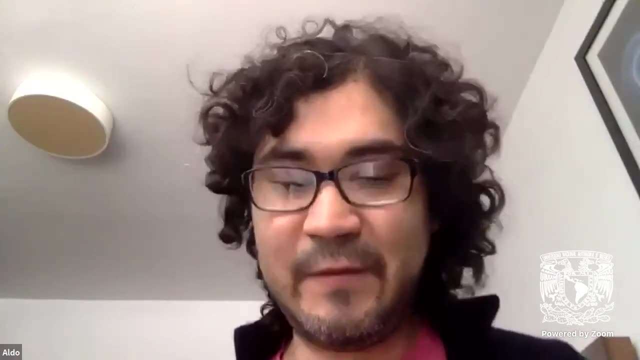 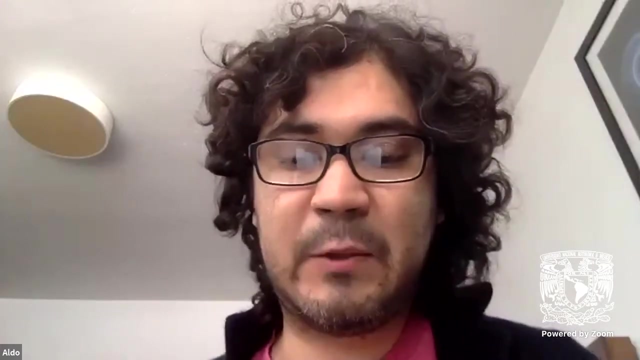 here and by comparing observations of Manga and 66 TNG population. So basically, he is like an interface between observations and simulations, And he has been also awarded Maria Slodowska-Curie Grants in Data Science and Machine Learning to carry out the Accervation and Implementation test. 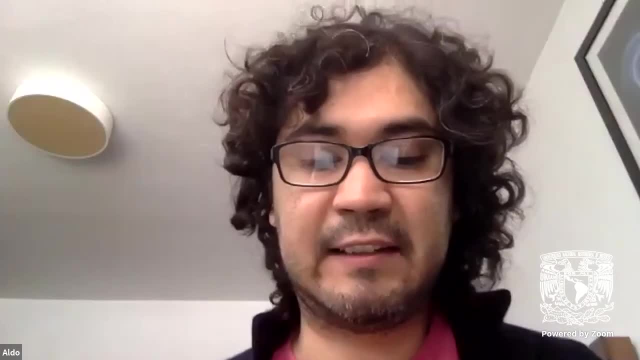 He has been also awarded with the Maria Slodowska-Curie Grant in Data Science and Machine Learning. to carry out the Acc examination, And quickly. we wanted to raise some particularly helpful but extremely mysterious question about the projects with Alexey Letov. 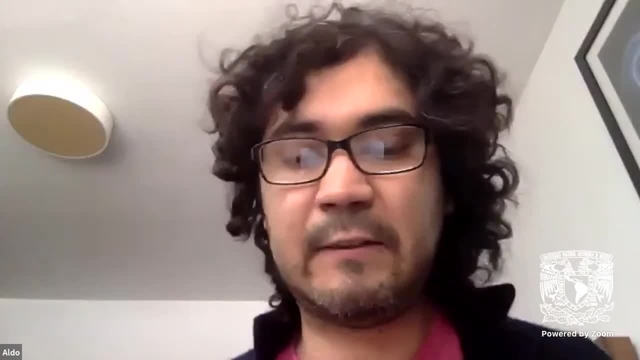 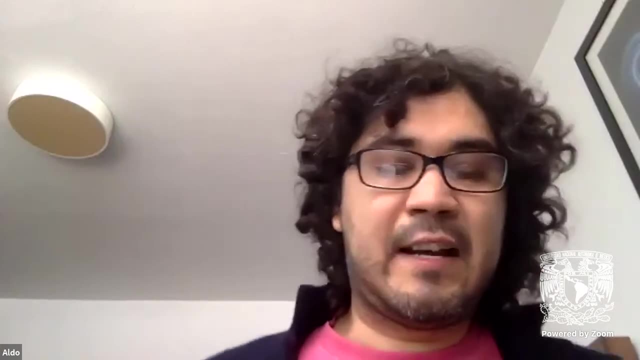 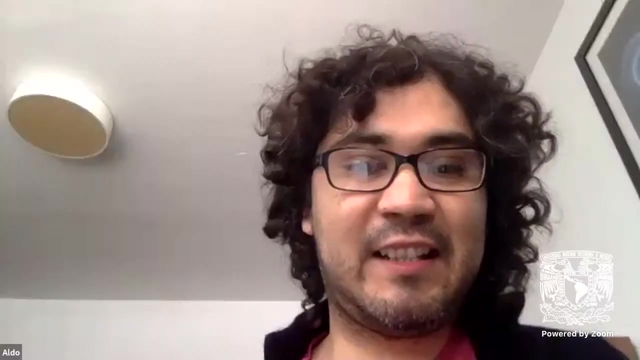 but to training a model based on simulated galaxies of the illustrious TNG and exploring machine learning algorithms. Okay, So I hope that I say everything that I need to say And it's all yours, So please go ahead, Carlo. Okay. 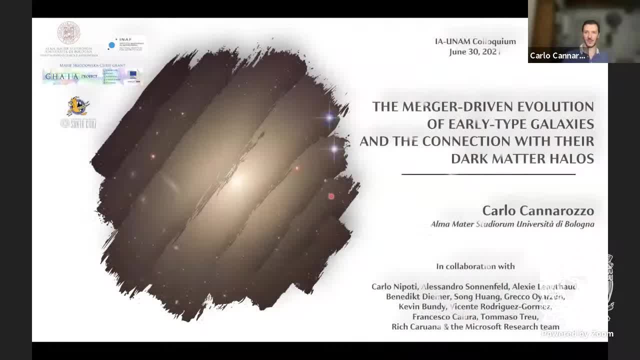 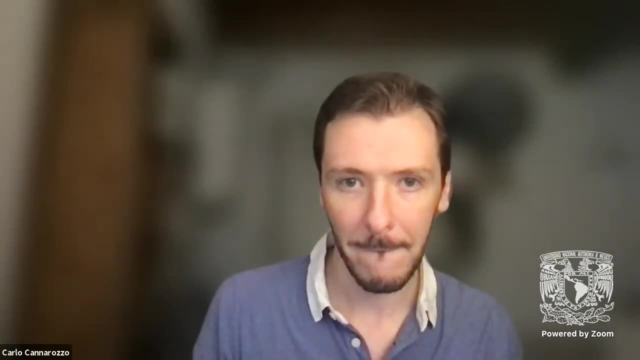 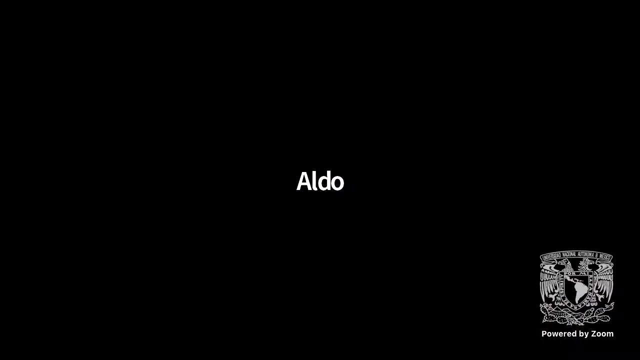 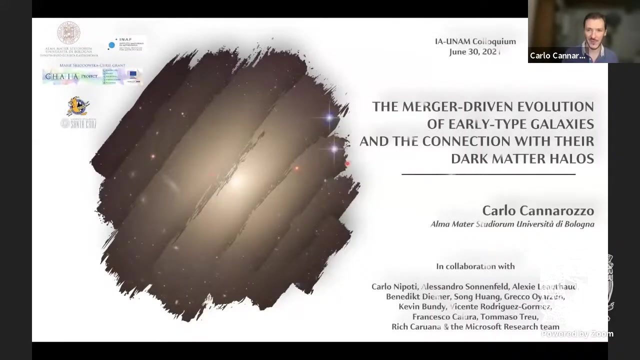 Share my screen. Do you see my screen? Yes, And my laser pointer? Yeah, just a moment. Oh, sorry, Sorry, We lost it. We lost the presentation. Okay, Do you see now? Mm-hmm, Okay. 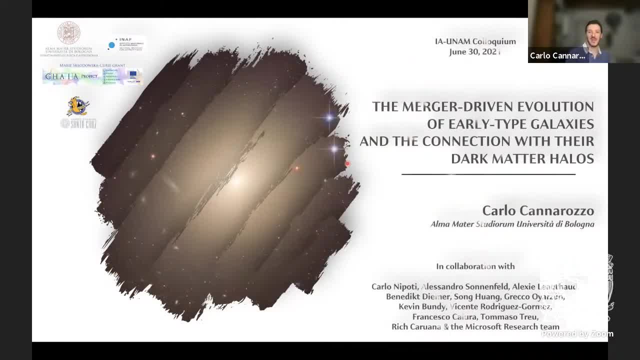 Yeah, Okay, I start. Thanks, Aldo, for the nice presentation. Again, hi to everyone. I am Carlo Cannarozzo and I got my PhD in astrophysics on May 24 at the Alma Mater Studiorum Università di Bologna. 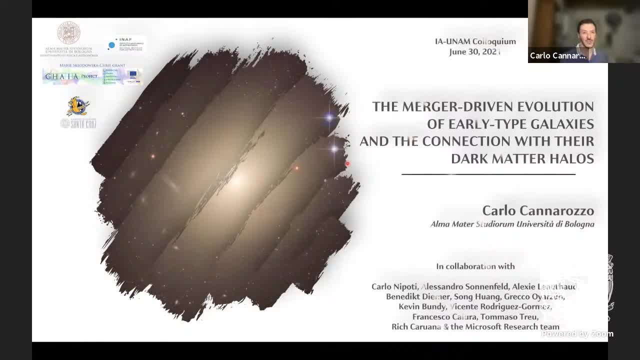 working with Carlo Nipoti and Dr Alessandra Sonneveld from the University of Leiden in the Netherlands, and with a great collaboration with Alexey Letov, Kevin Manley and all the other researchers here listed here below at the University of Santa Cruz. 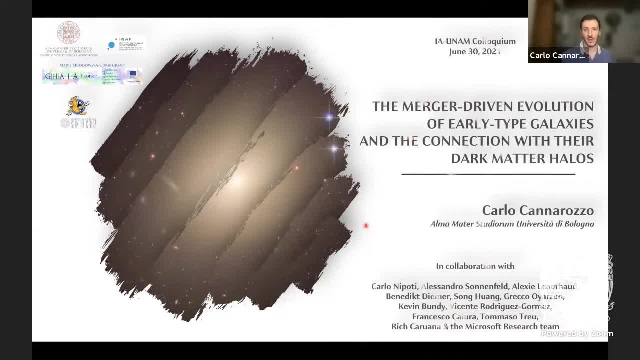 in California that I visited during my PhD three times for more than eight months, And today I'm going to describe you, illustrate you, three different projects I'm involved in in the context of early-type galaxies, the emergent revolution and the connection between galaxies and the dark matter helios. 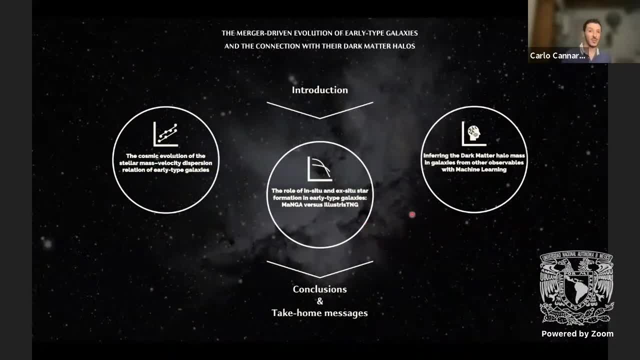 The structure of this presentation is the following: After an initial brief introduction about that, provide an overview of all the early-type galaxies, their formation and evolution and physical properties. I go through the details of the three different projects and then I sum up everything in my conclusion and I leave you. 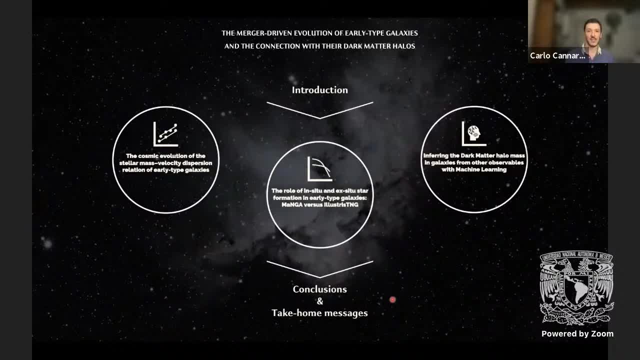 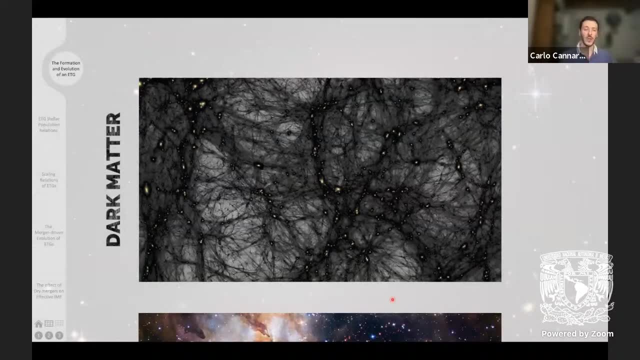 with my take-home messages of these works, Let's start. The first key ingredient we need for forming a galaxy is definitely the dark matter. We know from the lambda-CDM model that after the big bang from a homogeneous distribution, dark matter started to collapse. 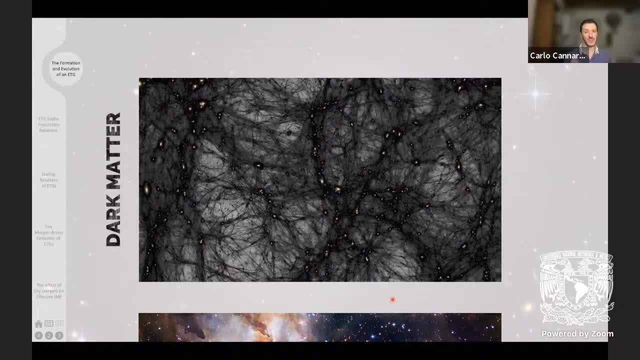 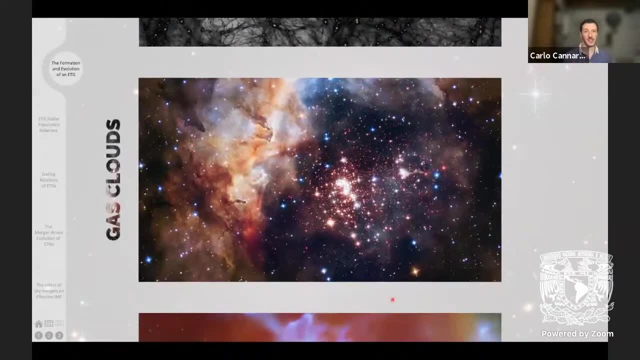 under its own gravity into a scaffolding of clamps and filaments that we know as the cosmic web. At the center of these dark matter densities, called the dark matter halos, variants started to migrate, aggregating into gas clouds and these gas clouds cooling down. 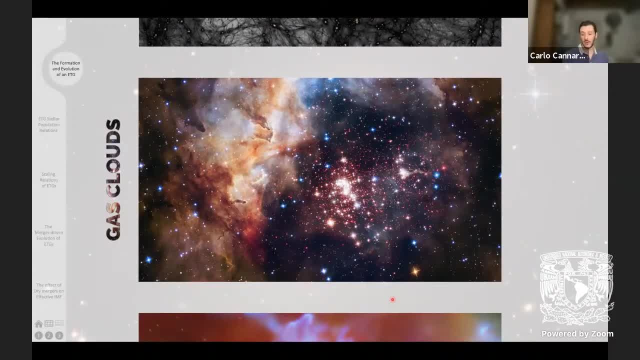 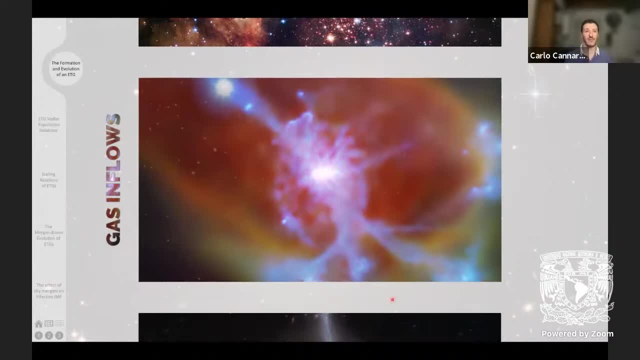 their temperature collapsing give birth to the first generations of stars. Here we have the first generation of galaxies, proto-galaxies, that have been formed a large amount of cold gas but that also accrete from the surrounding cold gas inflows that feed. 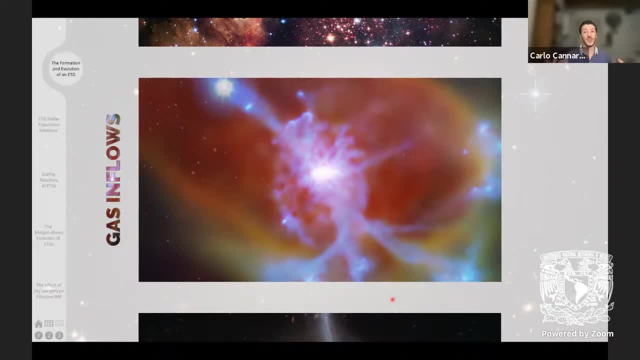 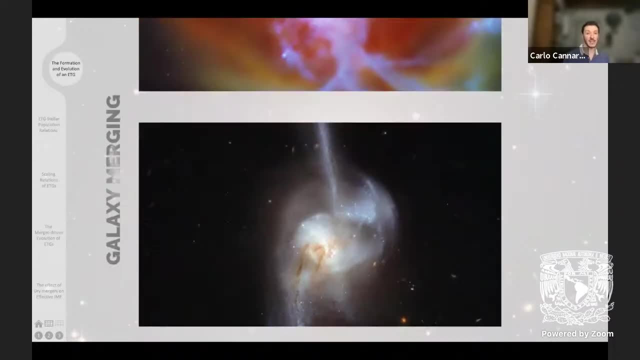 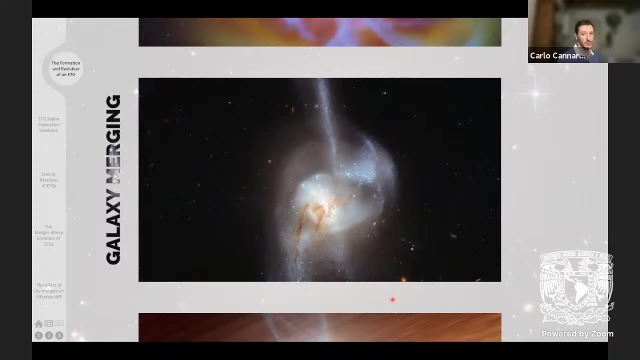 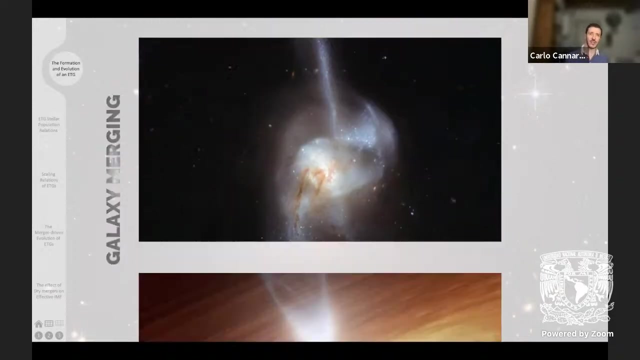 both the galaxy that form new stars, new generation of stars, and feed also the central supermassive black hole. uh, during its life a galaxy may experience several and several galaxy merging that can dramatically change internal physical properties and can trigger also new star formation episodes um. another key protagonist in the in this movie is definitely the central supermassive. 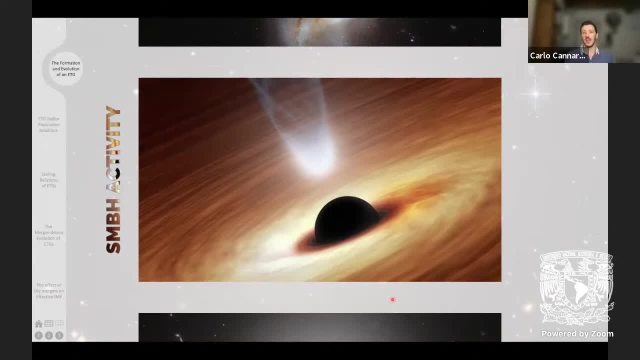 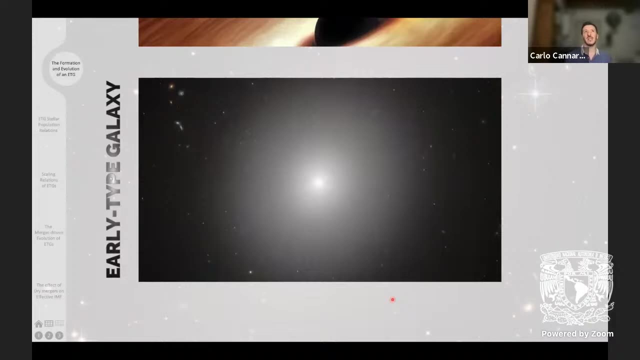 the coal that through its radiation- uh it- it is capable to blow out part of the gas, causing a halt in the star formation activity. and once all these gas reservoir is exhausted, um, we end up with a system that basically experience our passive evolution. and the only way to 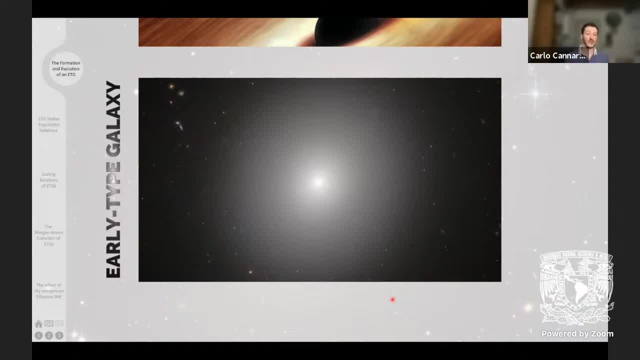 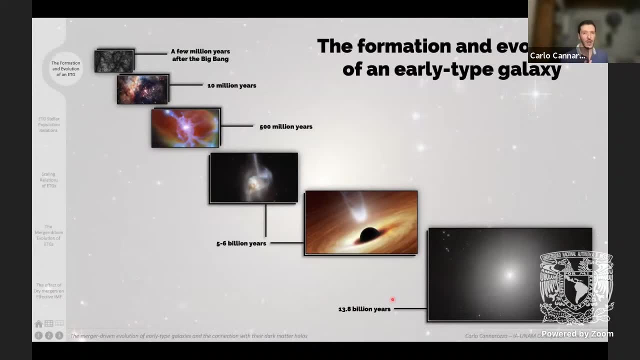 change internal properties into is to interact with the environment and interact with other galaxies through galaxies, through mergers. the entire scenario that i've just described you, uh, is a very long, and it may take a giga and giga years, even more than 10 giga years. 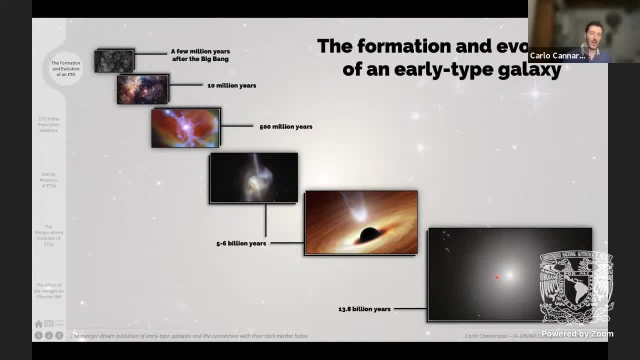 at the end of which we end up with an early type galaxies. the important thing that should be underlined in this a very complex chain of events, is that there are, during a this video years, um, tens and tens and tens of physical properties that co-work, co-act together. 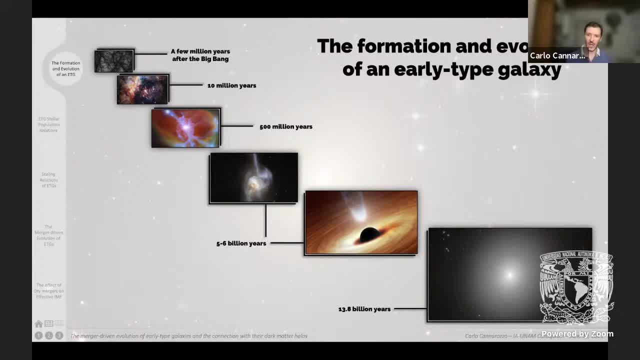 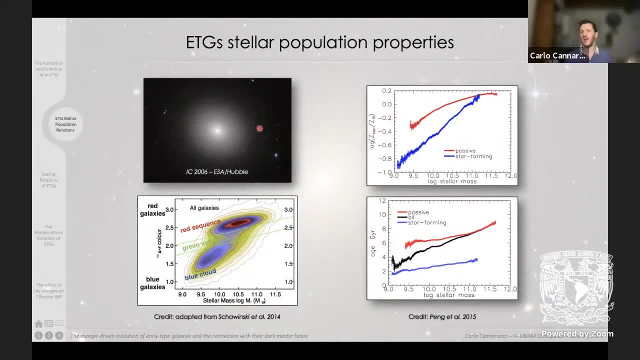 for forming and letting evolve these galaxies. morphologically speaking, as you can see from these photo, early type galaxies are very simple system in the sense that they are characterized by roundish or elliptical shape on the bottom left panel. here you have a color mass diagram, uh, drawn from chavisky child 2014, populated by both late and early type galaxies, and although 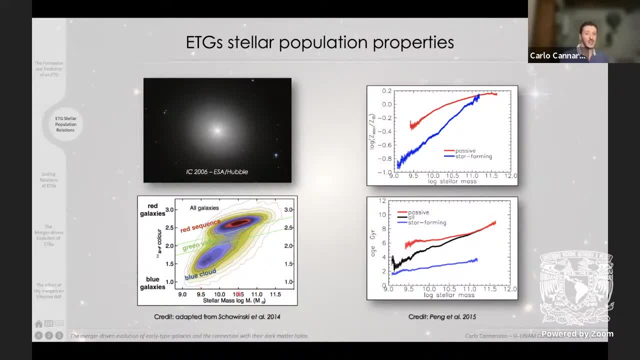 both kind of population are spreaded over the entire range in mass and over the entire range in colors. early type galaxies tend to occupy, uh, the red red spot of these plots, and also early type galaxies tend to be the most massive systems, as you can see here the fact that etgs are characterized by 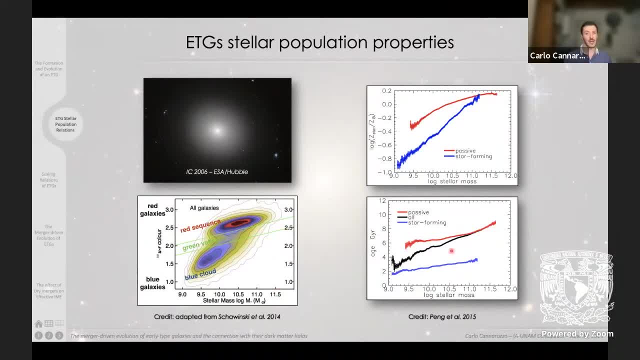 these red stellar population can be explained in terms of these two other results here here, as a function of the stellar mass, you have on the top panel the stellar metallicity and on the bottom panel the age of the of the stellar population. and what is this? is it found for early type galaxies? 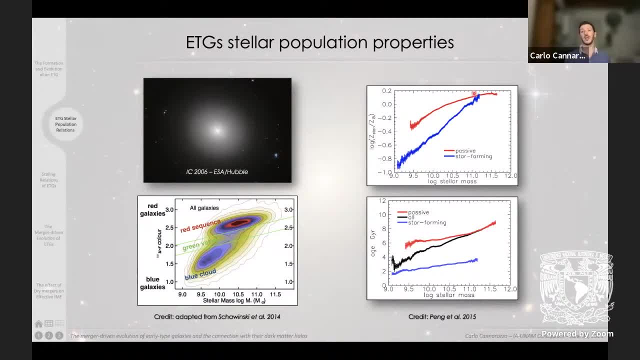 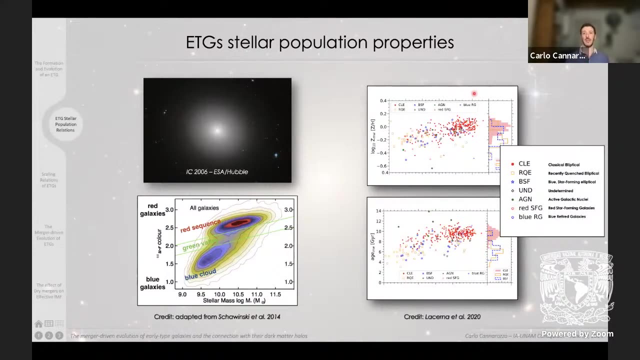 that this kind of galaxies, on average, are characterized um from uh, are characterized by very metal, rich stellar population and old stellar population, and these results are, of course, uh um corroborated from uh the state of the art and most more recent observation uh um occurred with the manga survey, for instance. these are: 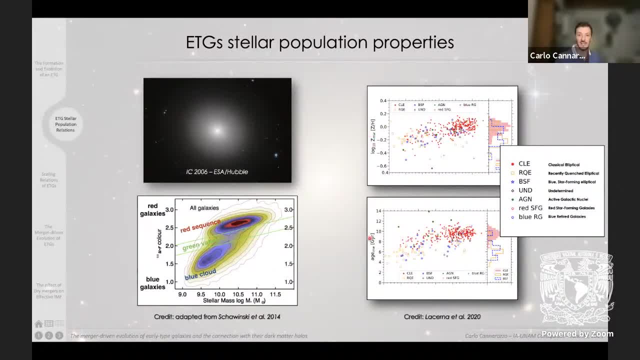 the same plots of before. as a function of stellar mass, you have the metallicity and the age from lacerne et al 2020 and, regardless of the um, the separation that disentangled that the authors applied in etgs to classify them as classical elliptical, the resonant sequential elliptical or other kind. 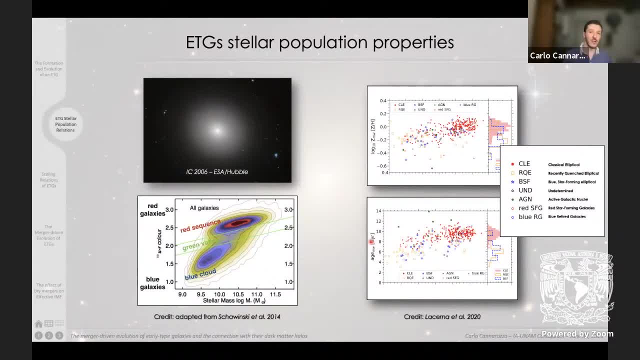 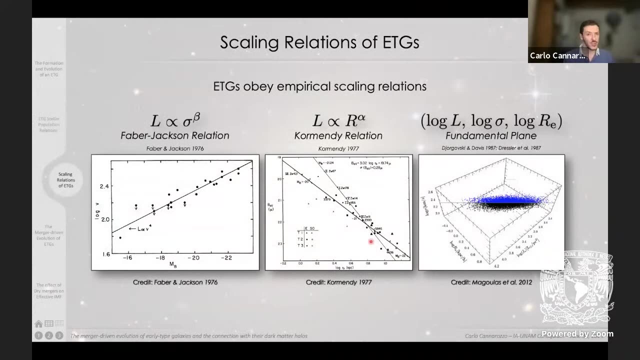 of subclasses. what is should be underlined is again that this kind of system are composed by stars with a very metal rich content and or old stellar population. uh, historically we know that early type galaxies obey some scaling relations. in the 70s was found that the first two were the favor. 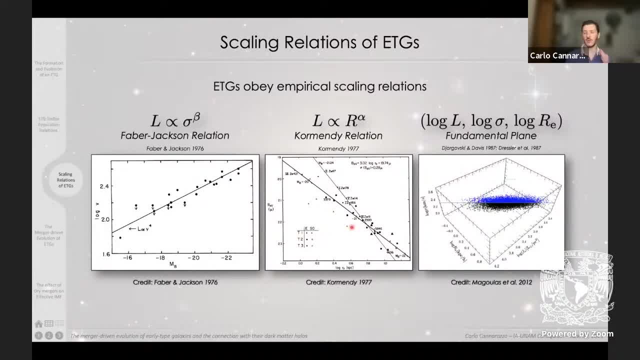 jackson and the common scaling relations that link the luminosity, or equivalently the stellar mass, to the velocity dispersion and to the sides of the galaxy respectively. and soon thereafter, in the 80s, it was discovered that these two relations are just two projections of a more general relation. 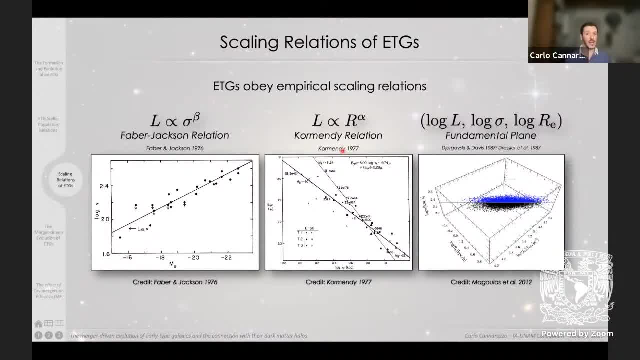 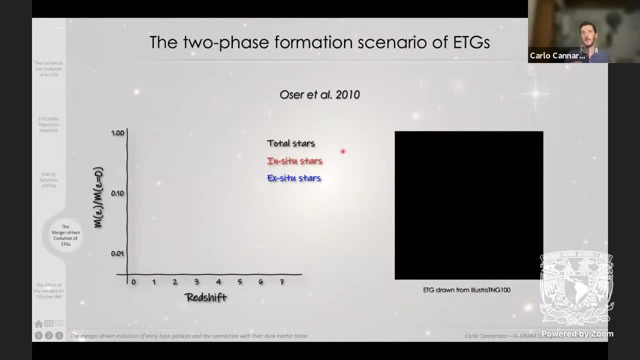 that is called fundamental plane, where all early type galaxies lie. at the beginning of this introduction i've i show you that the process for forming and evolving a galaxy is a very, very, very complex, but the stellar mass assembly history behind an early type galaxy can be easily summarized. 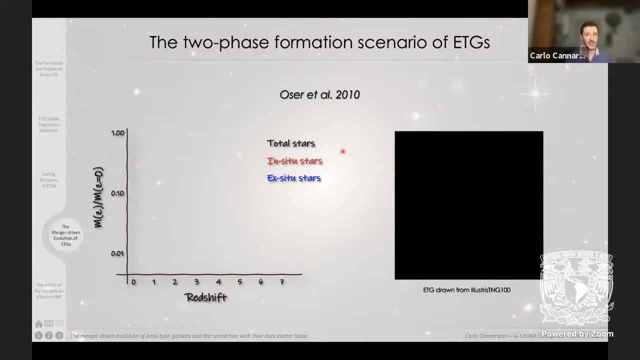 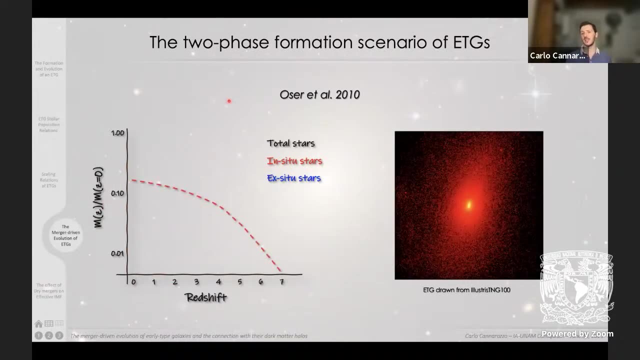 assuming the so-called two-phase formation scenario proposed by user italian 2010.. in this sketch here we have, as a function of redshift, the stellar mass at given redshift relative to the mass at redshift zero. uh, in the first stage of its life, an early type galaxy is. 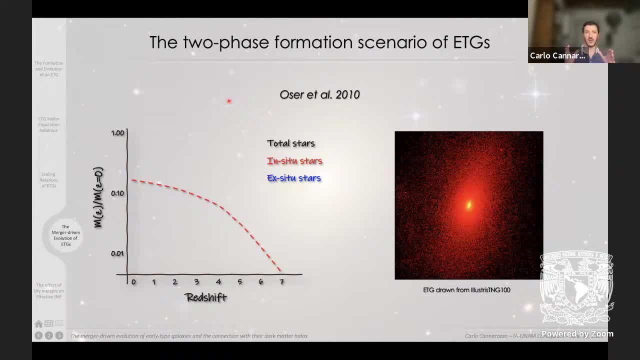 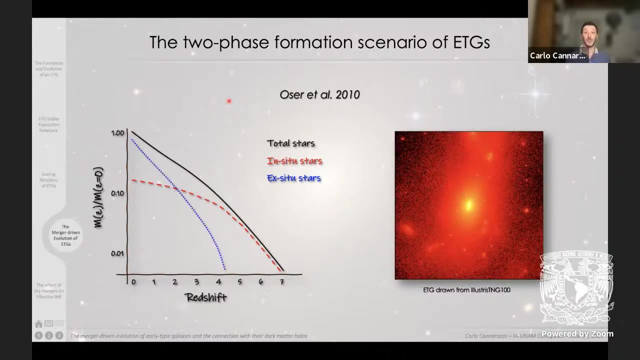 composed by this, called the institute component, so the fraction of star that was formed in that galaxy. however, as a consequence of galaxy equation processing and minor and major managers, the most dominant component from redshift to more or less up to the present day universe that can reach even 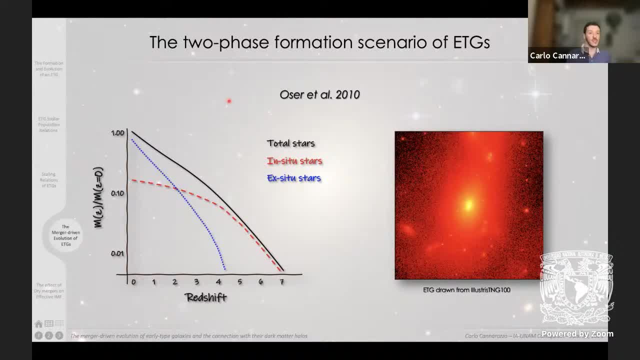 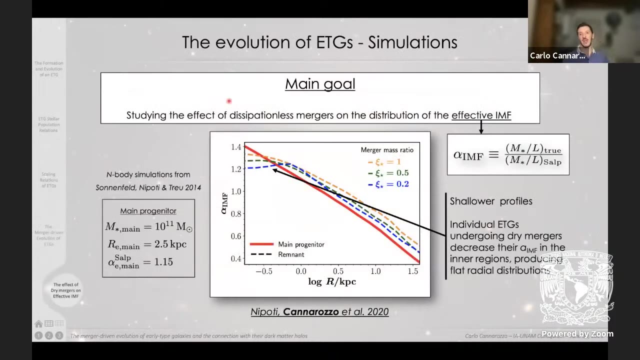 70, 80, 90 percent in some cases, of the total stellar amount is the exit of stellar component, so the fraction of stars formed in another galaxies and then accreted through mergers and accretion processes onto the main progenitors. and there are many, many, many features that suggest this merger driven evolution. 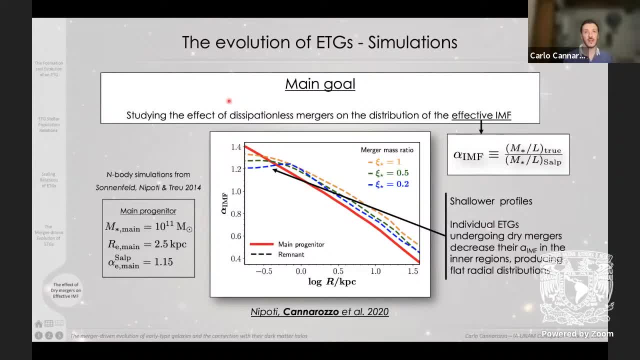 behind early type galaxies, and this is, for instance, one of the study that we conducted in collaboration with carlo nipoti and other co-authors, where we started the effect of dry mergers, both minor and major measure, in binary systems on the radial distribution of the so-called effective initial mass function parameter. 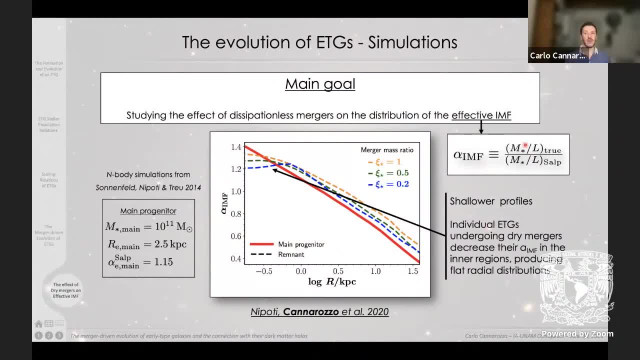 and here, basically, the effective imf is the ratio between the stellar mass to light ratio observed in real galaxies or assigned in to simulated galaxies, relative to the master lighter ratio expected, assuming an initial mass function assumed as a reference, for instance as a bigger one we were. we analyzed the set of these binary, minor and major. 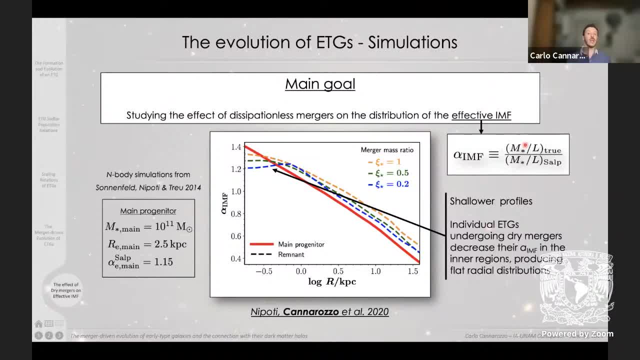 simulations with different orbital parameters and we analyzed the radial distribution of the effective imf, finding that that, with respect to the radial distribution of the main progenitor, here traced by the red curve, the final remnant- regardless of the mass of the two galaxy progenitors and the orbital parameters involved during the merger, 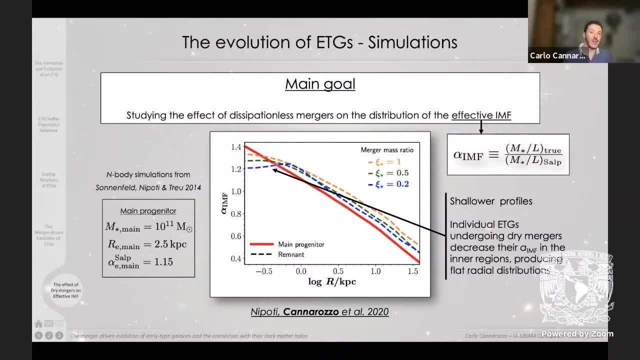 the final galaxy, the galaxy remnant, always show a flattering in the innermost region, and this is a an applicable signature of this merger driven evolution, because it it's telling us that the two stellar components of the two progenitors are well mixed in, even in the innermost regions. 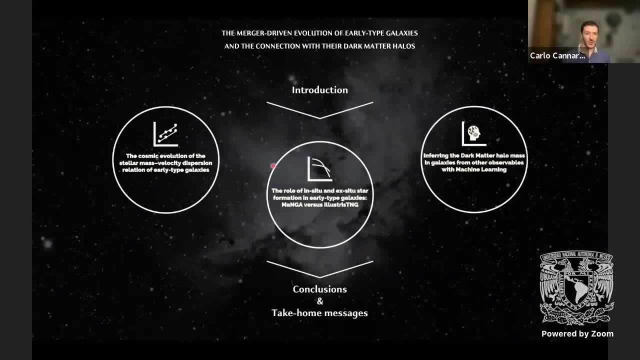 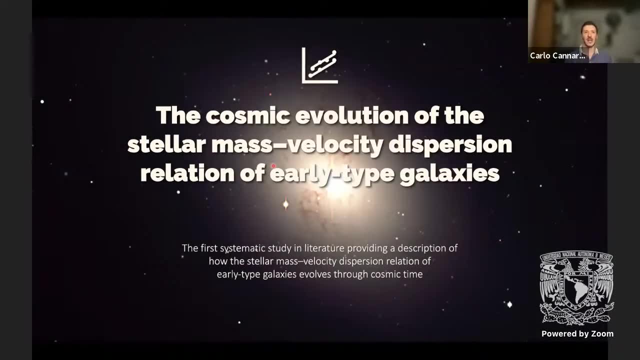 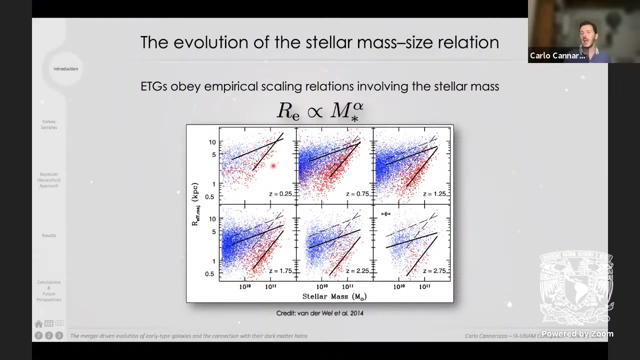 okay, so let's move to the first project of this presentation, that is, about the first systematic study in literature that provides a description and a question for how, on how the stellar mass velocity special relation evolved through cosmic time. um, as i showed you before, um early type galaxies obey scaling relation and with the improvement, 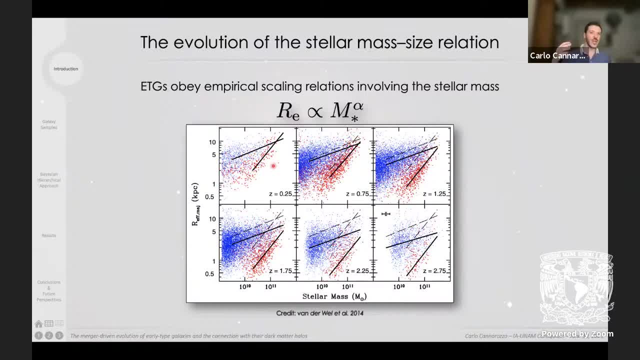 of surveys and telescopes, we are able to observe galaxies deeper and deeper in the universe and we can study if these relations are still there- a tiger redshift or- and if this relation evolve- evolves with the redshift too, and, for instance, this is what was done for the seismus relation. 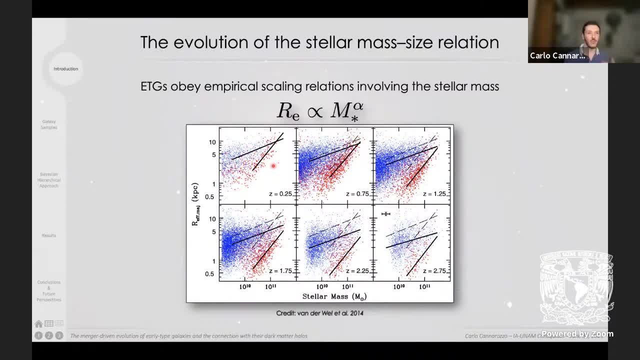 by van der well ethal in 2014 for a sample of both late and early type galaxies. here we have six redshift beings between redshift zero and redshift three, and what is it found? is that, at fixed stellar mass galaxy in the present day universe appear to be 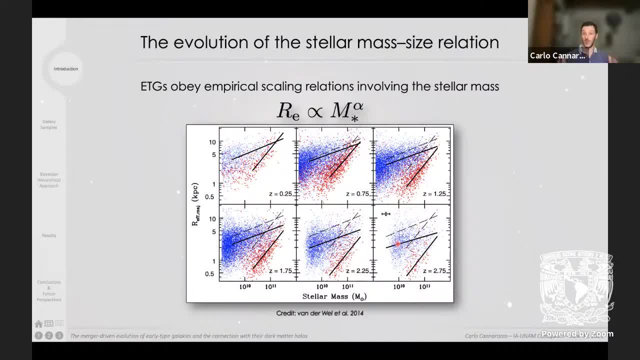 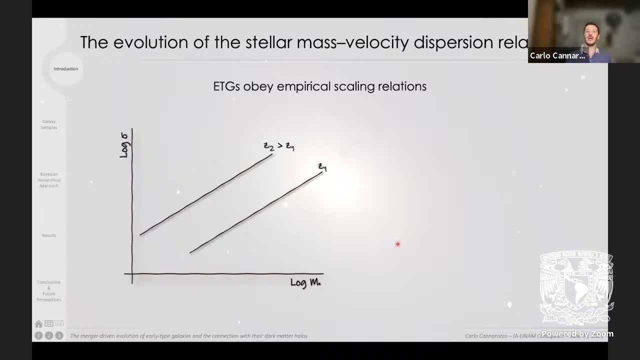 larger tend to be larger than their counterpart with the same mass at tiger redshift. so in principle one can think to study in an analogous way the evolution of the stellar mass velocity dispersion relation, if it evolves. In this sketch I drawn two redshift references of this relation at z2. 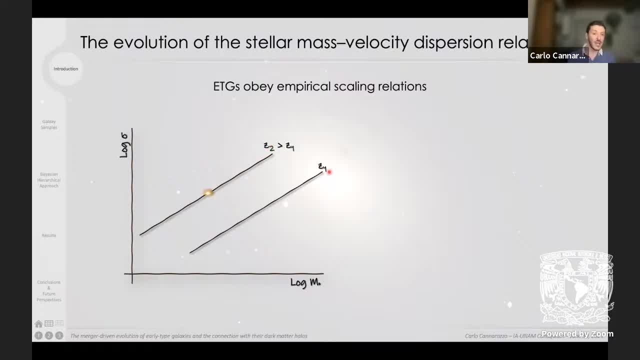 that is a redshift higher than z1.. If I put an early-type galaxy at z2 and I allow it to evolve to reach the functional format z1, this galaxy is supposing that it increases as a function of time. its stellar mass can reach the functional format z1 in three different ways, maybe slightly. 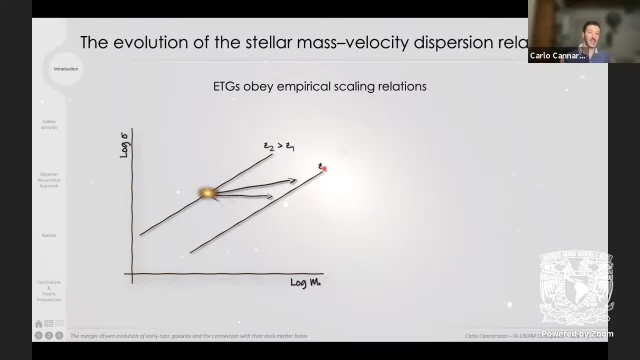 increasing its velocity, dispersion, maintaining more or less the same or decreasing its value. In collaboration with Alessandro Sonnenfeld and Carlo Nipoti, we built a Bayesian hierarchical approach to study how the mass of the stellar mass is distributed between the two galaxies. In collaboration with Alessandro Sonnenfeld and Carlo Nipoti, we built a Bayesian hierarchical approach to study how the mass of the stellar mass is distributed between the two galaxies. In collaboration with Alessandro Sonnenfeld and Carlo Nipoti, we built a Bayesian hierarchical approach to study how the mass of the stellar mass is distributed between the two galaxies. 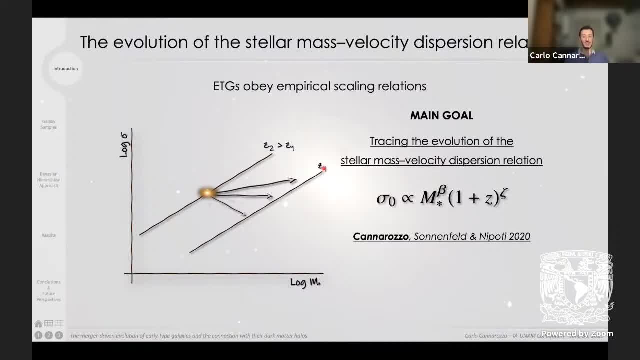 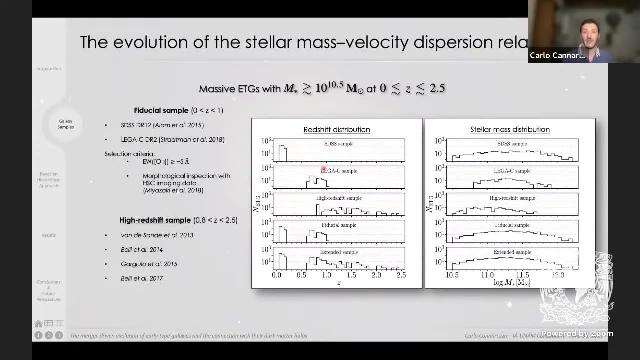 The problem here is that unfortunately unlikely was done for van der Waal-Thal for the side mass relation that evolves through cosmic time. So far there are no available surveys that covers a so huge range and redshift with a reliable and consistent velocity dispersion measurements, And so the first complication of this work was to build our 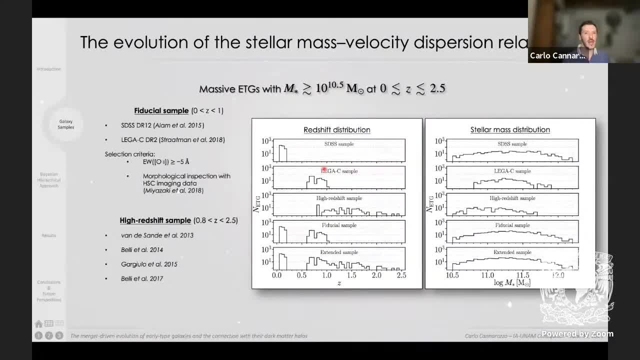 my own sample that is composed by early-type galaxies with a stellar mass greater than 10 to the 10.5 solar masses covering the range between 0 and 2.5.. Here you can see the redshift and the stellar mass distribution of the various subsamples composing my total sample, and there are two main. 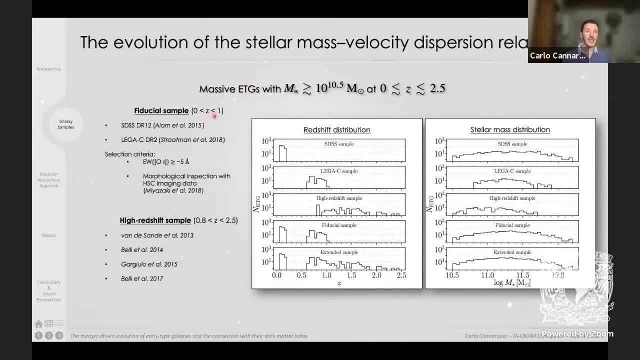 subsamples. The fiducial sample up to redshift 1 consists of SDSS and legacy galaxies that were selected as early-type galaxies, applying a selection on the equivalent width of oxygen second, and then I applied a one-by-one visual inspection, basically to remove all galaxies that 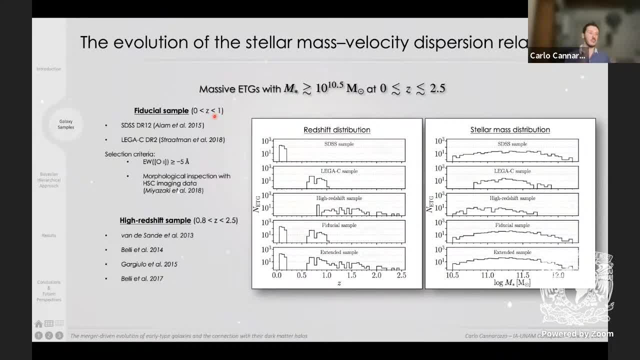 in their images showing weird features merging in axis spiral halves, basically just to keep a sample composed by a roundish or elliptical shape, And then I extended my sample towards either redshift, including looking for other works in literature that defined in a similar way early-type galaxies and the definition of stellar masses. 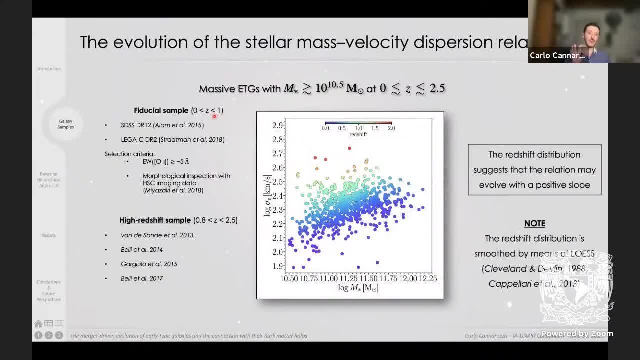 And if I collect all my galaxies and put them on the stellar-mass velocity displacement plane and I color them all as a function of the redshift, what I define is this �distribution� And, as you can see, there is a very clear trend of�there's clear evidence that there is. 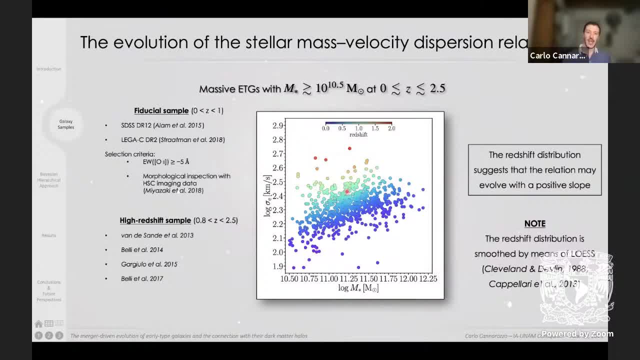 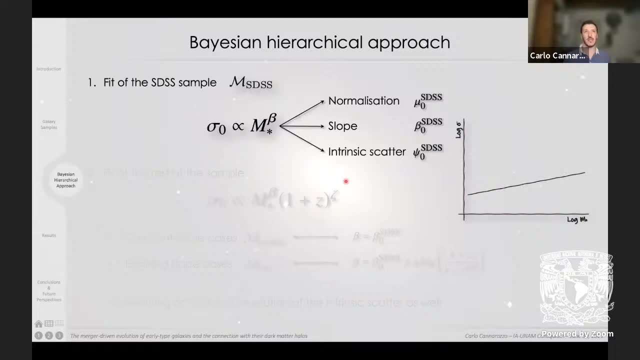 a trend of that. There is a clear evolution, evolution of this relation and in particular, at fixed stellar mass. the higher the red shift, the higher the velocity dispersion. As I've already said, I've modelled this scaling relation employing a Bayesian hierarchical 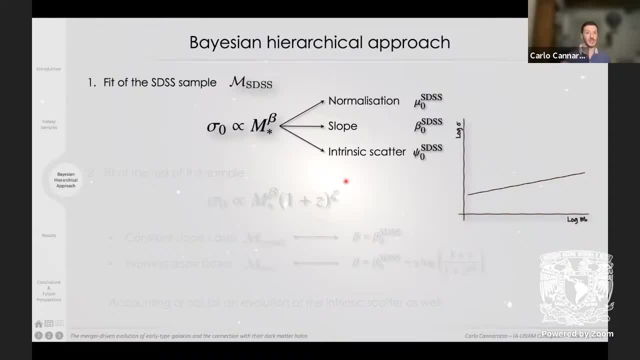 approach that can be easily summarised in two main steps. The first step consists of fitting the galaxy sample in the present-day universe. that, in my case would be the fit of the SDSS galaxies. From this fit we get the normalisation of the relation, the slope, and thanks to the 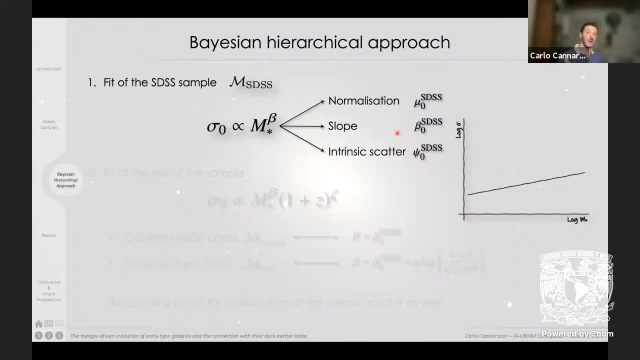 Bayesian hierarchical approach, you are able also to account for the intrinsic scatter that is usually a quantity that is neglected in the fitting literature. And then so we get all these hyperparameters we put in my machine and then I fit the rest of the sample. we assume two different classes of models. 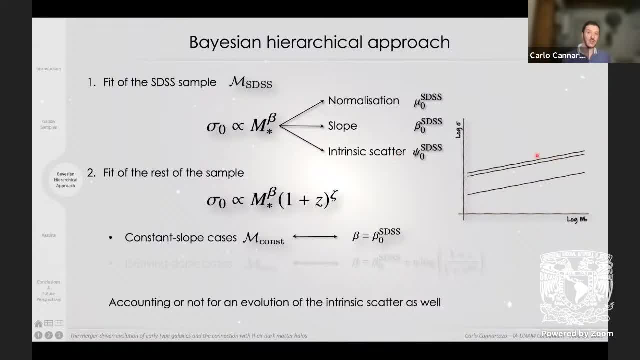 The first class of models is the constant slope model and, as you can see here, it's basically a model for which the relation evolves just in normalisation. The other family of models are the evolving slope models, for which both the normalisation and the slope evolves as a function of time. 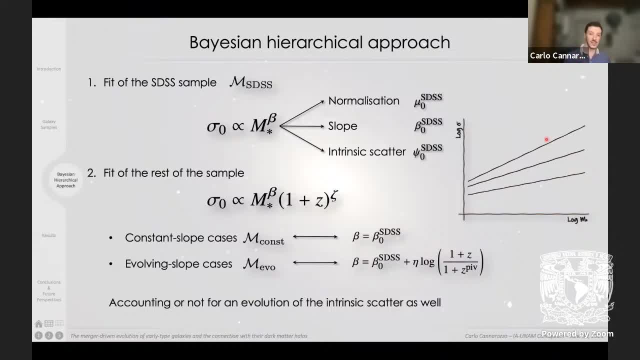 for each model, we consider other two models allowing or not for the evolution of the intrinsic scatter with redshift. So at the end we end up with a plethora of models and according to the analysis of the Bayesian evidence of each model, we do find that the two most representative 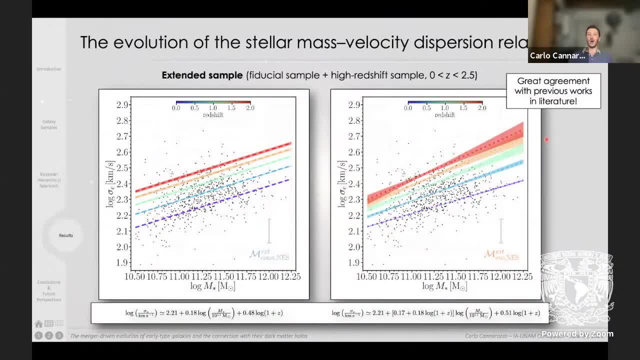 models of the relation are these two: On the left-hand side, you have a constant slope model. on the right-hand side, you have an evolving slope model. For both relations it is found that the intrinsic scatter here indicated by this grey error bar, is found. 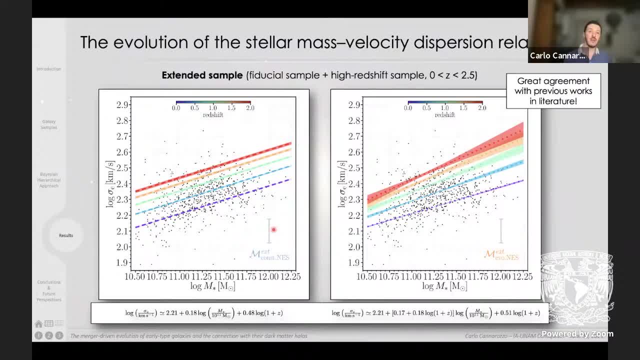 to remain constant at all. redshift. Here I drawn five redshift references between redshift 0 and redshift 2, from violet up to red colors. but let me stress again that with this Bayesian hierarchical approach you are able to tracing continuously over the entire range of stellar mass and over the entire range. 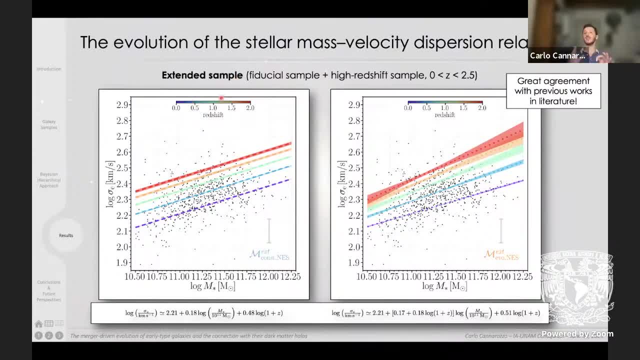 of redshift, this relation. As you can see, there is evidence for the evolution of this relation and to be just to be a bit more quantitative, for instance, a galaxy of 10 to 11 solar masses should be, on average, a velocity dispersion of around 160 kilometers per second. that can. 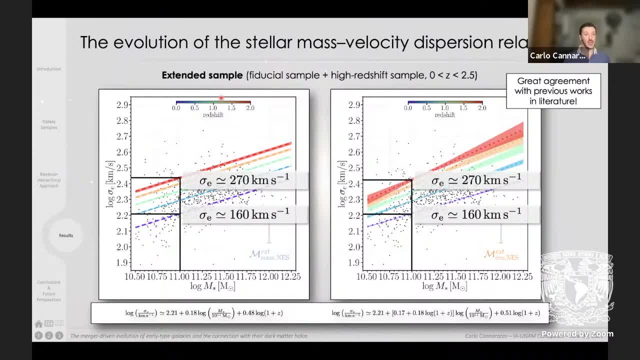 reach even 270 kilometers per second, more or less, at redshift 2.. However, understanding how a progenitor galaxy evolves from higher redshift to reach the functional form at redshift 0 is not trivial at all. But, thanks to our sample of galaxies and our relations found, 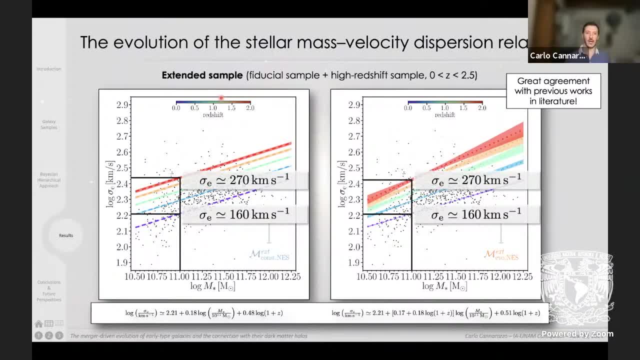 we can identify basically two possible regimes Below 10 to 11.5 solar masses. we can identify two possible regimes Below 10 to 11.5 solar masses. we can identify two possible regimes Below 10 to 11.5 solar masses. we can identify basically two possible. 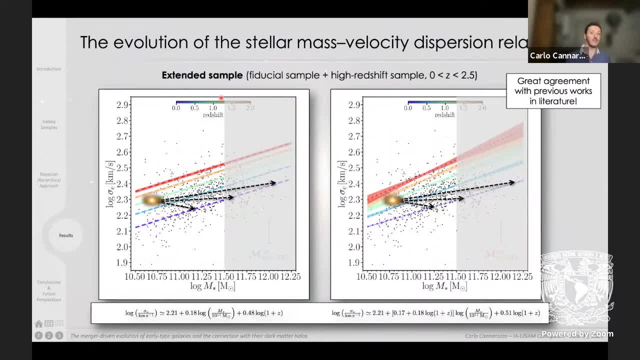 regimes Below 10 to 11.5 solar masses, we can identify basically two possible regimes. If I put a galaxy at redshift 1, it can evolve to reach the functional form at redshift 0 in three different ways: increasing, maintaining or decreasing its velocity dispersion. However, 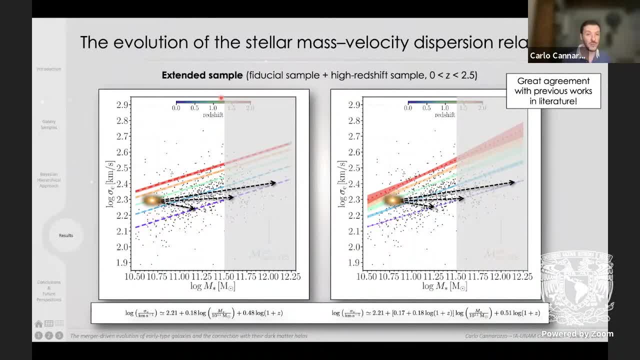 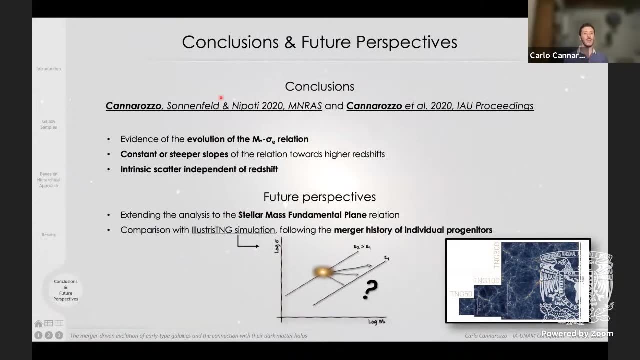 this scenario is not still valid above 10 to 11.5 solar masses, where instead, a galaxy from redshift 1 to reach the functional form at redshift 0 must necessarily decrease its velocity dispersion. So, in conclusion of this first project, I would like to say that we define a clear evidence of the evolution of the stellar. 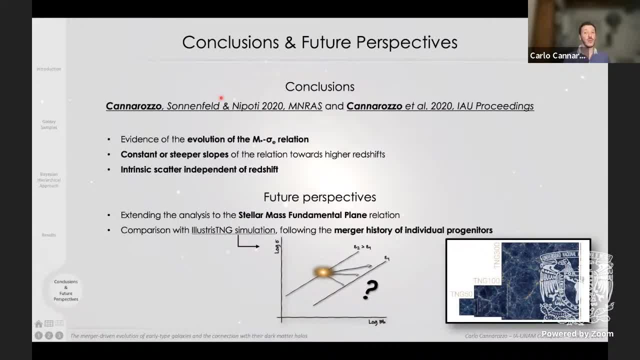 mass with loss of dispersion, relation that I've modeled with a state-of-the-art Bayesian hierarchical approach. This evolution can be with a constant or also an evolving slope, but in any case I define that the intrinsic scatter is found to be independent of redshift. What would be the 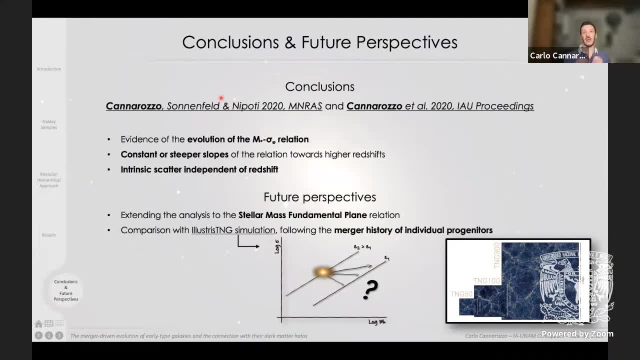 next of this kind of study. For instance, I can apply my Bayesian hierarchical approach for conducting the analysis of the evolution of other scaling relations, like the stellar mass fundamental plane, and to have a more complete 360-degree view of how an individual progenitor 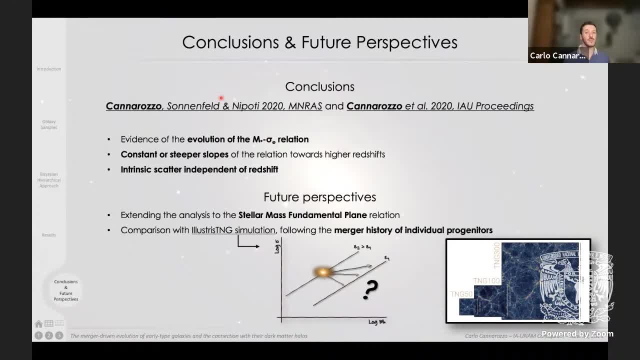 evolves through cosmic time over the stellar mass, with loss of dispersion plane. I plan to make a comparison between cosmological simulation, like illustrious TNG, in order to reconstruct, for individual galaxies, individual progenitors, the evolutionary path and the evolution of the stellar mass fundamental plane. 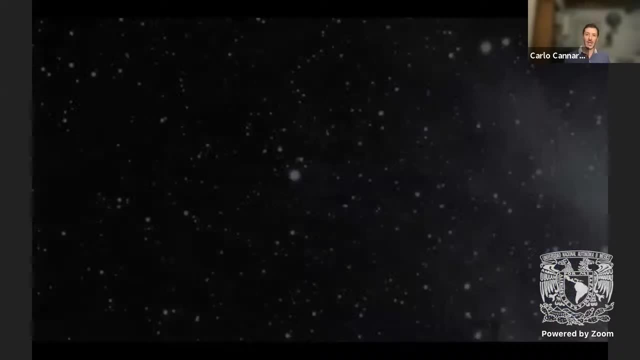 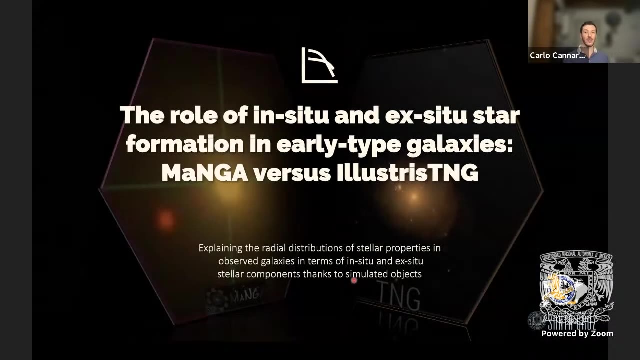 So I concluded with the first project and I moved to the second one, that is, in collaboration with Alexey Lyotho and the group of Santa Cruz, whose aim is to provide an interpretative scenario on how the present-day galaxies that we observe in the universe assembled during their secular 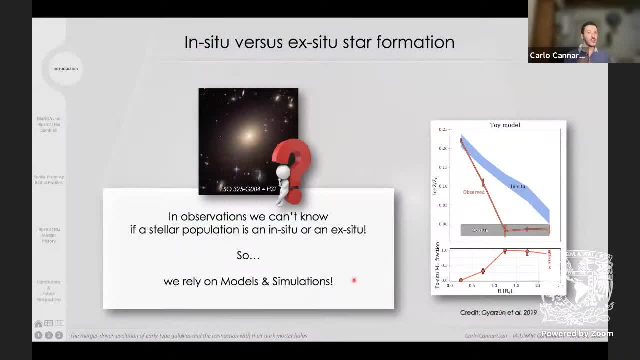 history. The main problem when we observe a galaxy is that if we observe these galaxies and observe a given star inside or a given stellar population, I cannot directly say if that star or that stellar population was born in that galaxy or was accreted from other galaxies, And so you have to necessarily look to dynamical 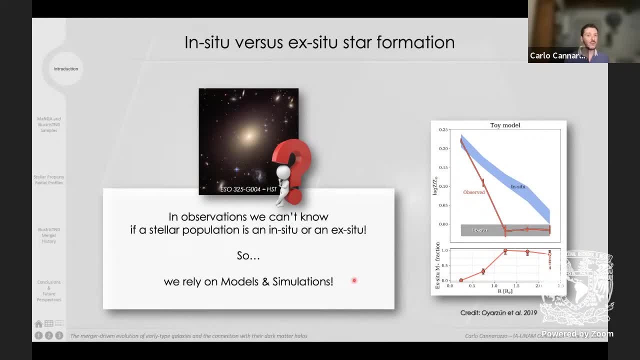 quantities or to quantities derived, for instance, from the spectrum, And you can build a model like the one adopted by Yartsun et al in 2019, where the authors studied, for a sample of early-type galaxies in the Manga survey, the distribution of the stellar metallicity. 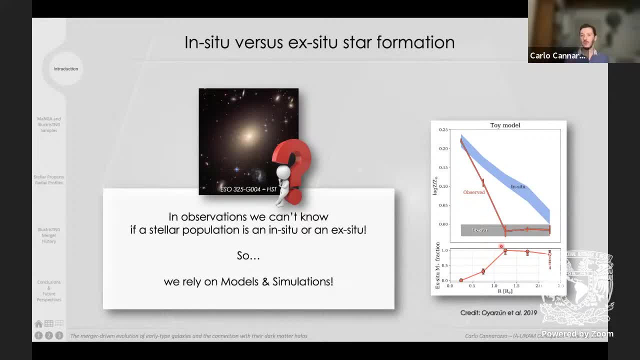 And they defined that the high mass tail of this early-type galaxy sample shows a flattening in the outermost region And they built an ad-hoc model for explaining this flattening. And their explanation is due to the fact that the exito-stellar component from other galaxies 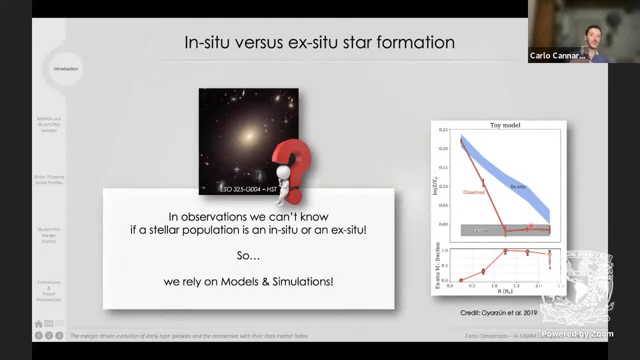 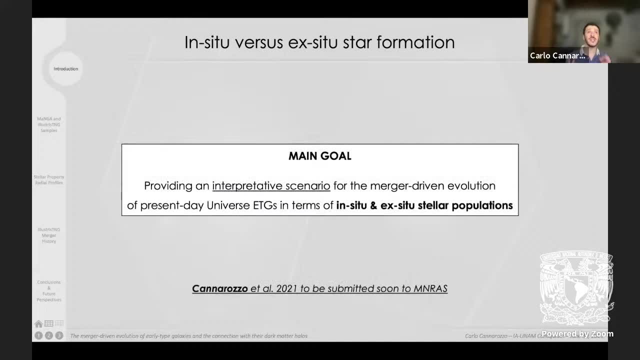 is accreted and remains in the outermost region of the systems. Another possible way to understand if a stellar population was born in cito-exito or provide a scenario is the one that I adopted in this work that I'm going to submit very soon to monthly. 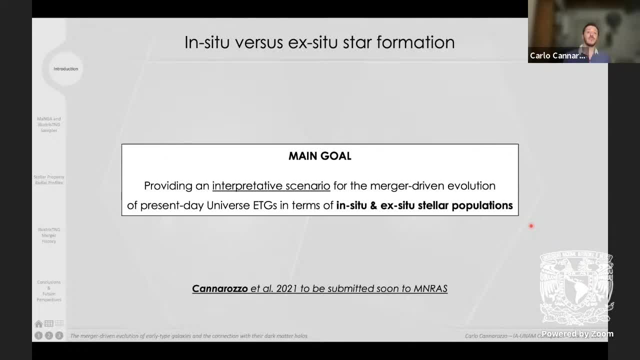 journal, the Royal Astronomical Society's journal, whose aim is to provide an interpretative scenario about the merger-driven evolution of present-day early-type galaxies in terms of in-situ and exito-stellar components. To do that, as I've already said, I make use of Manga and TNG. 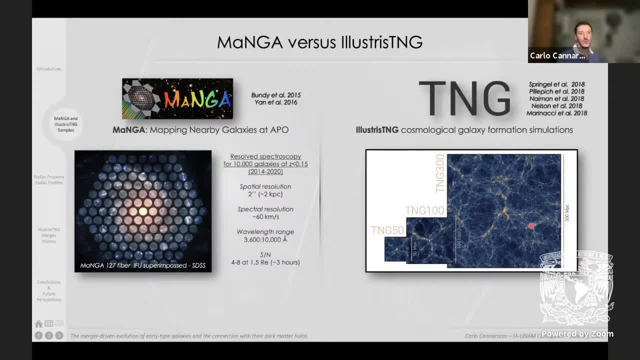 Of course, why them? I have not to tell you what Manga is, since you are largely involved in this survey, But basically, Manga up to now is the largest survey in the present-day universe that mapped more than 10,000 galaxies that exploit the integral. 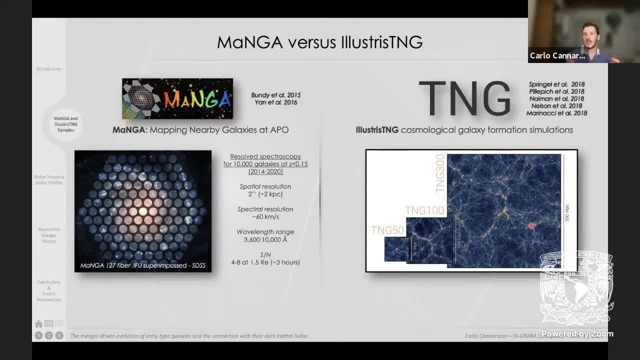 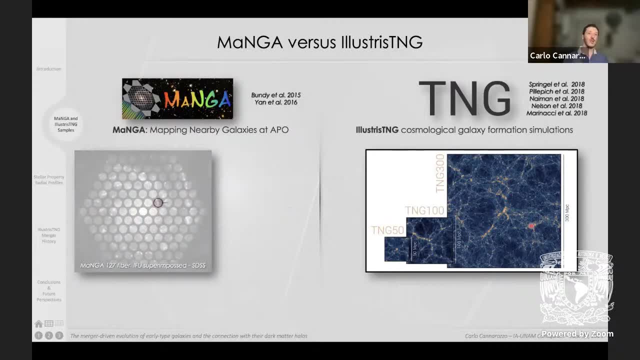 field spectroscopy technique. What does it mean? It basically means that when you observe a given object, you are able to appear to spatially resolve individual regions inside this galaxy and for each region you are able to get a result. So for each region you are able to get. 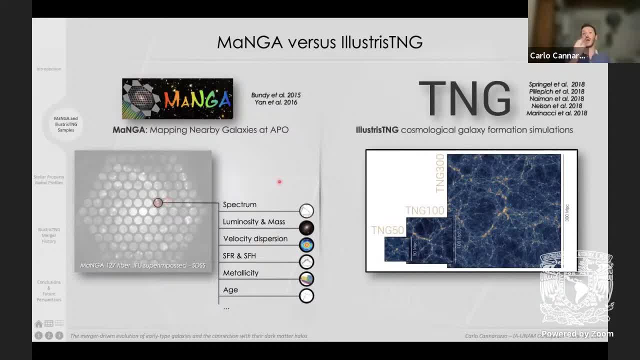 all the information you need. Why TNG? TNG is the next generation of the original, illustrious simulation suite. It is a magneto-dynamical cosmological simulation that mines the galaxy formation evolution in a cosmological context. This suite consists of three different simulation volumes and for this comparison I make use of the illustrious TNG-100. 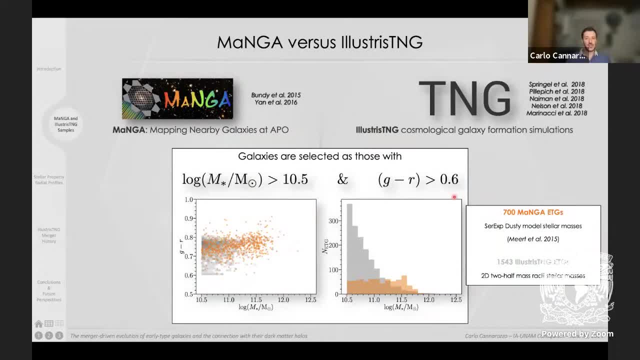 The next generation of the original, illustrious simulation suite consists of three different. there is a simulation volumes and for this comparison I make use of the illustrious TNG-100. our sample of ETGs. applying these two sample criteria, We select all objects with a stellar. 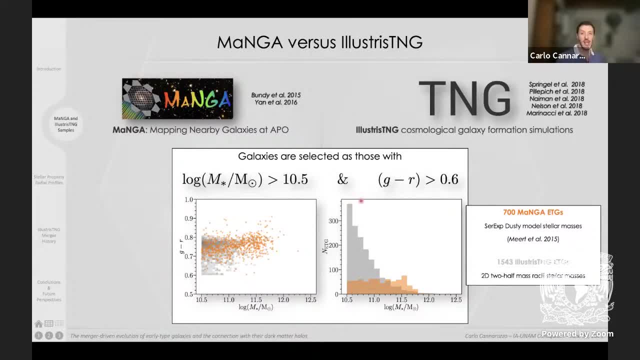 mass greater than 10 to the 10.5 solar masses, and we select only those objects with colors g minus r greater than 0.6.. Here on the bottom left panel there is the a color mass diagram reporting both the manga galaxies indicated by the orange dots and the 2d gray histogram on the background. 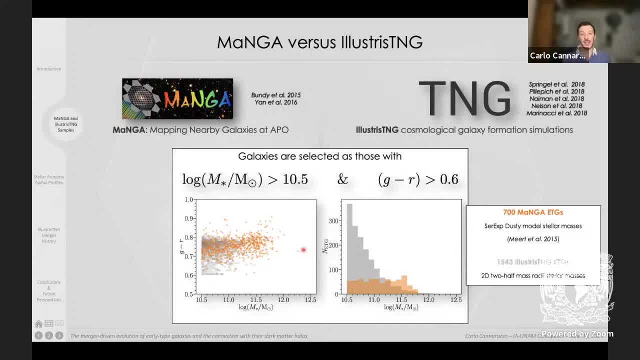 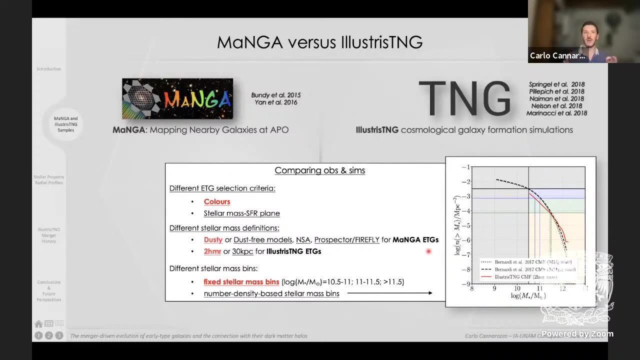 tracing the illustrious TNG sample, While on the right hand side you have the 1d distribution for both manga and TNG, of the stellar masses. I have not much time to go into the detail of this kind of analysis, but the problem is that 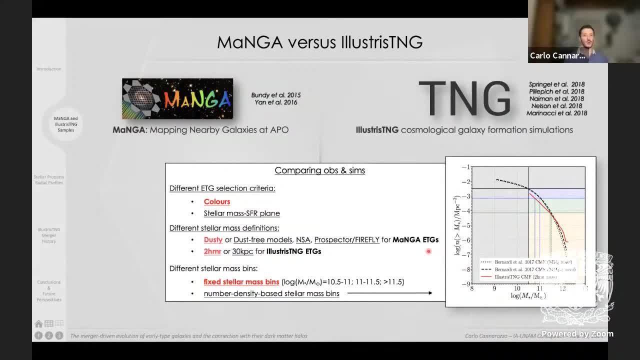 when you compare observation and simulation, it's not trivial at all, and so to understand if the results that I'm going to show you in the next slides are in some way biased by our selection, we tested and our assumption. we tested different definitions of early-type galaxies. we tested different stellar masses for both Manga and TNG galaxies. 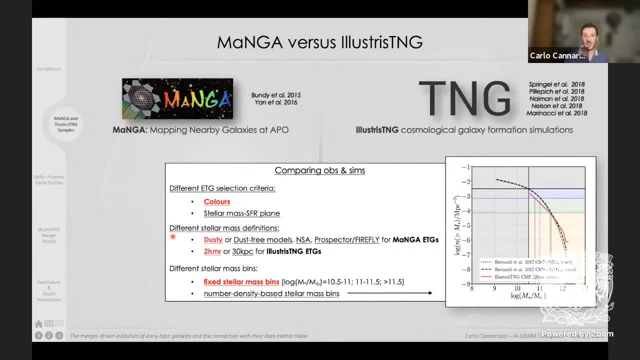 and we tested also different stellar mass beings built, assuming different approaches, And let me say that, however, in any case, we do not find any significant difference, assuming all the combinations of these definitions. So in the following I'll show you the results for early-type galaxies, selected in colors: 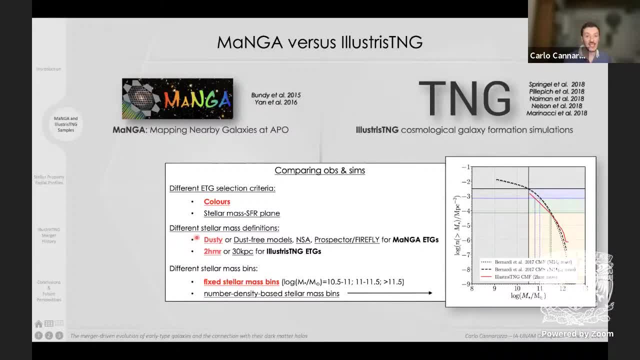 as I showed you before, assuming for Manga galaxies the dusty mass from Mertetal 2015,. while for TNG galaxies, I show you the mass. I use the mass enclosed in a circle with an area enclosed within two-half-mass radii. 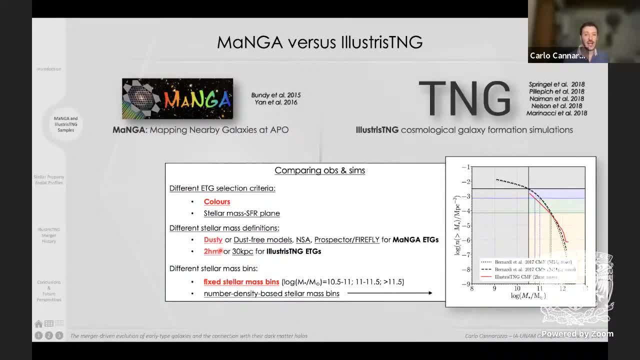 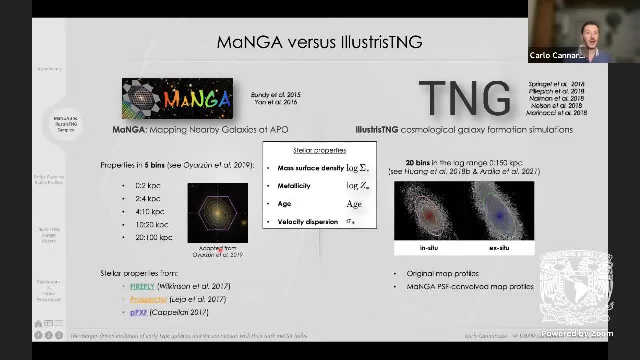 And I compared the radial profile of the physical properties analyzed at fixed stellar mass beings. The four stellar properties analyzed here are the following: the stellar mass surface density. the stellar metallicity, age and velocity, dispersion. Concerning Manga, we derived these four properties in these five beings listed here. 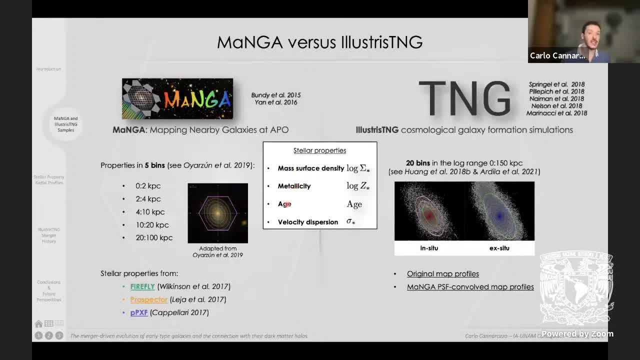 and in particular for mass surface density, metallicity and age. we made use of the estimates made using Firefly and Prospector stellar fitting codes, While concerning velocity dispersion, we use the PPXF estimate. We drawn from the simulation the same stellar properties, but in simulation we are able to. 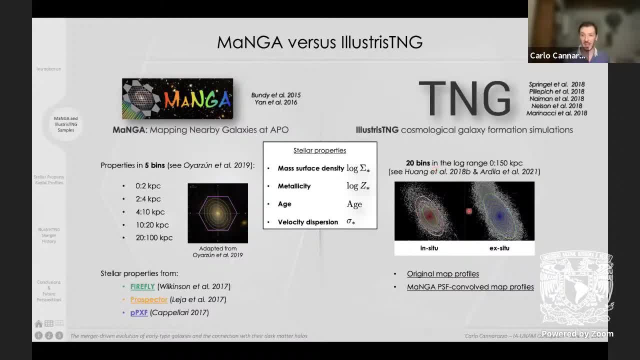 disentangle the role of the in-situ and ex-situ stellar components, as you can see here, And for each of the two stellar components we compute two kinds of profiles. The profiles radically derived from the 2D projected map of the original maps. 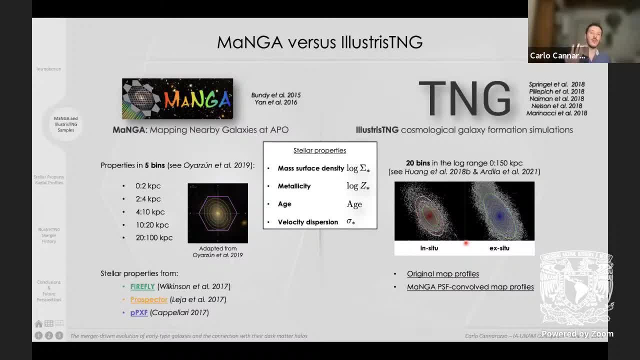 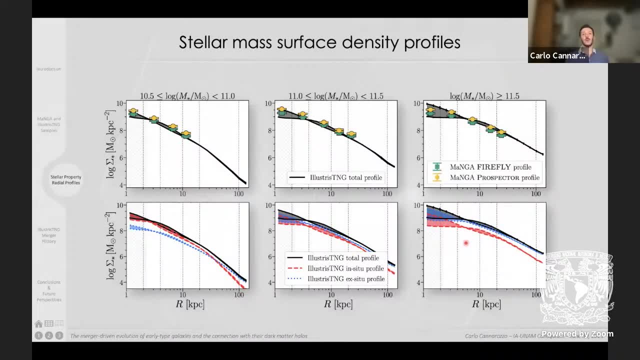 and the profiles from the 2D projected maps that previously were convolved before the Manga PSF. And so start with the results. These are how the stellar mass surface density profile appears. Let me explain and show you these results. Here we have three stellar mass beings. 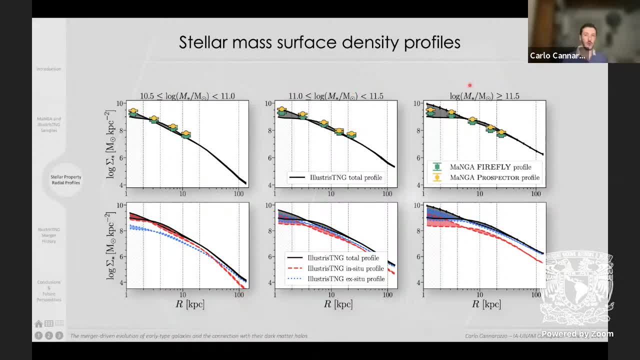 10.5,, 11,, 11,, 11.5, and 8.6.. AD or L You can get some fantastical test results. and above 10 to the 11.5, the bottom panel show you the direct comparison between the total stellar. 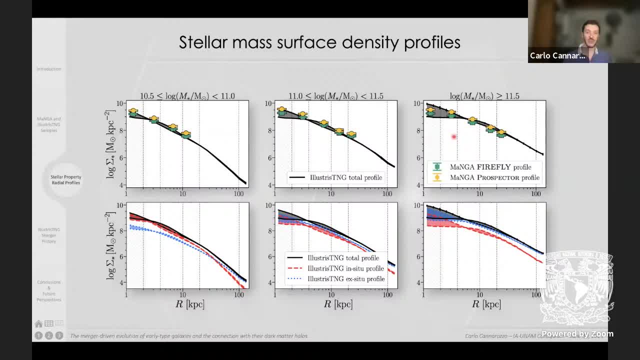 population in king and the manga estimates for the given stellar property analyzed, while below regard only illustrious dng galaxies where ids entangled the role of the institute and exitus as a component. let's focus on the three upper panels, as you can see the illustrious dng profiles remarkably, where we produce the radial distribution of the two. 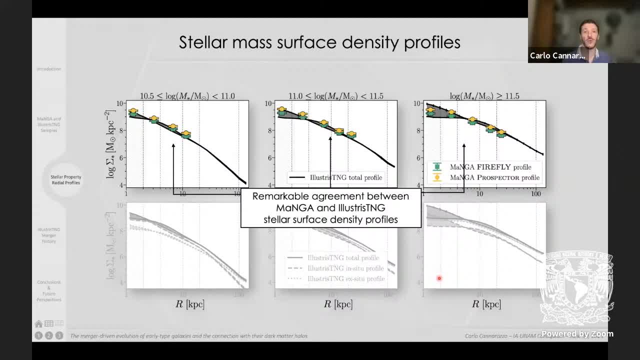 of both firefly and prospector estimates for manga galaxies at all radii and at all stellar mass beings, and this is a very good thing because in this sense we can exploit, as we will see later, illustrious dng for providing an interpretative scenario of how this kind of 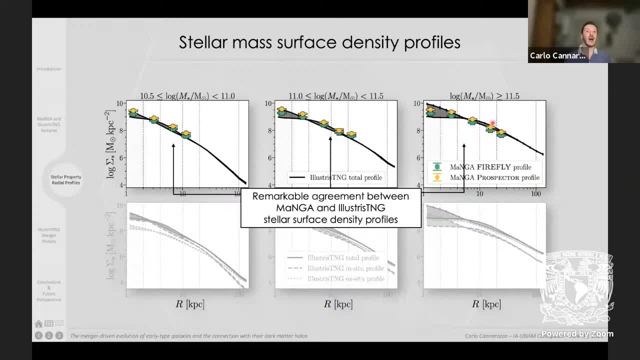 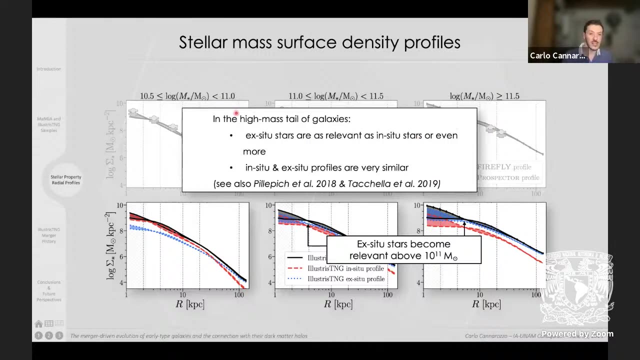 galaxies in the real universe are assembled in the real universe, so this process will affect the uh neural networks and we will see how they are. that is exactly what we are looking at now. so here you can see a construction here and the main number of classes are actually different. 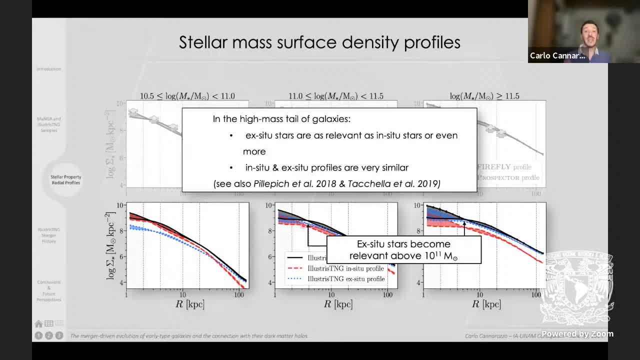 blue dotted curves becomes as relevant as the in-situ component, or even more relevant than the in-situ component in the very massive systems. And this fact and the fact that the shape of the profiles above 10 to the 11 solar masses, for both in-situ and ex-situ stellar, 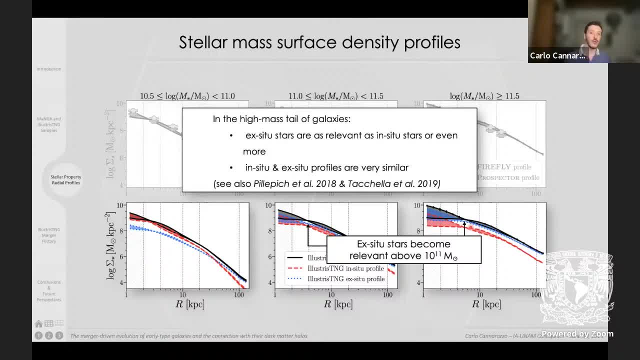 components are very similar to each other are two particular signatures of a stellar mass assembly history that should be marked by major mergers, but we will come on these later. Let's analyze other physical properties. These are, for instance, the stellar metallicity profiles. 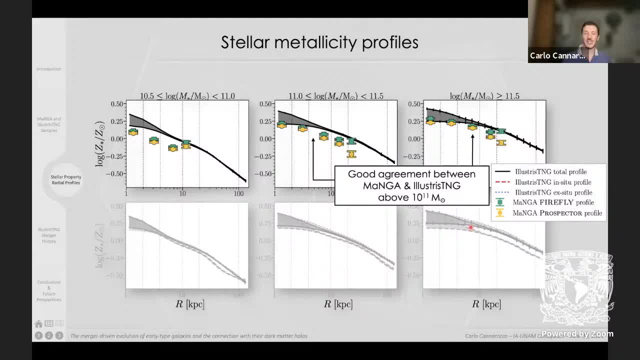 As we can see, more or less, TNG is providing a good representation in terms of the shape, the radial distribution of the Manga galaxies, in particular, above 10 to the 11 solar masses. What about the role of the ex-situ component? 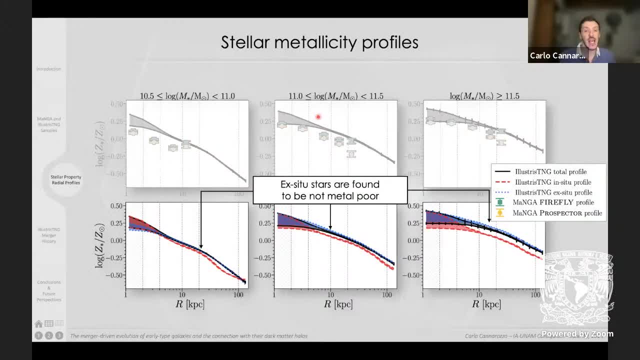 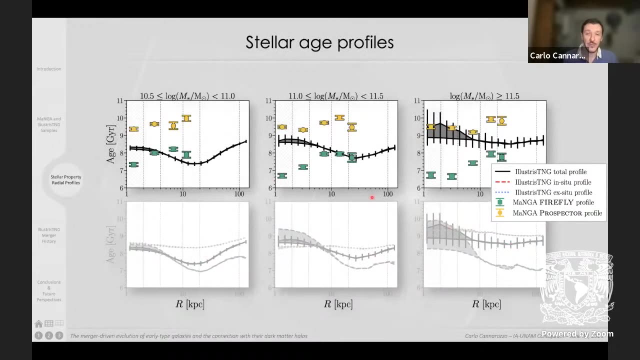 What we do find in TNG is that the ex-situ components tend to be metal rich and, in particular, in the most massive systems, they tend to be systematically more rich than the in-situ counterpart. Let's move on the stellar age and here, as you can see, there is a very clear 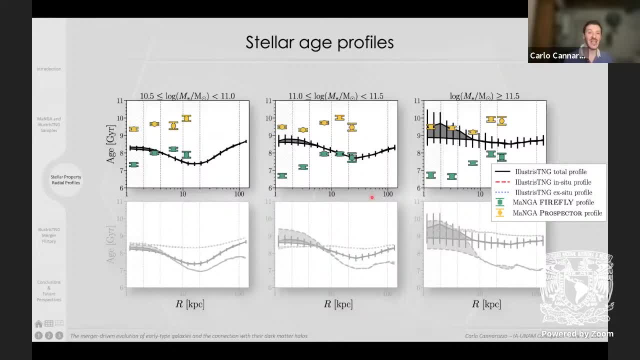 criticism between the two Manga estimates because, as you can see, there is a systematic shift of two, three, even three gigahertz And if we look at the Phylaeas, assigned by Firefly and Prospector to the same galaxies, 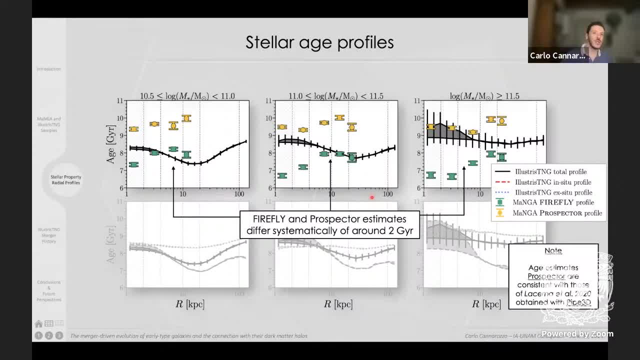 as argued by Conroy in 2013,. for instance, the fact that these two stellar population, these two stellar age estimates differ so much can be addressed to the fact that we are using two stellar fitting codes and these two stellar fitting codes assume different. 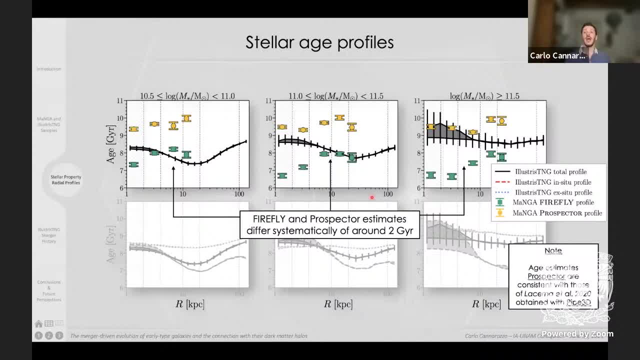 inputs, different libraries, different features of the stellar age, But at least the good thing here is that the almost flat profile of illustrious TNG galaxies more or less always lie in between the two manga estimates. What about the role of the ex situ component in this case? 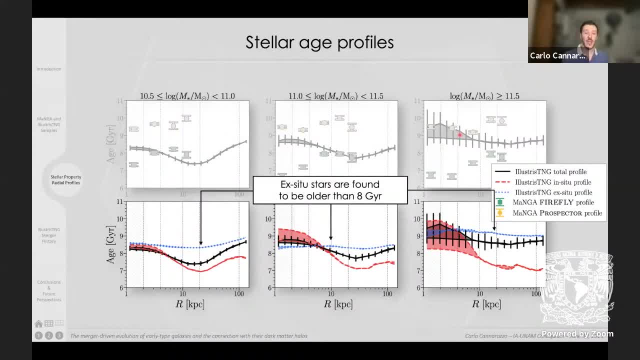 The ex situ component show more or less flat profiles, and these plots are telling us that the ex situ stellar fraction is systematically older than 8 to 8.5 giga years at all masses. But we need more And for instance, we analyze also the role of central and satellite galaxies. 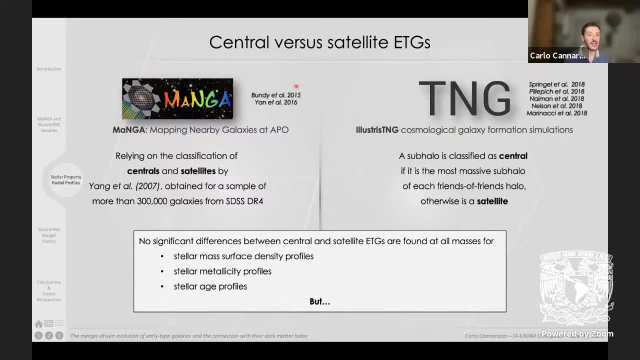 For manga, we disentangle the two stellar population using the Young et al 2007 catalog. here And for TNG, instead, you are able to divide a central and satellite galaxy directly from the simulation. What I find is that there is no a significant difference between central and satellites. 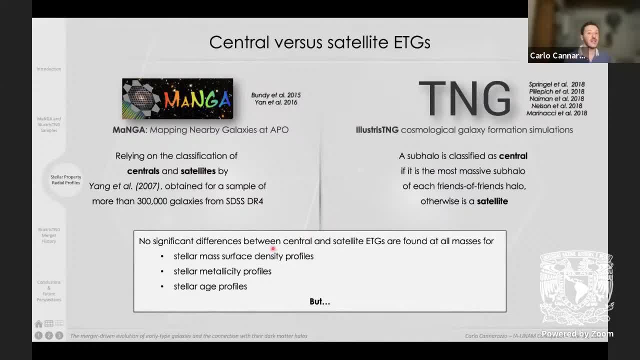 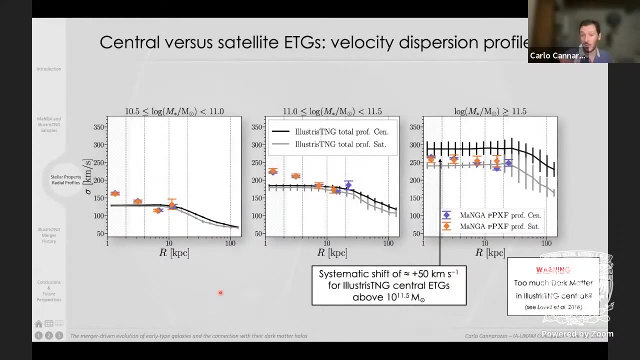 and between the estimates of manga and TNG for the stellar mass surface, density, metallicity and age profiles. But so far I haven't shown you the radial distribution of velocity dispersion yet. And this is how, and this is why I show you now the radial distribution of velocity dispersion. 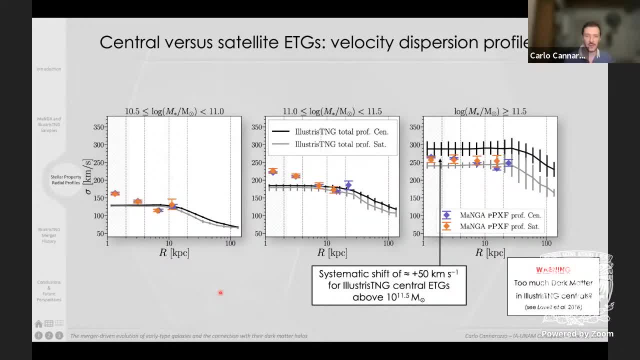 Let me explain, Because this plot is a bit different with respect to the other that I've shown here. Here we have two curves. The black and the grey curves are tracing, respectively, the role of central and satellite galaxies in TNG simulation, while the dots- the violet and orange dots- are tracing the 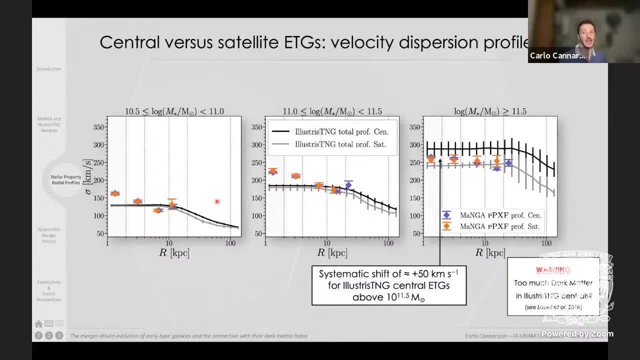 median profile for central and satellite galaxies in the manga sample respectively. What do we define? We define that, qualitatively speaking, below 10 to the 11.5 solar masses, both the central and satellite median profiles for the simulated galaxies more or less reproduce quite well. 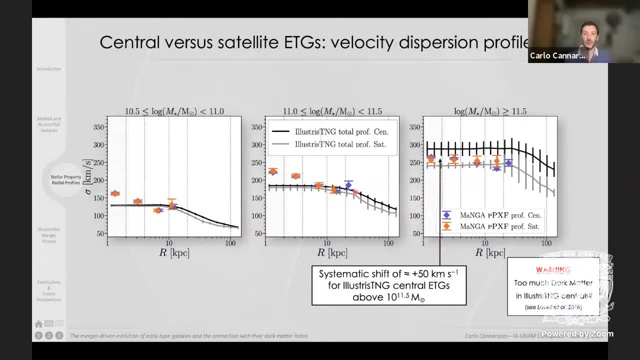 the radial distribution of the velocity dispersion for centrals and satellites in manga, However, it's not still true above 10 to the 11.5 solar masses. As you can see here the radial distribution of the velocity dispersion for the centrals. 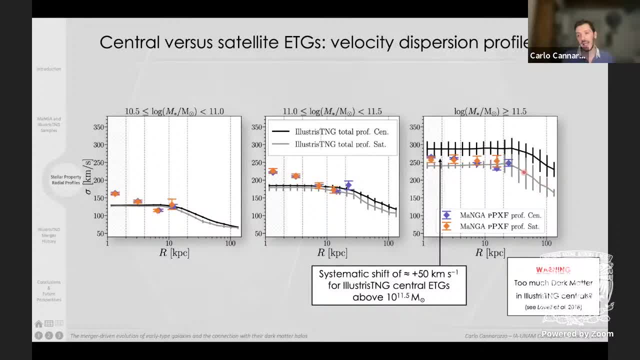 and satellites in manga. However, it's not still true above 10 to the 11.5 solar masses. However, it's not still true above 10 to the 11.5 satellite galaxies, including in the analysis further, indeed, the median profile of satellite in TNG within uncertainty. 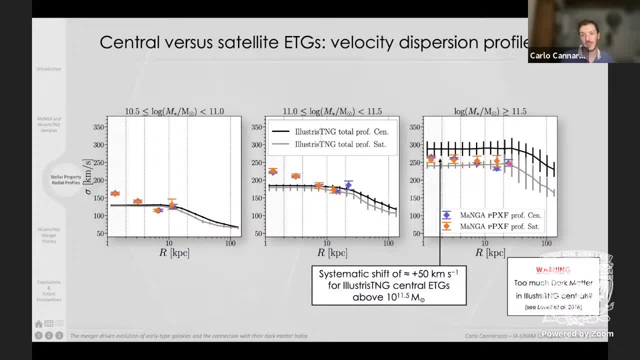 reproduce well the radial distribution of velocity dispersion for both central and satellite, While the profile of central galaxies in TNG is systematically shifted up a factor of around 50 km per second, and the reason for this systematic shift is the following: here 1976, then 1996ね. 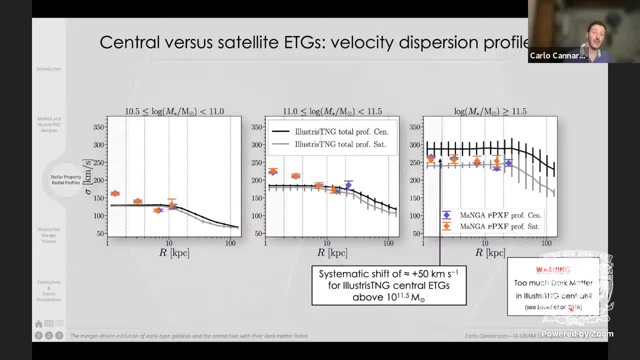 2010. then what argued by Lowell et al in 2018, because central galaxies, in illustrious TNG galaxies, in particular the very most massive galaxies above 10 to the 11.5, for instance, have a too much high content of dark matter and this is the main responsible of this systematic. 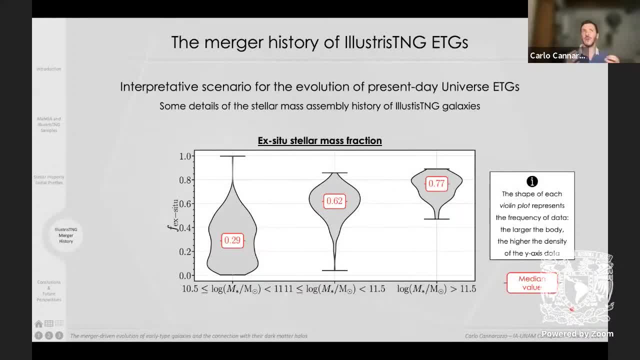 sheet. Overall so far I defined an enough good agreement between TNG and Manga Galaxies and in particular TNG, as I showed you before, reproduces very, very, very well the radial distribution of the stellar mass surface density profiles of Manga Galaxies. So I can exploit. 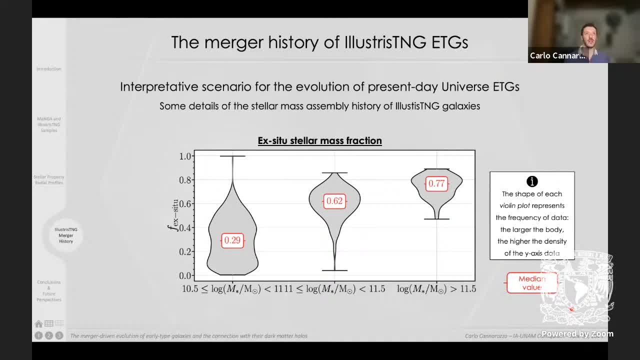 the merger history of illustrious TNG to provide an interpretative scenario of present though universe Httgs and how they assembled Here in these three mass beams, I show you three biolink plots that show the distribution of the fraction of the Xy toe accreted on. 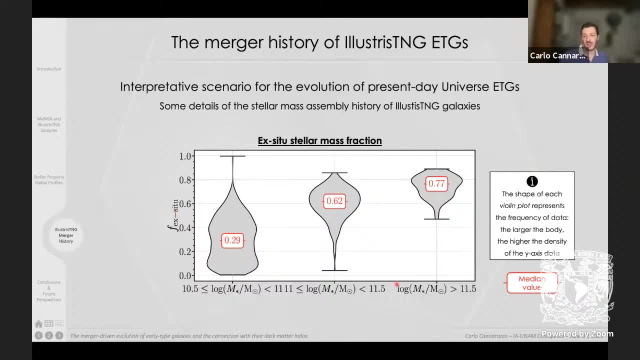 these systems. As you can see, as the mass grows up and goes up, the fraction of the xy toe goes up as well and in particular for the most massive system, on average 80, more or less at description, over 80 per cent ofíssy huge. ET. So I'm now continuing with a just simple new theorem, doing the constant number of Xy to once again extend the relationship between Pantsone andIK- which is all watching here, Pantsone- to why are indicated by theseعتbles Thoris? Well, this is when it was planned before. 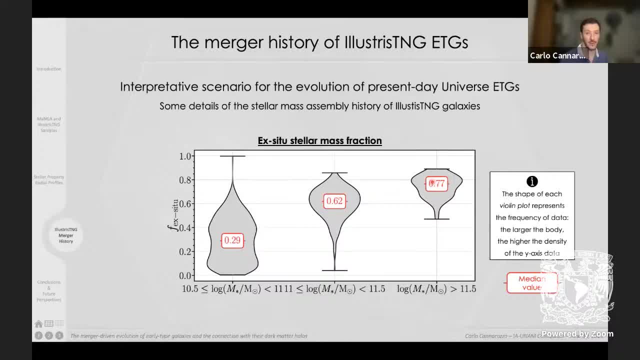 with żad پ wahrσιο, for example, after more or less 80%. we wanted the information of the of the total fraction is due to the Xe2 component, But how this Xe2 component is accreted. if I, for instance, analyze the fraction, 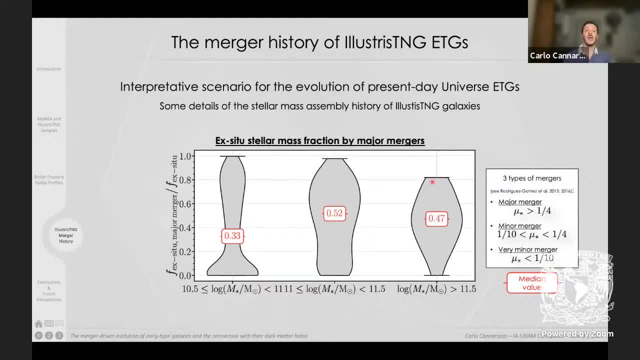 of the Xe2 component, due only to major mergers relative to the fraction of Xe2 component due to all the Xe2 component, although these distribution are very spread over the entire range on the y-axis. what is it found for TNG galaxies is that: 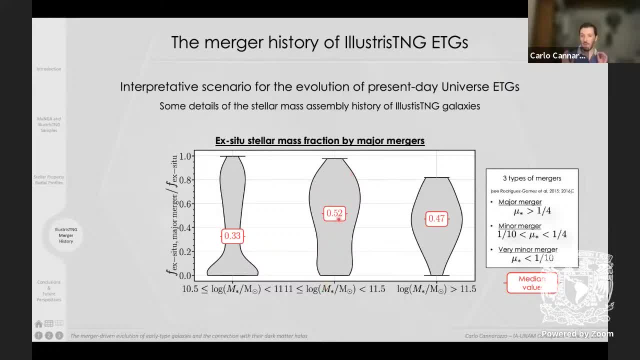 above 10 to the 11 solar masses. on average, half of the total of the Xe2 component come from major mergers And so, given the good agreement between TNG and Manga galaxies, and these last results, a possible interpretative scenario. 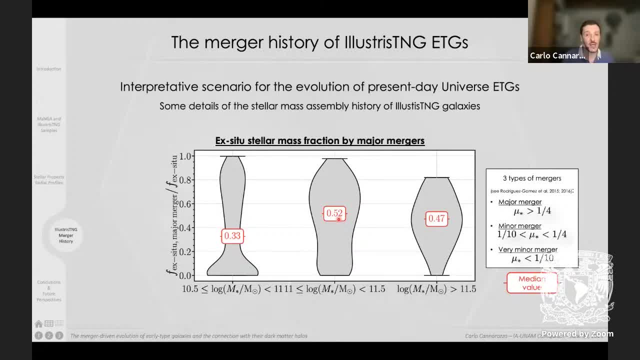 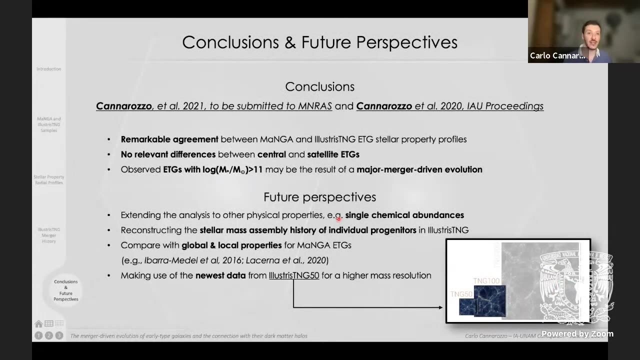 for the present-day universe, early-type galaxies that we observed can be that above 10 to the 11 solar masses, this kind of system may be the results of a major merger-driven evolution. So, in conclusion, I compared the galaxies simulated in TNG and observed in the Manga galaxies. 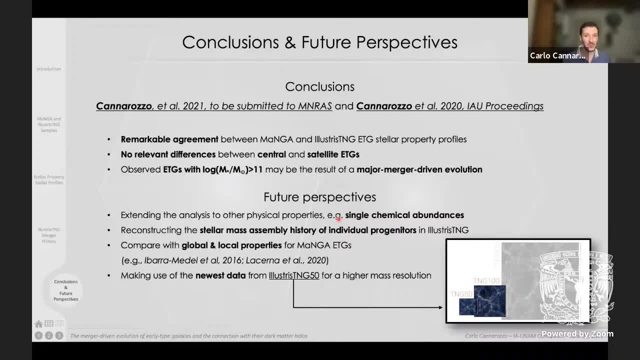 in order to provide a scenario of how these galaxies assembled through cosmic time. We do find that TNG reproduces well some physical stellar properties of galaxies, in particular the stellar mass surface density. There are no relevant differences between centrals and satellites. 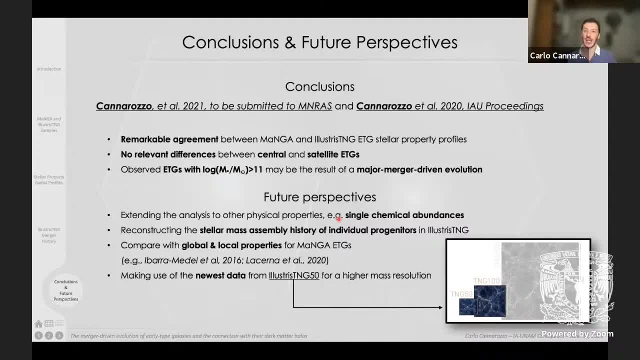 except for the high mass state for velocity expression in TNG galaxies, And so we provided this possible scenario of a major merger-driven evolution for early-type galaxies that we observe in the local universe. This work will be submitted very soon, but what the next of this kind of analysis? 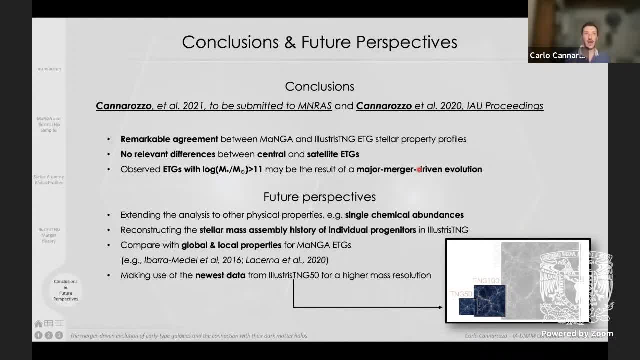 Of course I'm going to extend the analysis, analyzing other aspects, For instance individual chemical abondances in TNG and the Manga galaxies. I'm going to reconstruct in TNG galaxies the stellar mass assembly history of individual progenitor gapiami. 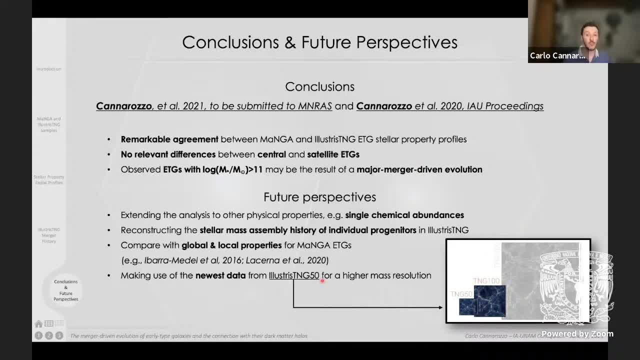 and these can be directly compared with the global and local properties for Manga galaxies. At the beginning showed from La Serre國家 Inter i Total 2020,. I am going to use also the newest data from illustrations in TNG- illustrious TNG-50 simulation that are characterized: 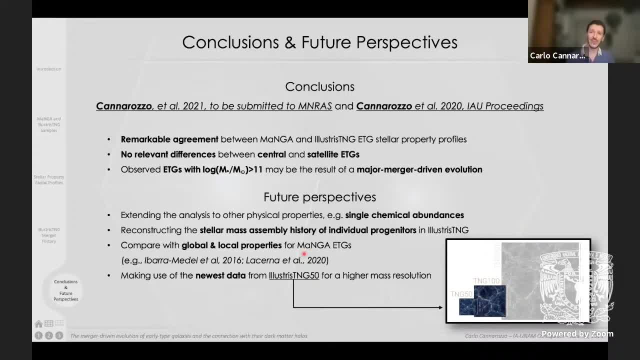 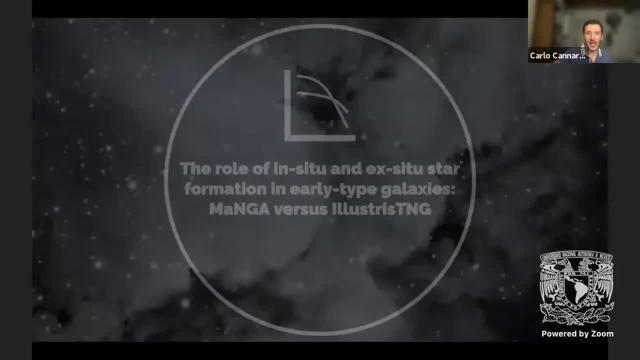 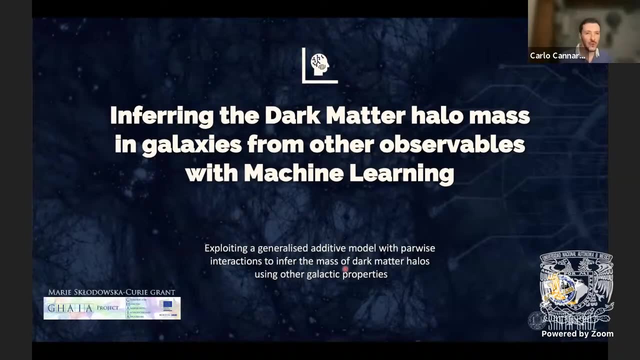 by a higher resolution quality of the data. And then let's switch to the final part of this presentation, Changing a bit the topic. as Aldo said before, in 2019, I was awarded the Marie Curie Grant from the European Commission to conduct a project. 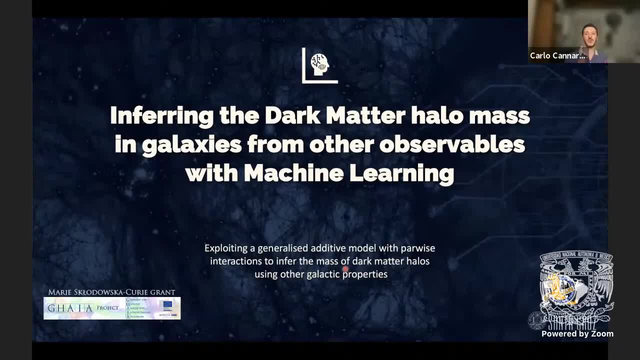 in the context of data analysis and machine learning, And thanks to this grant, I visited for more than six months the University of California, Santa Cruz, working with Alex Liotho and their group, and also collaborating with the Microsoft research teams. 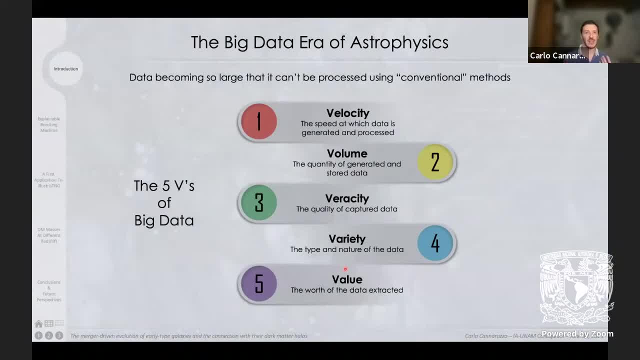 In the last decades, in the last two years, astrophysics has been leading the so-called big data era. Every day, indeed, astrophysicists and cosmologists have to face with an enormous amount of data, of different types of data. 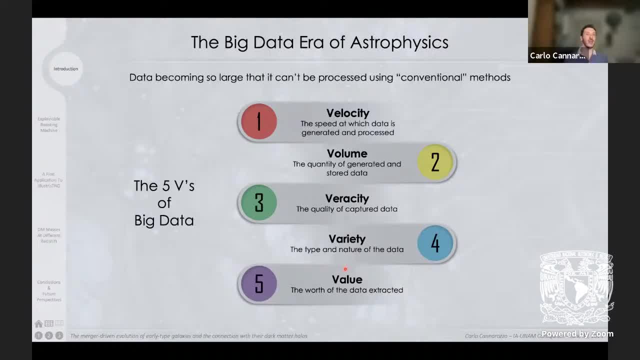 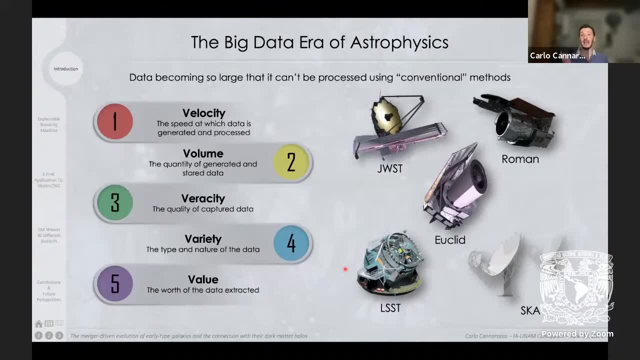 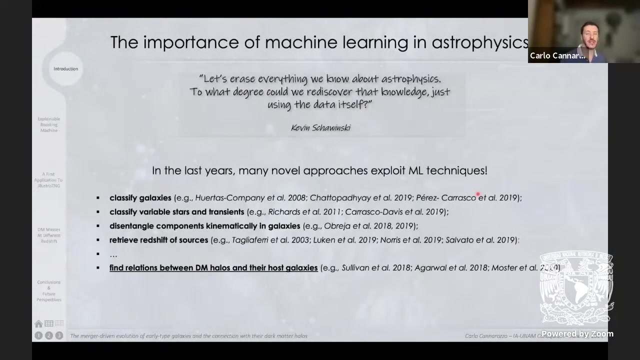 of different nature, coming at a very huge rate, And one, of course, of the main sources of this huge amount of data are the current, the next generation of observation carried out, for instance, from these newest and upcoming telescopes, Machine learning and deep learning techniques. 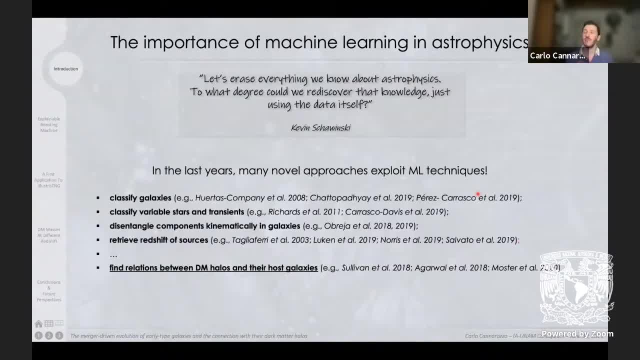 are widely used in machine in astrophysics for a wide variety of problems, For instance for classifying objects like galaxies, stars, transients, exoplanets, for disentangled dynamical aspects in images, for retrieving distances and redshift of sources. 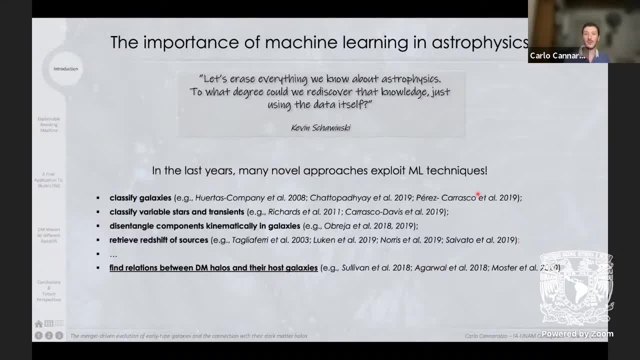 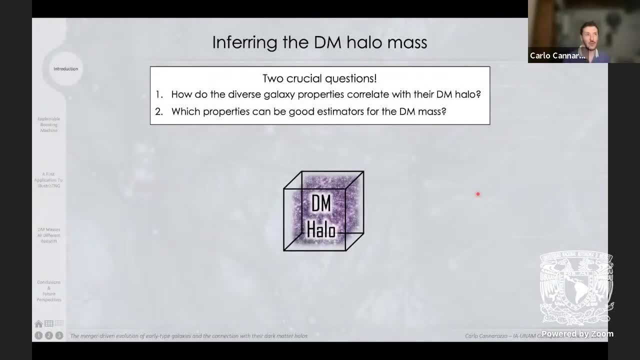 and also to find possible relation between dark matter halos and day-host galaxies. For my scope, that is, to infer the mass of dark matter halo in real-time. I'm going to use this data, But I'm also going to use it to find out. 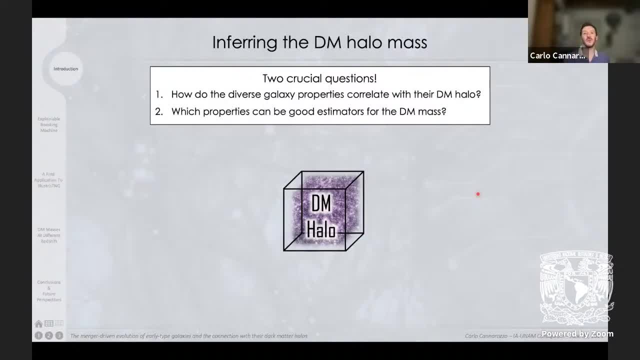 more about the mass of these galaxies. There are two a priori, two crucial questions to do. The first one is how different galaxy physical properties correlate with dark matter halos And, if they correlate how, which of them are good or even the best estimators. 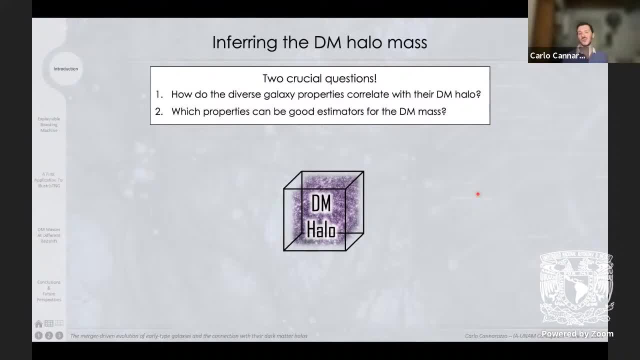 for the mass of these dark matter, halos. Of course, the most well-known study- and largely studied a relation that links the galaxy, the galaxy-based galaxy, with the galaxy-based galaxy, the galaxy to its halo, is the stellar-to-halo mass relation that links directly the stellar mass. 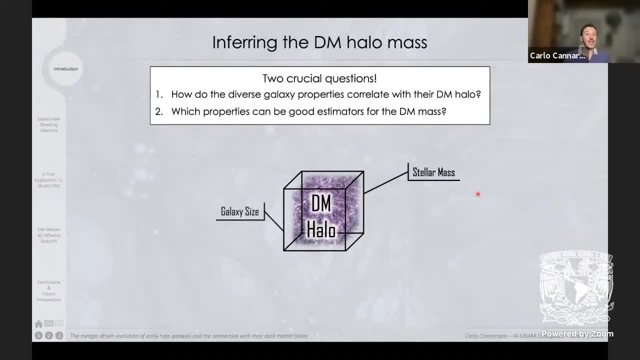 to the dark matter halo mass. Another possible relation is that the galaxy size correlates with the size of the halo where it is hosted. However, in this kind of study one should take into account also for all the other correlations that these properties may have with all the other several. 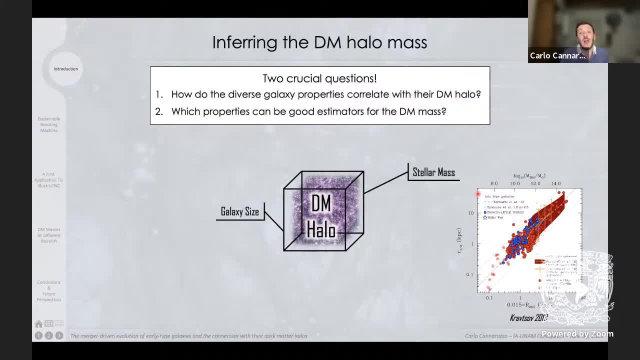 properties, For instance. in fact, we know that the stellar mass is strictly related to the mass of the central supermassive black hole, or, again, as I showed you before, with the stellar metallicity, or it shows a relation also with the gas metallicity. that again in turn, show a 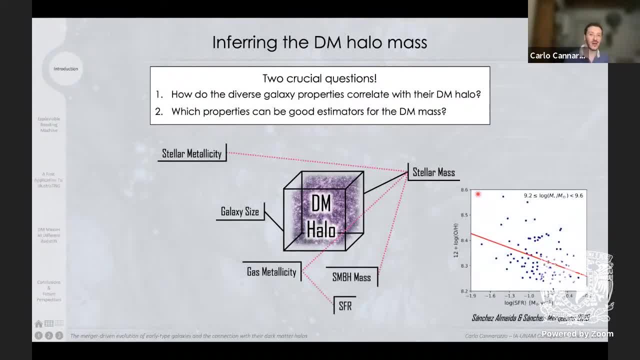 correlation with star formation rate, and it was also found that the ratio between the black hole accretion rate and the star formation rate directly relate with the mass of the star. So at the end of this process we end up with, as you can see, a very intricate and complex. 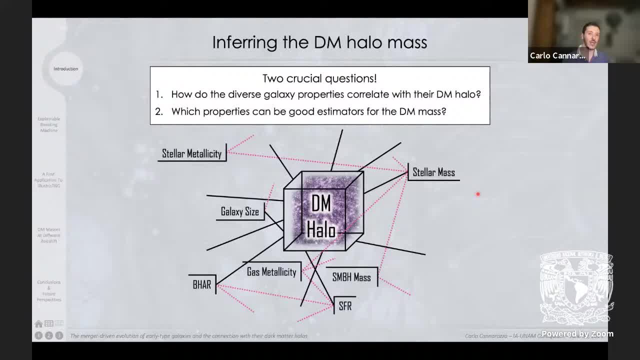 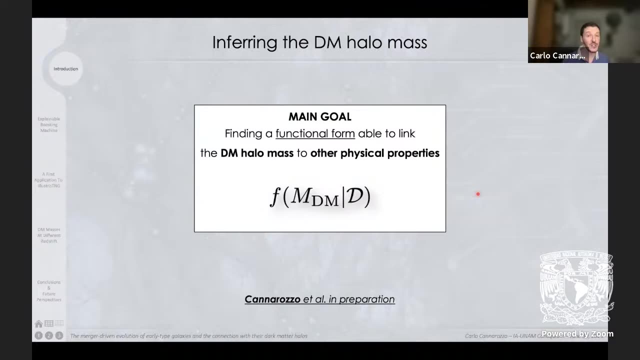 web of possible relation and, of course, machine learning can be a way, can be a silver bullet to shed light on these hidden patterns. The main goal of this project, so, it would be to exploit these machine learning techniques that learn, that are trained, model on the basis of cosmological simulation in order to derive 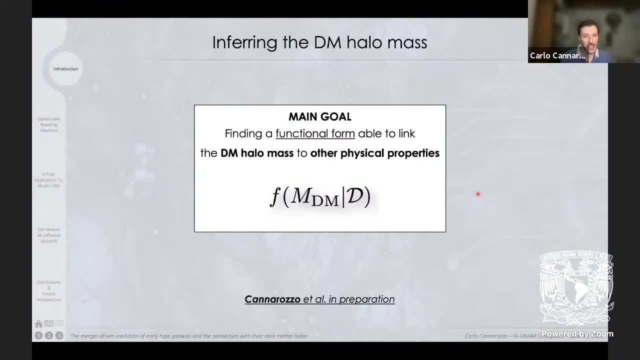 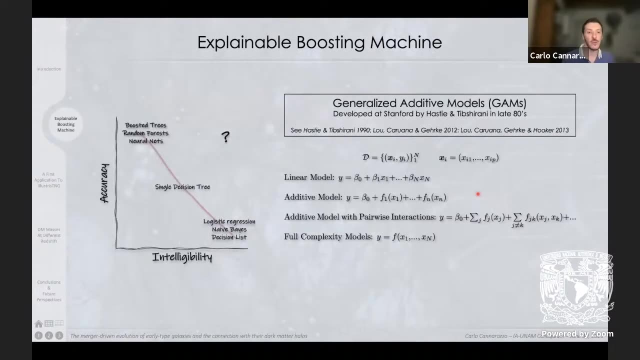 a functional form able to be used on real galaxies for deriving their mass of dark matter halos using the physical properties that you observe in your observation. basically, In machine learning we usually observe a sort of trade-off between two properties: The accuracy and the intelligibility Among the most accurate machine learning techniques. 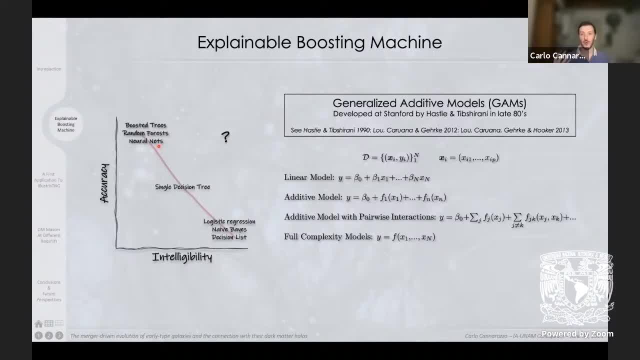 we count, for instance, boosted trees, neural networks, random forests- Much less accurate but very, very, very intelligible, so easily to be understood by the user that is using these methods. we have, for instance, linear or logistic regression. 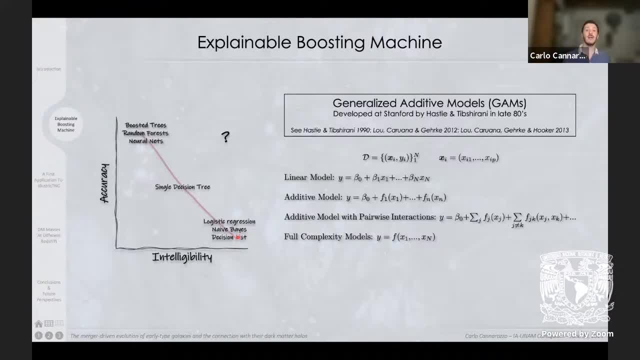 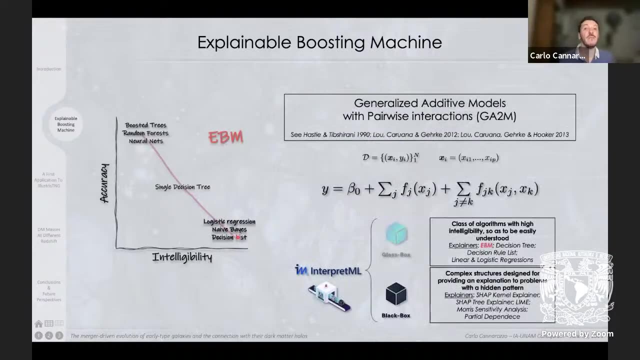 In between these two different classes of models, there is a family of models called generalized additive models. The good thing is that recently Microsoft Research released EBM. EBM- that is the explainable boosting machine- is a state-of-the-art machine learning method that 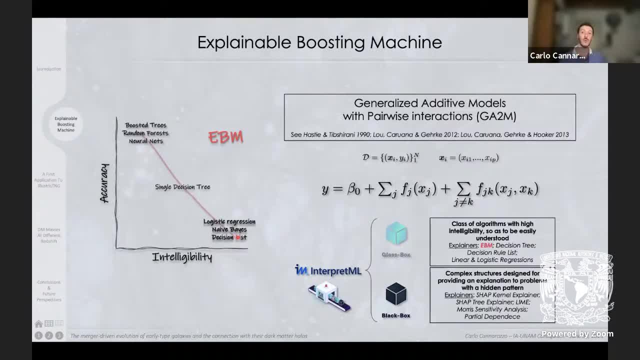 in the context of generalized additive models with pay-wise interaction that is at the same time, is as accurate as intelligible. EBM is fully included into InterpretML. that is a toolkit, a full library of machine learning methods classified on glass box models and black box models. But let's focus on what EBM does. 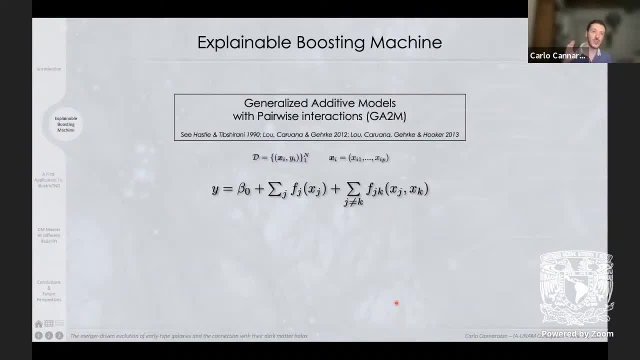 This is a generalized additive model with pay-wise interaction. So if you have your data set of observation, the quantity one would like to infer that in my case would be, for instance, the mass of the center of mass of the point. in the case of the uh point x-axis, you have the error log. 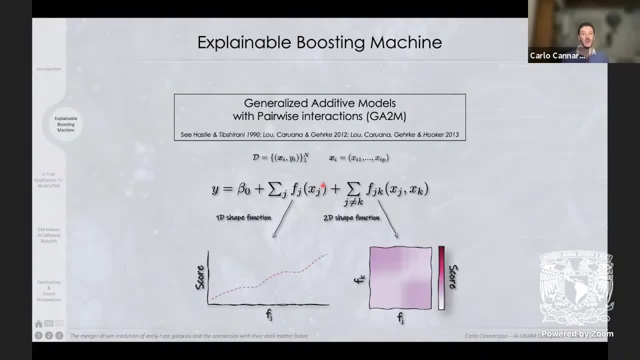 that is the mass of the point in the case of the energy axis and in the case of the temperature, or few of the other possible observations of the point. so that's what the EBM model students say is going to do, and then we would simply interpret the same thing just by using the same algorithm. 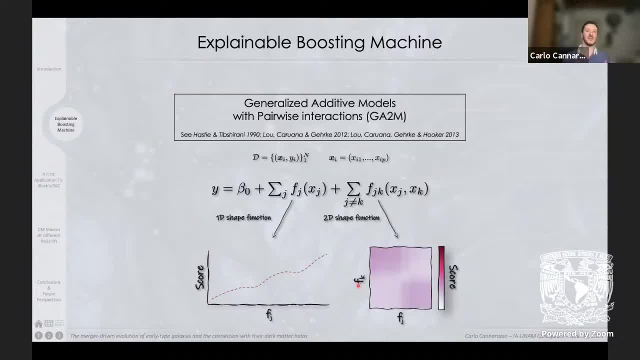 However, the problem here is that the values of the function, the value of the function and the functions of the function themselves, can be expressed as a summation of two classes of map. on the 2d shape function is a quantity in units of the quantity to be inferred, so the mass. 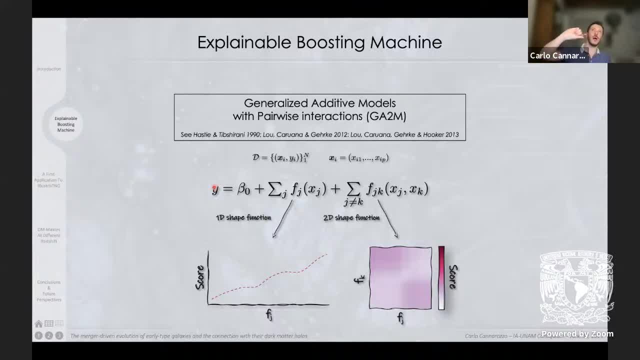 of dark matter that the user had to uh has to add or subtract to make the final inference. but i will show you a sample, an example, very soon. ebm is largely used in many different science fields. the first application was presented in carolina 2015 from the microsoft research team uh to 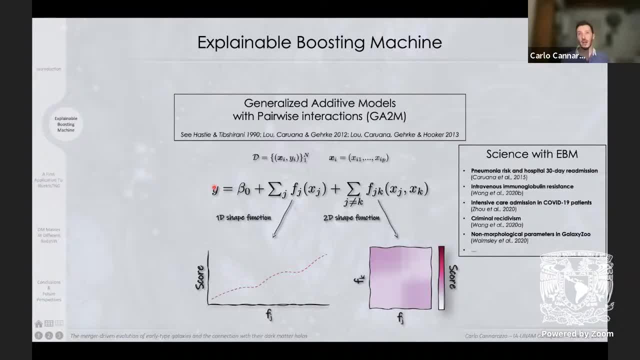 conduct a study for predicting the probability of dying because of contracting pneumonia. it is uh. it was also used for conducting recently also um studies on kobe 19 pandemic situation, but also for conducting psychological studies, for instance for shed line, on psychological hidden patterns, on a catalogue of serial killers and in astrophysics. 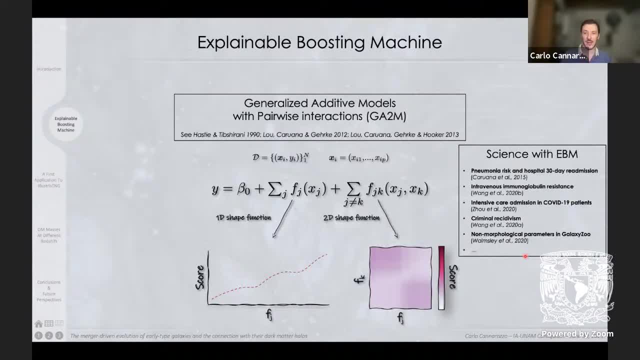 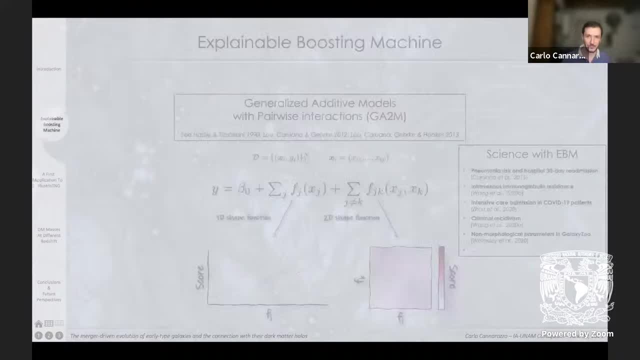 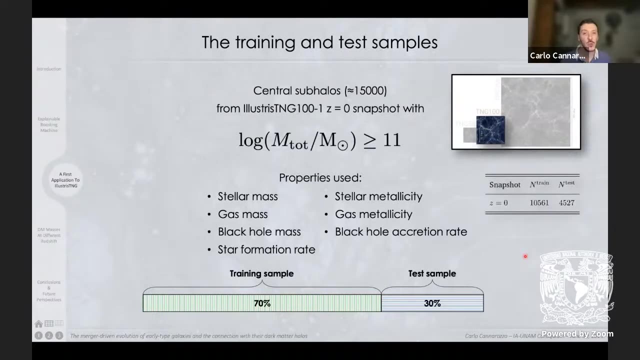 it was used also in by walmsley italian 2010 for conducting, for understanding the role of non-morphological parameters in galaxy zoo. for my first test, for my first application of this method, i selected from illustrious g100, from the red sheet: zero for illustrious. 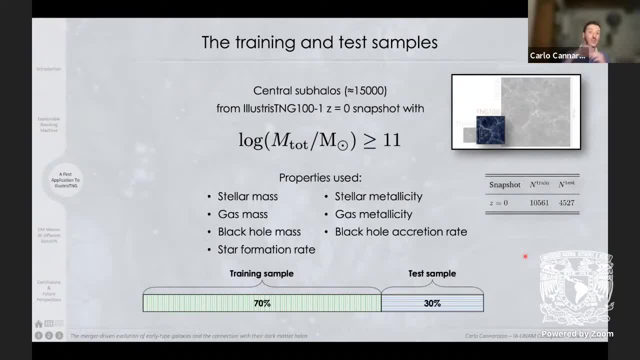 g100, all the central galaxies with a total mass greater than 10 to 11 solar masses, meaning by total mass the mass given by the sum of all the massive components of the dark matter, stellar black hole and gas mass. and to retrieve the mass of dark matter we use the seven properties. so far, 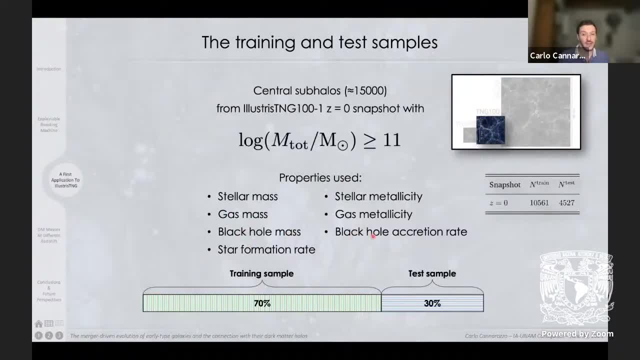 the stellar gas and black hole masses, the star formation rate and the black hole accretion rate amass methodology. therefore, these wasn't explicitly heteroglyphics, although they were studied on aобut. the old my hermanos disorder, in which the我的 mother learned, is then tested on the thirties percent. sample remains arod study. i have a model of two elements related to the picture, email cлятьv, and i put data more specifically on the putting the crystal cluster data and how it is associated with the see, how it works and the analysis of these. dona've erhu interest in physics and registered fundamental master Range reflex to fields what leben y luciano versus the science of galaxy. take two elements and both known to being too deep for reason i. the total sample i derived andilation spring up from illustrious stingy is composed by more than 15 000 central galaxies. i split into a sub sample the 70% of the same or the original same pool is employed for training. the model and what the model learned is then tested on the 30% centその la Punktual other是. 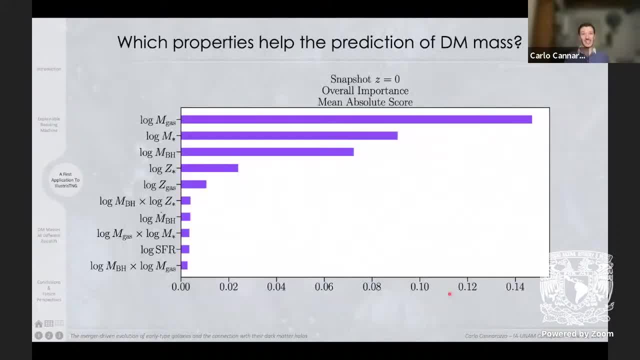 and on this 70 sample, this is what ibm learned. this plot, the overall importance plot, is telling us: uh, which is the relative role in making the inference of the mass of dark matter, halo given by the features that you are using, and also the pairwise interaction, the three most relevant. 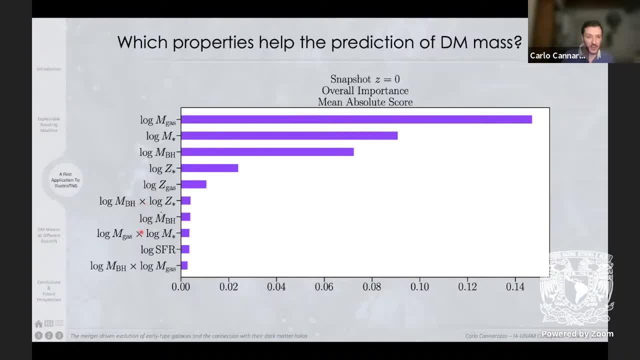 payways, interaction found by ibm, indicated here by the crosses. as you can see here, all these 10 terms are giving their important contribution for making the final inference of the mass of dark matter hairs right. but what i would like to uh twilight is that the baryonic components at 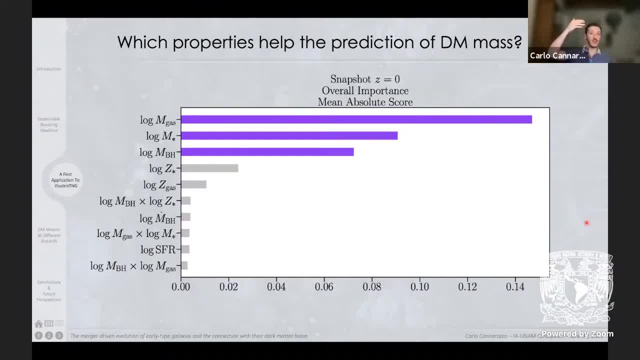 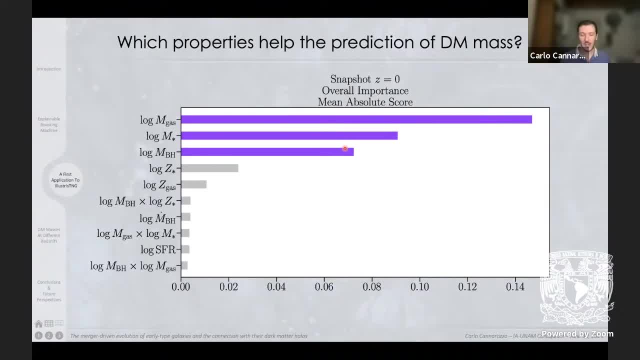 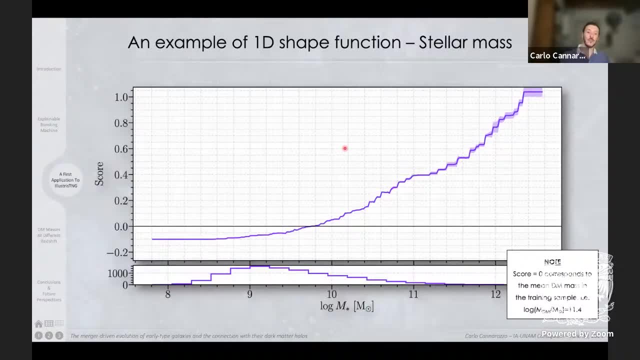 components of the baryonic, components of the stellar mass and the black hole mass. and, for instance, i would like to show how the 1d shape function of the stellar mass appears. um, here on the x-axis you have the stellar mass range of your, of your training sample. 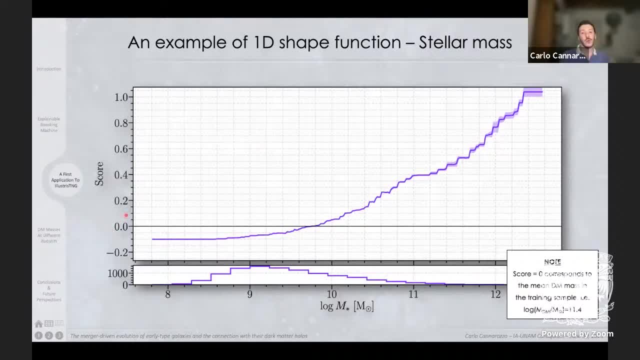 while on the y-axis you have the score. score equal to zero correspond to the mean of the dark matter in your training sample. that in my case, as you can see here, corresponds to 10 to the 11.4 solar masses. how can i use, for instance, this 1d shape function for the stellar? 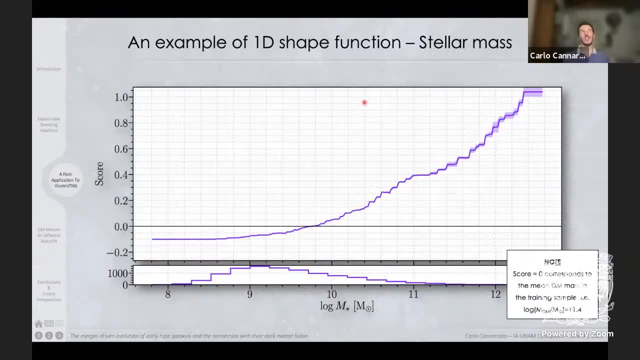 mass. basically, this plot is telling me which is the role to the final inference given only by the stellar mass and, for instance, to the total contribution, to the total inference of all the properties used um a stellar, a galaxy with a stellar mass of a 10. to the 8 solar masses add a. 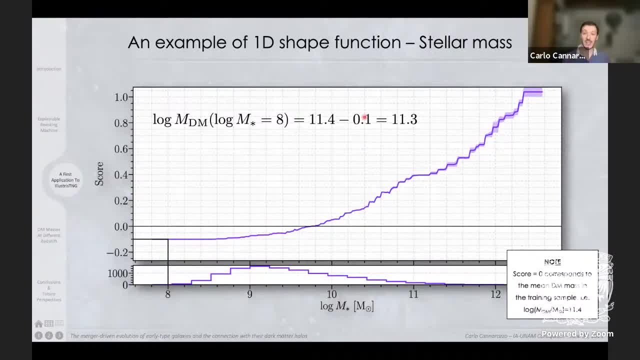 contribution of minus 0.1 to the total inference. instead, a more massive system. for instance, append to the 11 solar masses, add a contribution of 0.4 um. the good thing of ibm, as you can see here, is that this function is not, for instance, a straight line or a note function like a parabola. 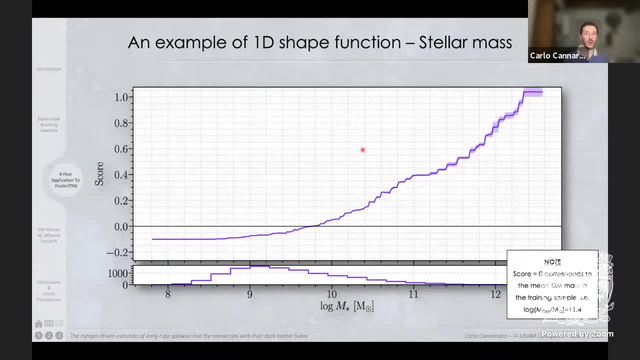 or an exponential or logarithm, but it's a much more complex function and this much more complex function is a much more complex function. and this much more complex function is a much more complex function allows us to highlight peculiarities on the training sample we are using for training. 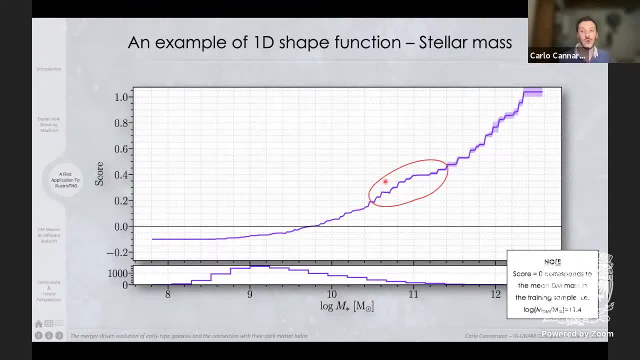 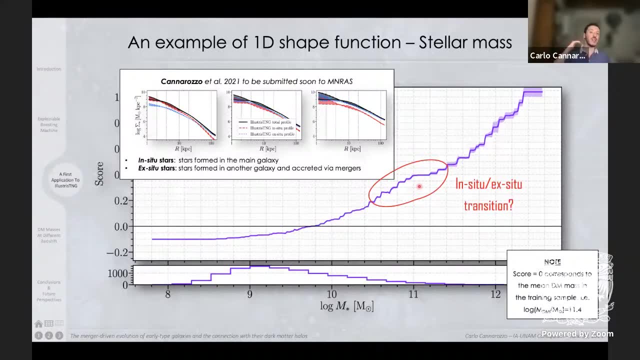 the model. For instance, here around the 10 to the 11 solar masses, there is this transition, there is this hump-like structure, As I showed you in the previous results. this hump-like structure can be explained in terms of the fact that, above 10 to the 11 solar masses, 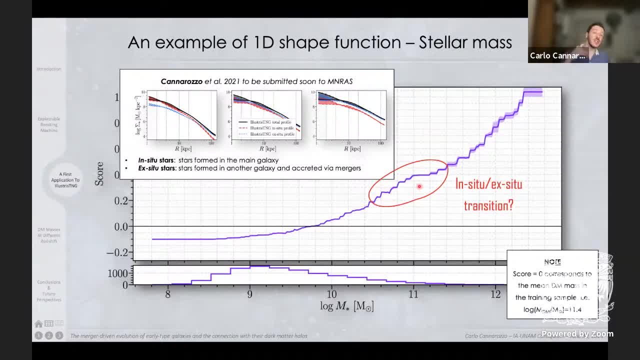 as I already said, the exogenous talent component becomes as relevant as the incident component, or even more relevant than it. Anyway, our EVM model learned something by the trained sample, and so we can test what it learned on the test sample. And these are the predictions. 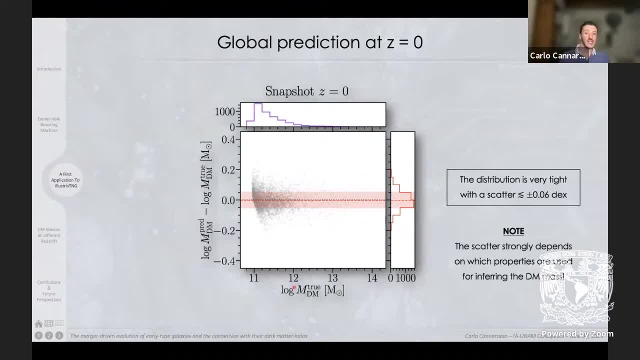 made for the test sample. On the x axis, you have the mass for the test sample: galaxies directly derived from the simulation from illustrious energy. instead, on the y-axis, you have the residual, so the difference between the mass predicted by ebm and the mass from the simulation. and, as you can, 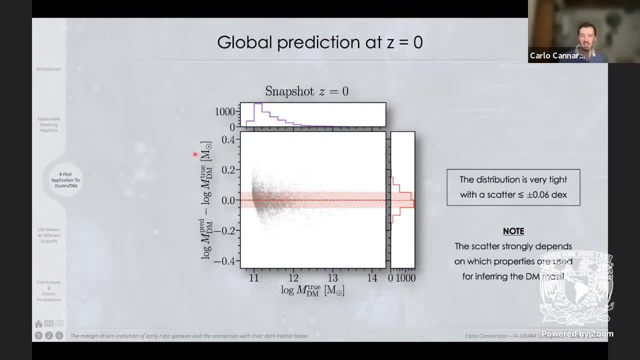 see here. ebm is a is fantastic in this sense because it funds a very a distribution with a very, very tight scatter smaller than 0.06 decks, and in this sense ebm is very prompt, is a very promising tool because it allows to accurately provide an estimate of the mass of dark matter. 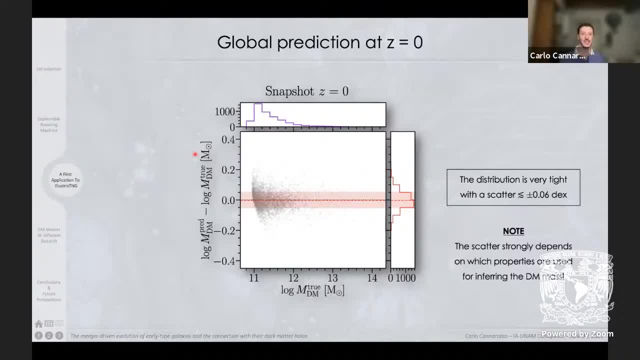 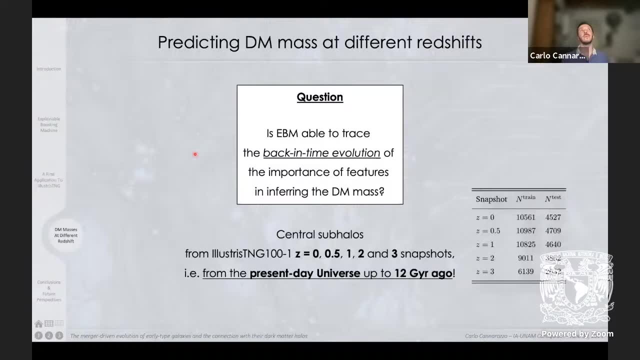 in the sense. but i did more than this and for instance, i extended the analysis toward eiger and dagger redshift in tng in order to understand if ebm is also capable to understand if the importance of given features change as a function of time. to do that, in retrieving the mass of dark matter hairs of course, to do that i analyzed um also. 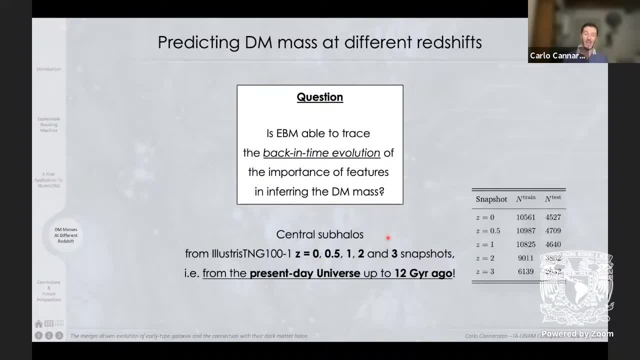 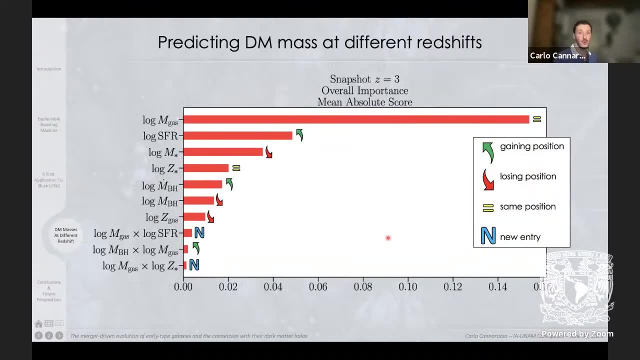 other snapshots, from redshift 0 up to redshift 3, and for instance, here i show you the same plot of before, but for the overall importance plot, but for the redshift 3 snapshot. here there are some, some differences. there are some new entry, payways, interaction, some of the terms that 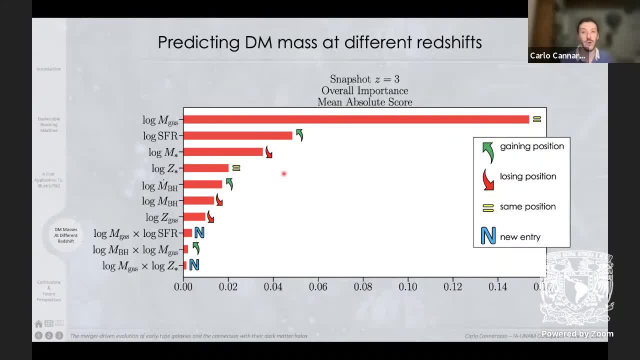 are in the same position. of the zeta 0 overall importance, for instance, the gas mass is again is lying on the first position again. but what would i like to show you is that while at redshift 0, the stellar mass and the black hole mass, 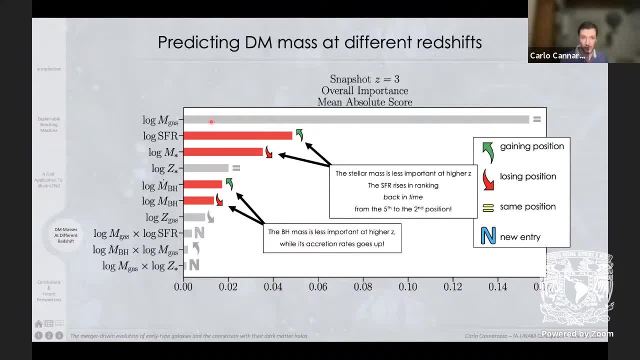 occupied the second and the third positions respectively. now at redshift 2. with redshift 3, the role of stellar mass and black hole mass go down, while the star formation rate and the color christian rate go up, and this is a very good thing, because ebm is also capable to trace this change in the evolution, and this is 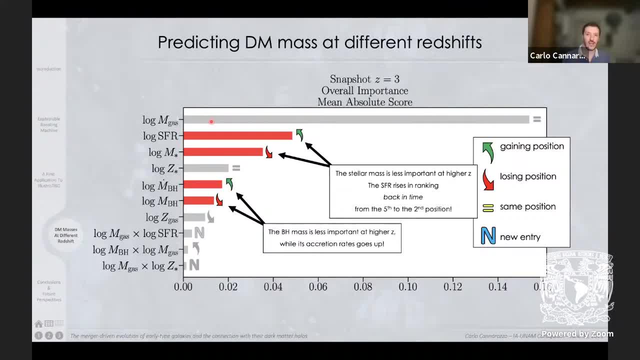 something that is expected from theory, because we know that the tiger redshift, the galaxies form the more and more stars than they counterpart in the present day universe, and also that the black hole accretion rate at tiger redshift is much higher than also passed in passive galaxies today. so, in conclusion, this is, uh, uh, still a very 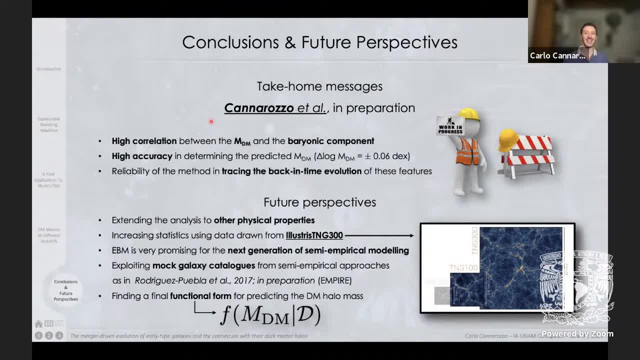 still ongoing project. it's a number. it is still in an embryonic stage and the aim of this work is to compare. um is is to train a model based on simulation- cosmological simulation- for deriving a functional form for predicting the mass of dark matter hails in real galaxies. so far, 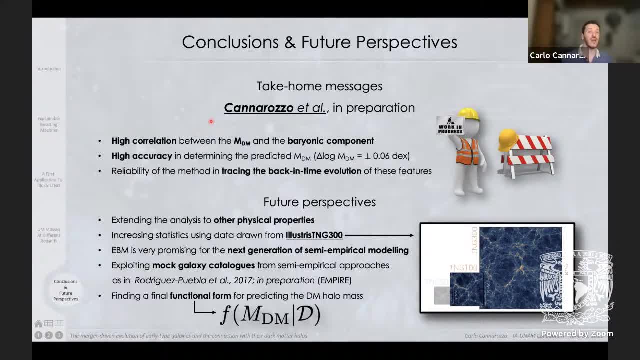 and i think that this is a very promising tool because it finds a very high correlation between, and provides a very good estimate for, the mass of dark matter, finding that, for instance, the baryonic component, like the mass gas and black hole masses are the three most relevant estimators for them. 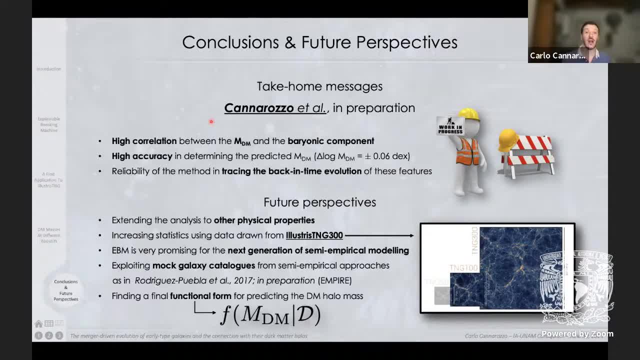 and the and the estimates of these dark matter halo masses are very accurate, with a scalar lower than 0.06 that's, and it is also uh able to trace the evolution, the back-in-time evolution, of the importance of the features used in your inference. what the future of this work? there is a very uh huge stuff for things to do. 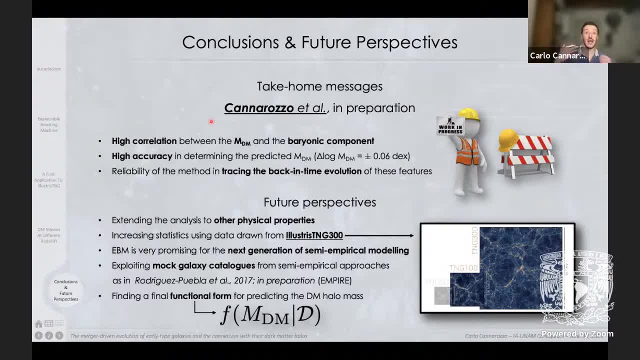 uh, i'm going to extend my analysis, um, adding other physical properties. uh, i'm going to increase, to enlarge my sample including galaxies from the larger simulation, illustrious stingy 300, and this, and since evm, is very promising tool. i think that it is very pro, very promising tool also for um. 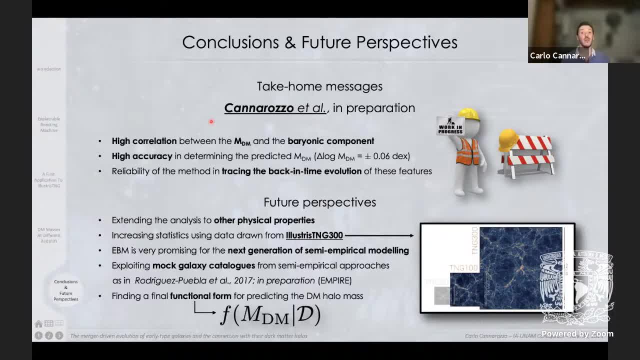 comparing and constraining the next generation of semi-empirical models for understanding the, the mutual role between the dark matter halos and their host galaxies, and then going, for instance, to exploit galaxy catalogs derived from empire or other semi-imperial uh models, for instance the one um developed by rodriguez puebla, by aldo, and then the final aim would be: 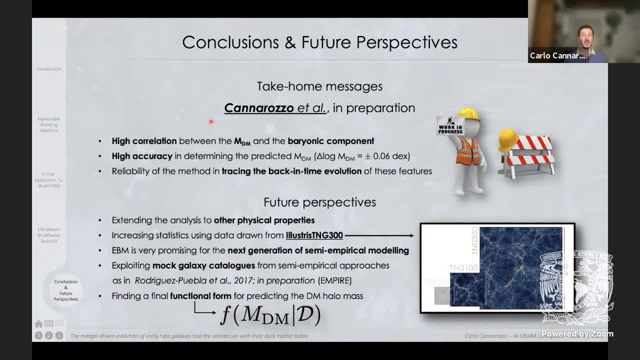 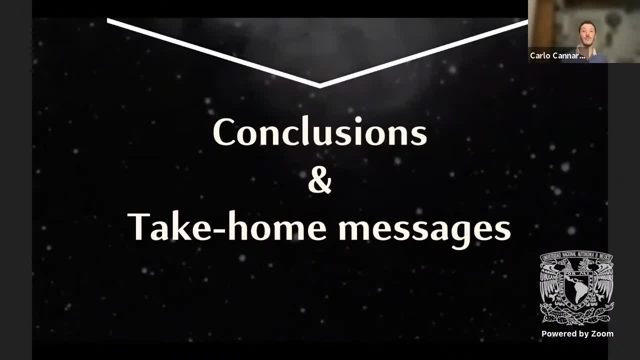 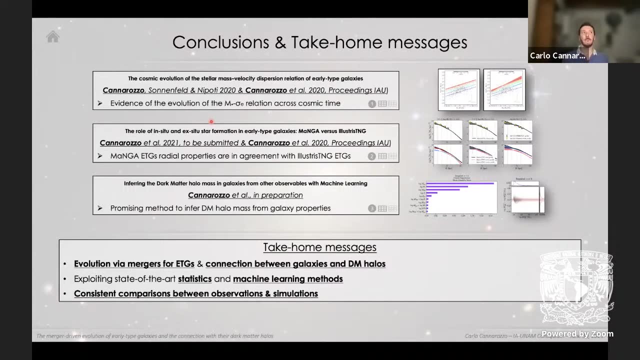 to find a functional form to predict the mass of dark matter halos in real galaxies. so i want to leave you with my conclusion and, uh, let me give you just the take-home message of these, uh, of these works i'm involved in, um, i find that very evidence for the evolution of early type galaxies and 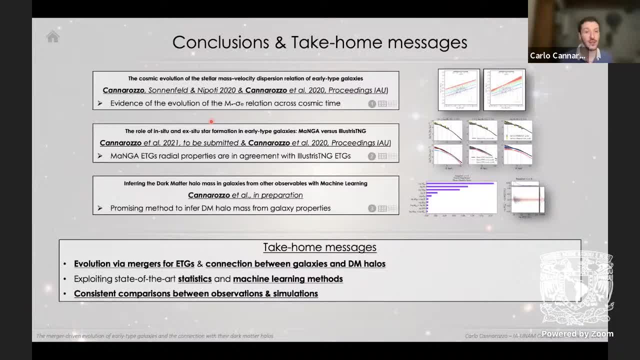 confirm the previous evidence of the measured dream and evolution behind early type galaxies, and also i'm studying uh the very intriguing field of the connection between dark matter, halos and their host galaxies. um, i would like to uh underline the paramount need of exploiting state-of-the-art. 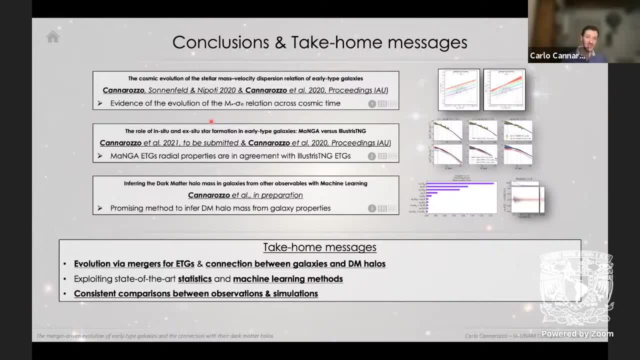 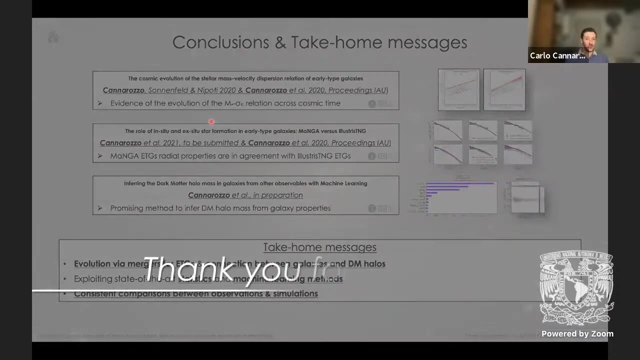 catenage, uh statistical, advanced statistical and machine learning methods for comparing observation simulation in consistent ways- as consistent as possible at least, and also to handle this huge amount of data that are going to come from the next generation of surveys. i think that that's all. i'm open to your question and thank you for listening me. 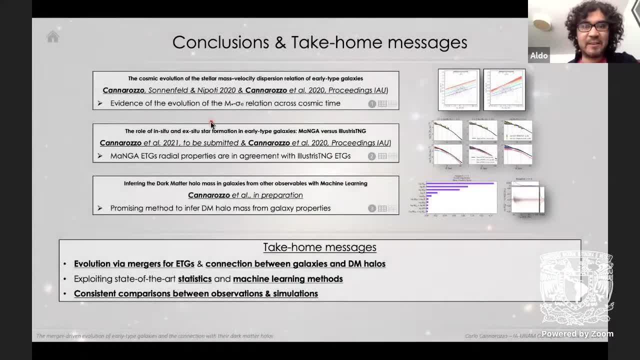 okay, thank you very much, carla, for this nice presentation. is there questions or comments? for carla jorge aldo, can you hear me? yes, okay, uh, thank you, carla for the nice talk. i have a couple of questions regarding your results from the manga survey. uh, i'm pretty sure i missed it, but 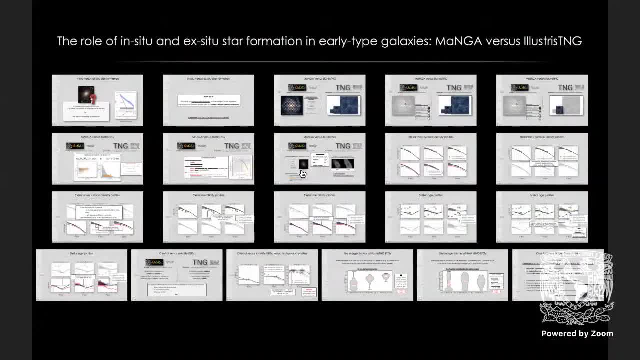 uh, you mentioned. oh well, you have a comparison between illustrious and the mass and the example from manga, right? so, judy, you do this comparison between TNG and Manga for Redshift 0, right? Is that correct? Yeah, yeah, yeah. 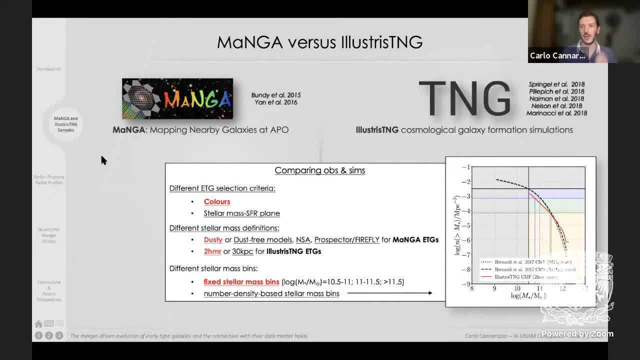 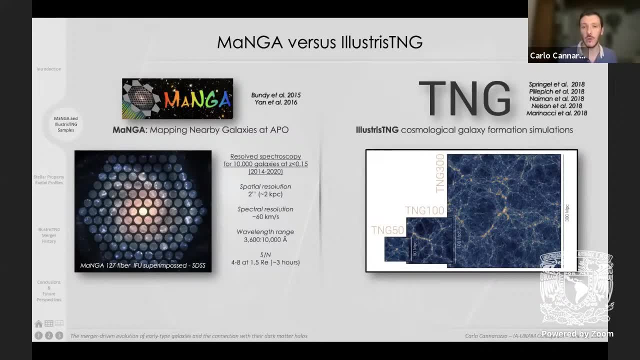 Because Manga, of course, lies in the Redshift range in the present day universe below, yeah, around the Redshift 0, yes, So I did this comparison with the Redshift Snapshot from TNG 0.1.. That is more or less the median Redshift. 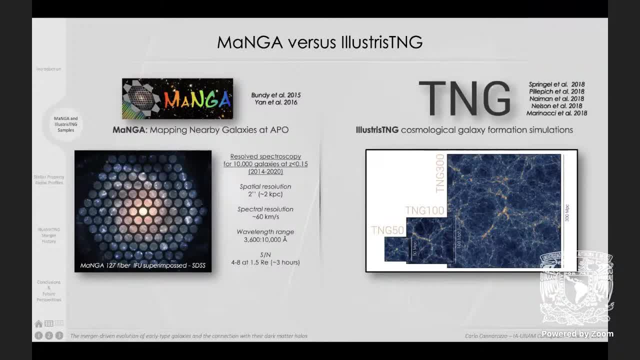 of the observation in the Manga survey. Yeah, exactly That's what I was going through, Because if you look at the mass Redshift distribution of the Manga, there is a significant- I mean, it was designed to be like that. A bias for massive galaxies tend to be at higher Redshift. 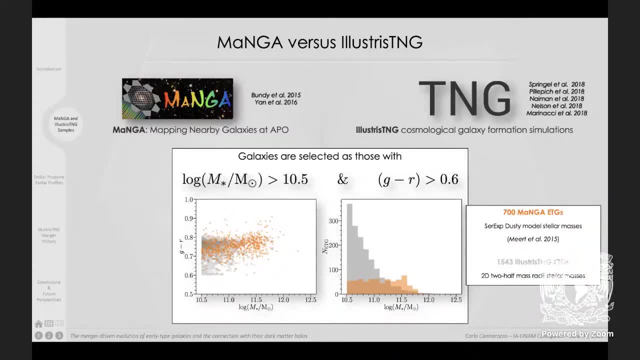 in comparison to low mass galaxies. I'm pretty sure you know that, So I was wondering if you could have to quantify that bias, that you observe That there is this intrinsic bias from the Manga sample, in order to compare with your illustrious simulations. 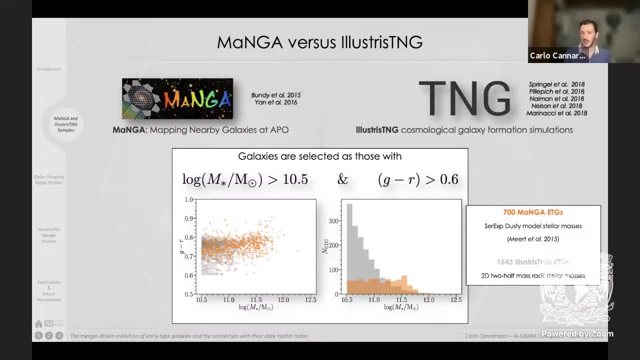 Yeah, Basically, I haven't done it yet, in the sense that the aim of this work was properly to compare Manga and TNG, So to provide a scenario of the present day universe galaxies. It's something that I should, Yeah, Yeah. 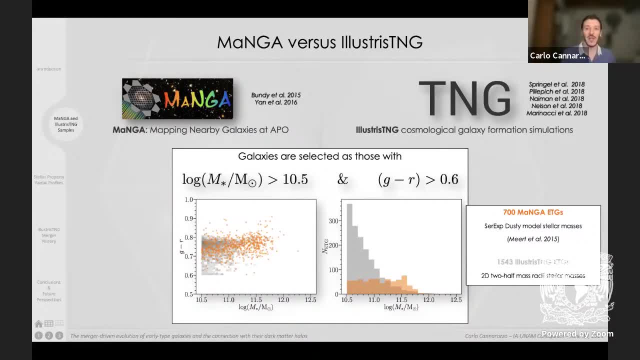 It's something that I will do in the future, of course, And this is something that I cited before, because I would like to reconstruct how individual galaxies in TNG evolve through cosmic time And, in this sense I can, in order to explain how their physical properties evolve. 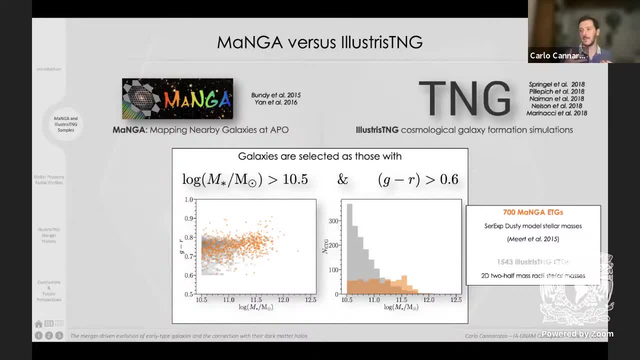 through cosmic time and in this sense I can provide an answer to this question. to understand if there is a bias that varies as a function of time. Yeah, I will encourage you to check that, because it's a significant difference in time if you have a low mass galaxy or a massive galaxy in Manga. 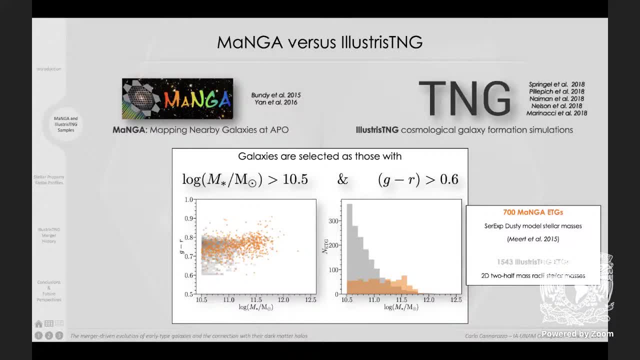 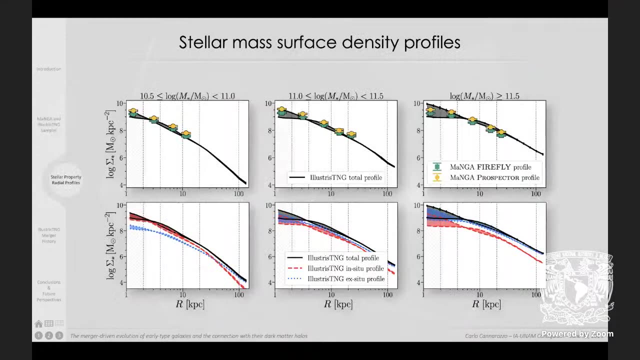 So that's something to consider. The second question that I have is that you show a royal profile between the simulations and the data that you use with the- I think it's Firefly and Prospector. Yeah, I'm not surprised that you have a significant, I mean. 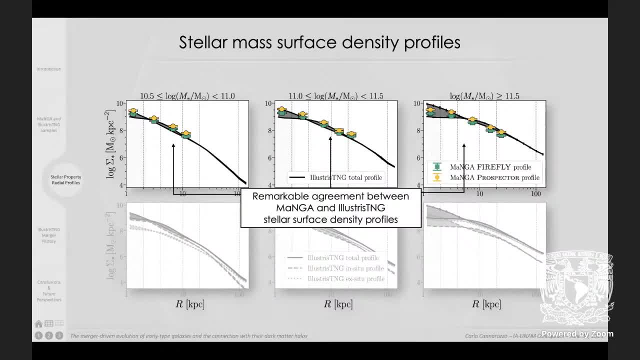 I would be really surprised and concerned if you don't find a significant match between the observation of the stellar mass surface density profiles and those from Illustrious. But you do seem to find discrepancies between the two. The metallicity, the stellar metallicity, and the age. 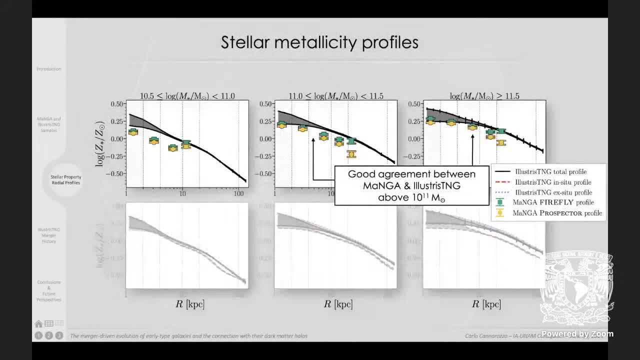 and the profiles. So can you comment on that, like those ones? Yeah, Can you comment on those differences? Of course, The first thing that I would like to say a priori is that the reason why for these three quantities, 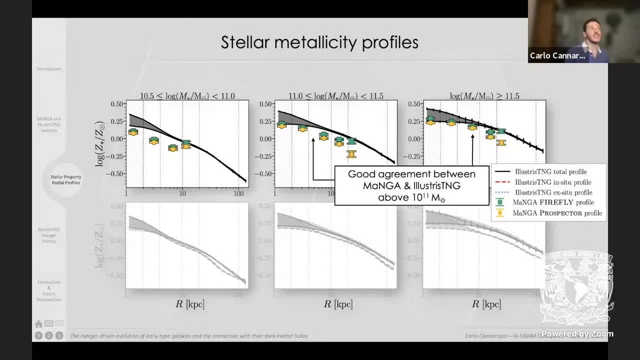 metallicity, stellar surface density and age. we decided to use two fitting code. that is the one that I said before. So the fact that stellar fitting codes can provide, in real galaxies, different estimates for the same galaxies about the same stellar physical property. 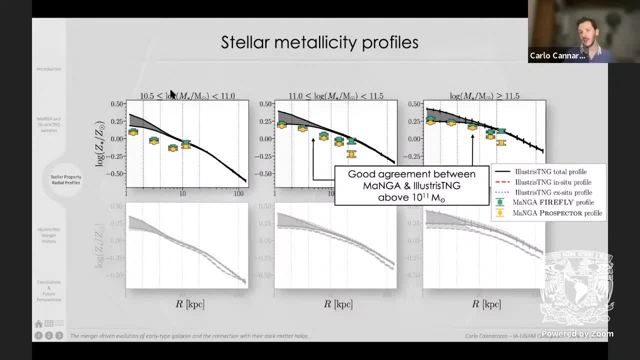 At least for the metallicity as you can see, in particular above 10 to the 11, at least the shape of these metallicity profiles are in a in enough good agreement, in particular above 10 to 11.5 solar masses. but this match is not so good as you can was saying below 10 to 11, because even if 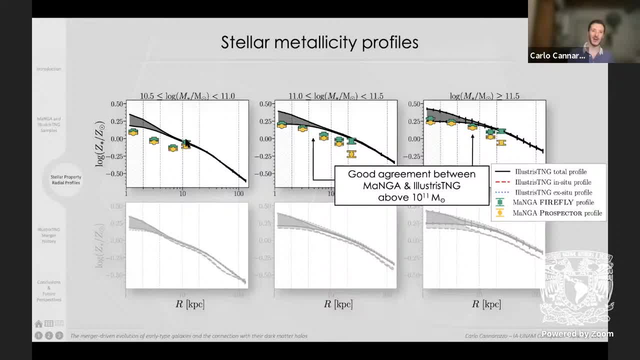 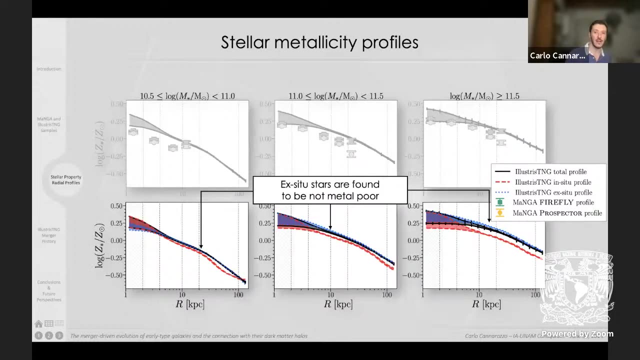 although these are two outliers, because there are a few, a few more points here, but at least there is here the square pansies over point two decks in this direction in the stellar mass, and the situation is it's harder here for for the agent. then one of the main reason of course is: 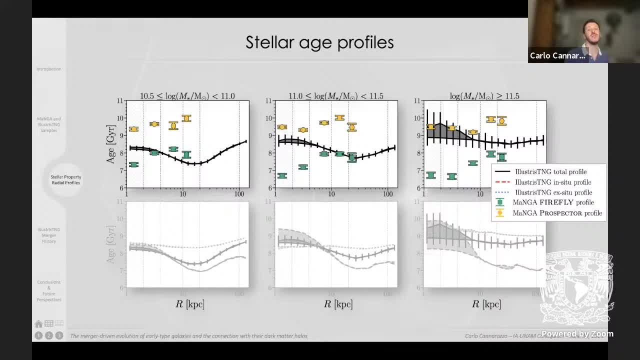 resides in the, the receipt behind the implementation of illustrious tng, because maybe the agent feedback inside this galaxy is, maybe can be too high in this kind, in some kind of these systems, and so um this, these discrepancies, i think i suppose that in future from the, from the illustrious tg team, will be improved, because 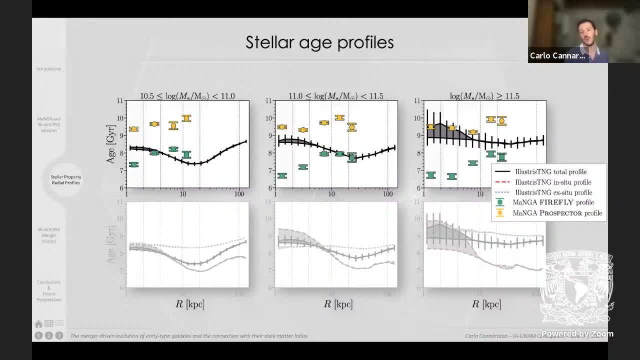 i think that basically is due to the receipt on how the physical implementation in the physical, the physics behind the formation, evolution of galaxies in kingi is uh implemented. i think that is something related to the particular to the uh, to the effect of the agent feedback that may cause this. these 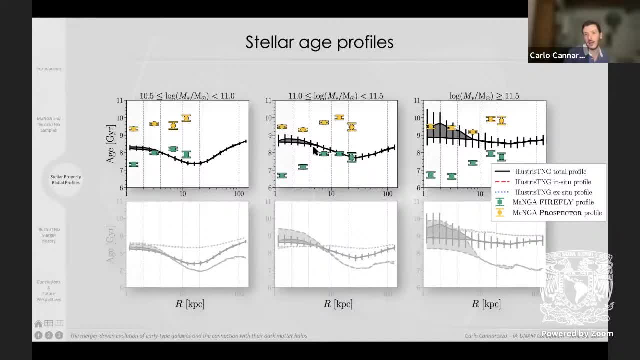 systematically shift. uh, the good thing again here is that at least the h profiles lies in between this to these two profiles of firefly perspective, but here the situation is more critical than the and the stellar surface density. of course, Yeah, exactly. So that could be, as you mentioned. 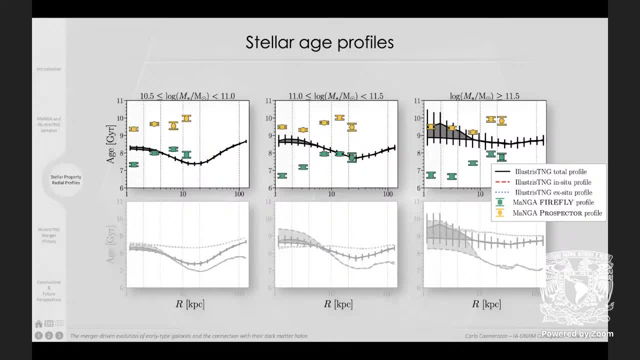 a combination of effects. On the one hand, you may have the physics that you are injecting to the simulation, But on the other hand, as you can clearly see from this comparison between Far and Far and Prospector, the differences in ages is the order of almost 2 giga years. 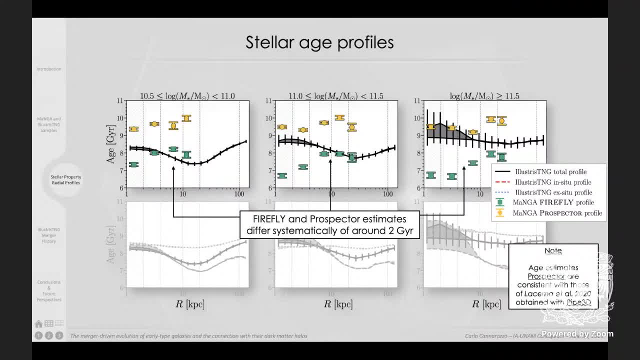 Yeah, 2 to 3 giga years. So it will work to explore what was causing this difference between the different single-stellar population-fitting techniques. OK, that's great. Thank you for the nice work, Carlo. Thank you very much. 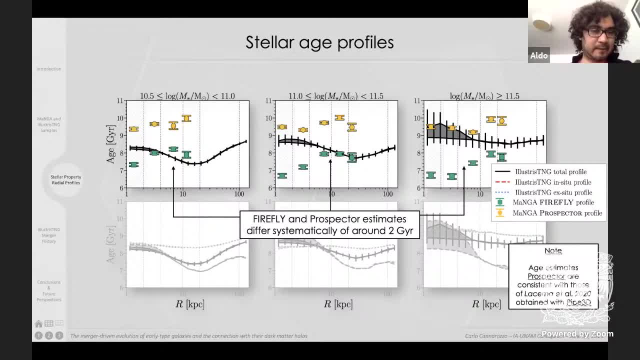 OK, so Silvia, Vladimir and then Octavia. OK, my question is very simple. On the last section of the talk, you mentioned that there is a relation between, or the dominant diagnostics can be the gas of the mass, the gas of the stars. 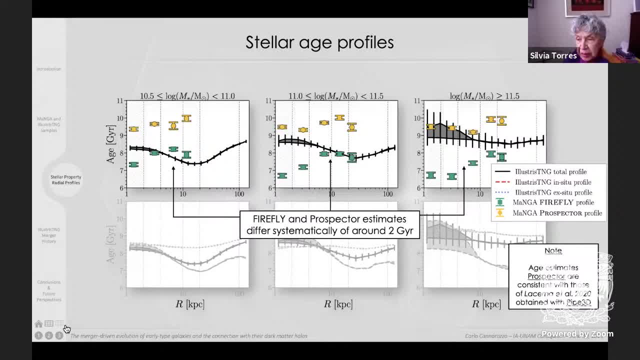 and the mass of the black hole to determine the mass of the dark matter. Now, what are the physics of that And how come these changes for different z? I mean, if you go to different z you have different diagnostics, dominant diagnostics. 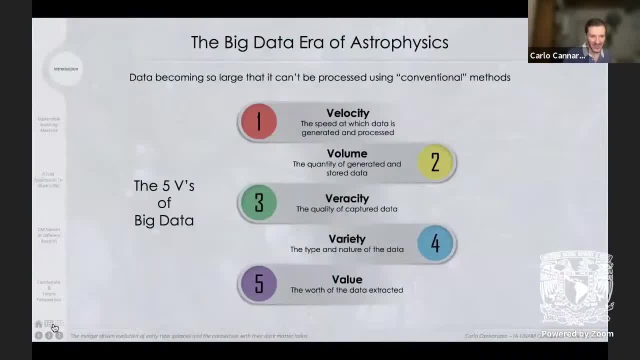 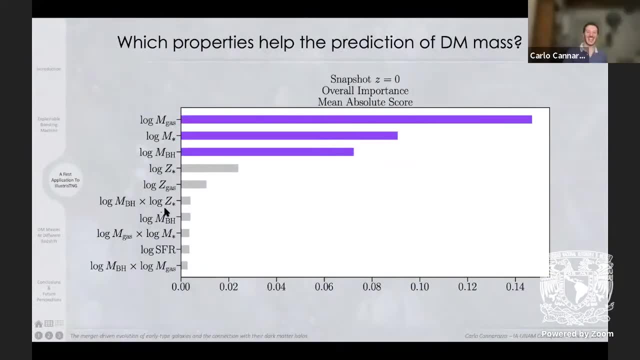 What do you think? Yes, Thank you, And I know that the mathematics is what you have, but I want to speak about the physics of this. Yeah, yeah, yeah, I understand. Yes, of course, here at redshift 0,. 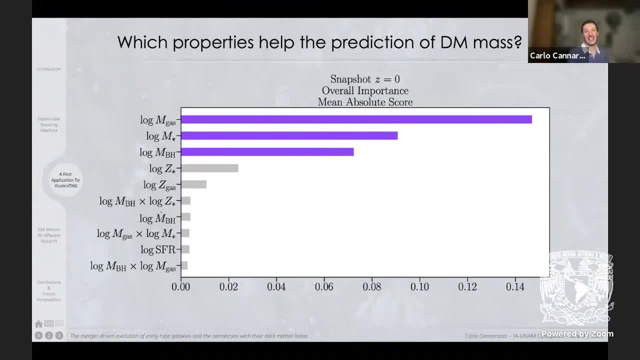 and it's not still valid at higher redshift. the gas, the stellar and the black hole masses are the three best estimators. The explanation, the possible explanation for this is due strictly to, at least for the mass- OK, For the gas and the stellar mass in terms. 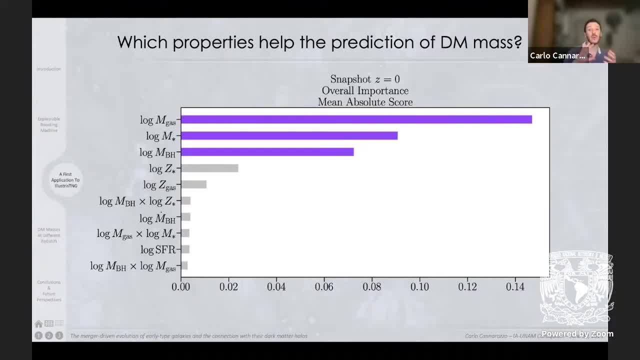 of the baryonic component, the dynamical aspect, Because in these systems the galaxies now are relaxed, So, dynamically speaking, stellar masses and gas mass are gravitationally bounded to the dark matter. So I think that it's unavoidable that these are. 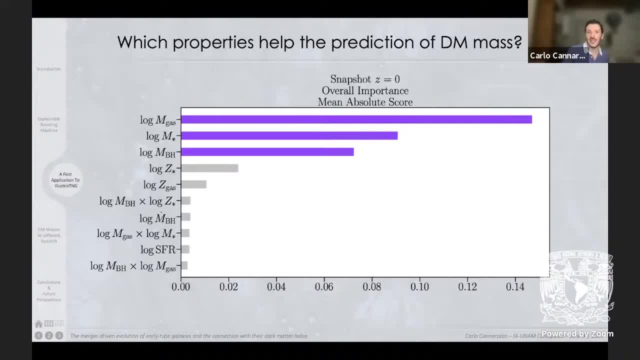 the two best estimators And, of course, for instance, the stellar mass is the up to now through. the stellar to yellow mass relation is the. I think that is the most well-studied, the most well-known relation. 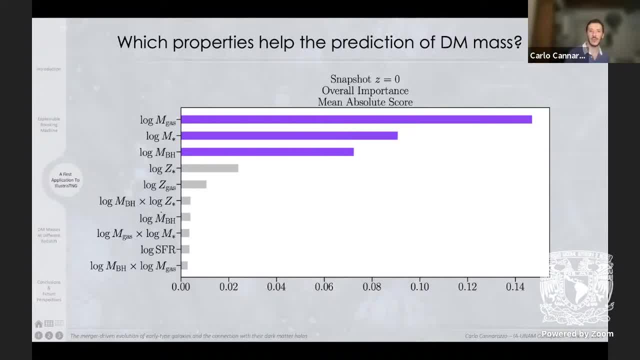 Because it is very easy to retrieve the stellar mass under some uncertainties, but it's something that is, I think, gravitationally bounded, So the origin is on this direction, The fact that dark matter, halos, gas and the stellar mass. 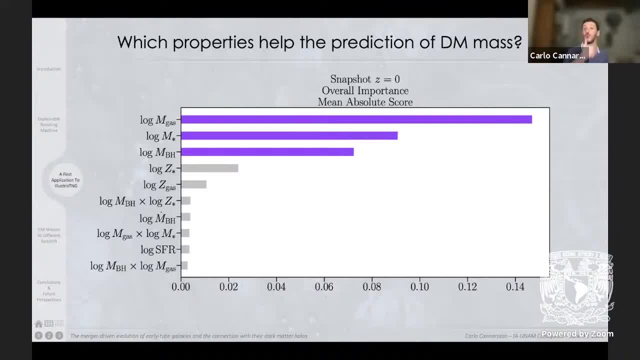 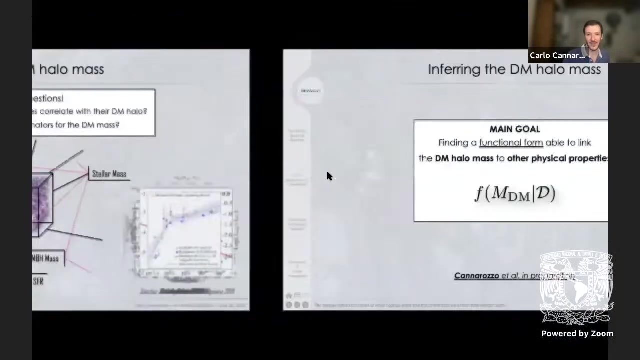 share the same dynamics through the cosmic time while deep galaxies evolved. The fact that the black hole mass are strictly related can be due to several factors. One of these factors was the one that I showed you before when I at the beginning of this part, because we know that sorry. 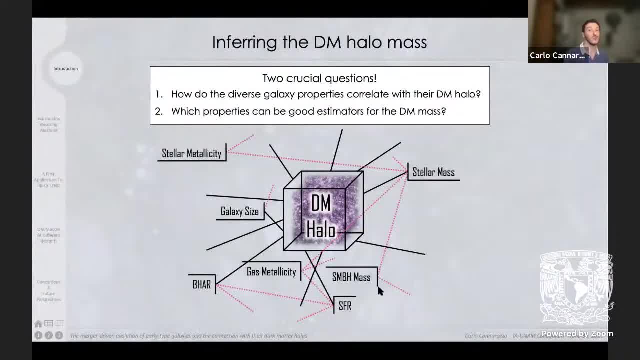 that the stellar mass directly is linked with the supermassive black hole through the Magorgian relation. And so if there is this link between the stellar mass and the supermassive black hole mass and there is the already link between the stellar mass, 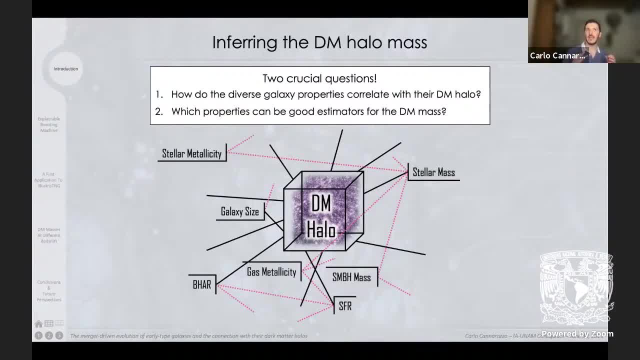 and the yellow mass. I think that also there is a hidden link between the black hole mass and the dark matter here, Hello. So that is why- at least at redshift0, after all the physical processes occurred in these evolving systems. these are the three most relevant components. 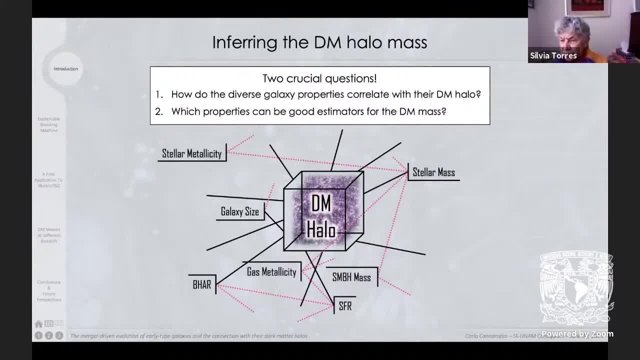 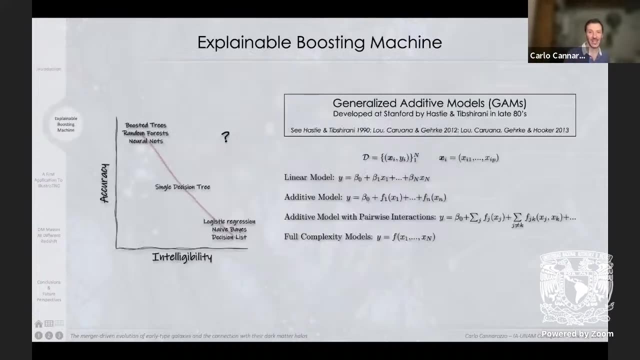 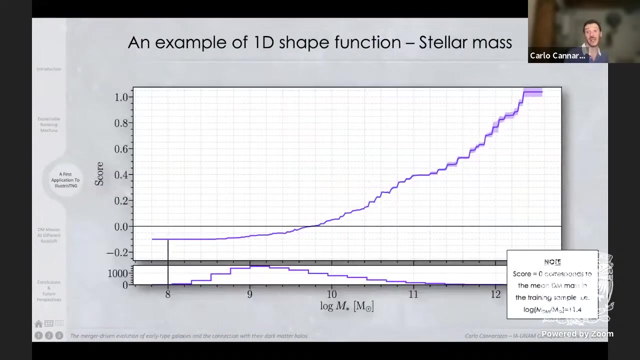 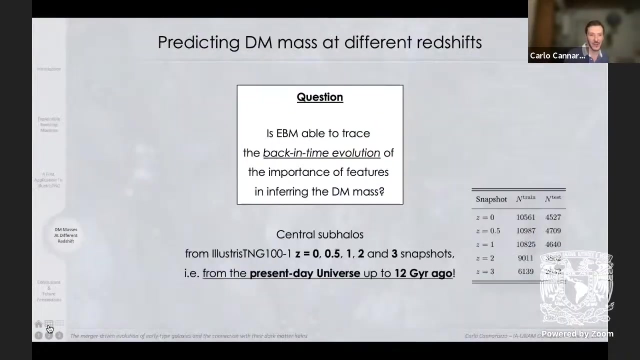 I think that you can see that the indicators were different parameters. Yeah, Hang on. Yeah, Because at redshift3, as I showed you before, for instance, the gas mass- because it's the second most dominant component in a galaxy- is the- sorry- the most dominant component. 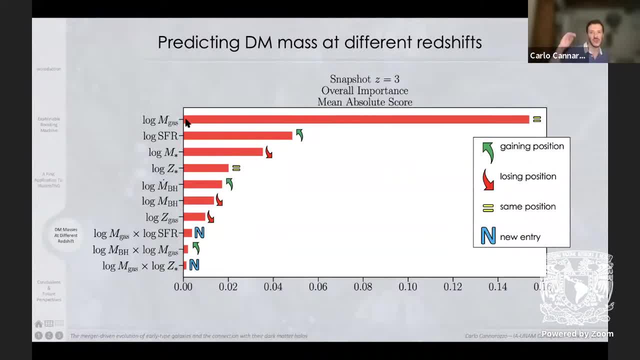 is gravitationally bounded and it remains in the first position. The fact that the Tiger redshift, the stellar mass and the black hole mass go down- Yeah Is- can be due to the fact that these galaxies are still evolving And they are not in equilibrium, because I 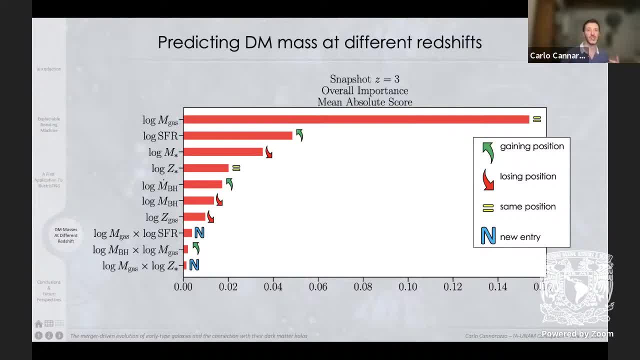 think that these galaxies are experiencing a lot of mergers And so the mass is not well. the mass of stars is not well defined, in the sense that the galaxy is not at its last stage, It's not in equilibrium, And Yeah. 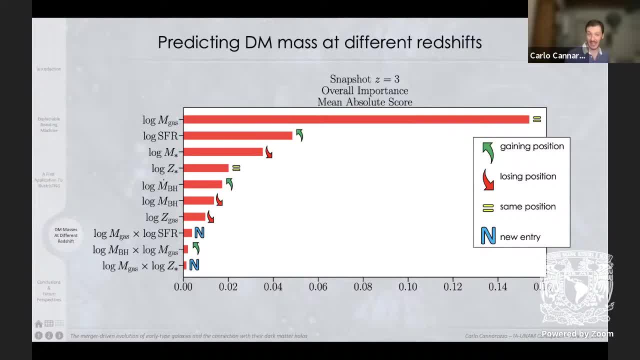 Yeah, Yeah, Yeah, Yeah, And I think that it's something that I'm I'm- I'm studying it now in the spirit of conducting this work, But I think that the answer is behind these, is in this direction, The fact that this is. these systems are still evolving. 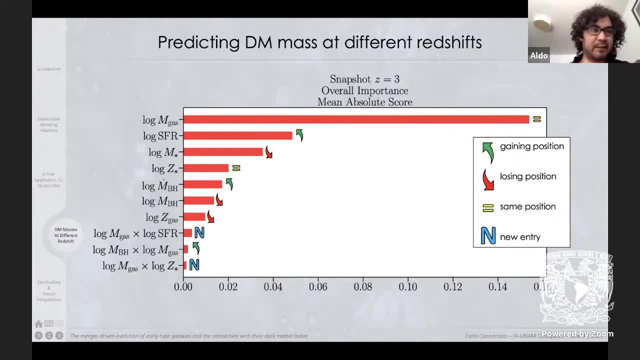 Thank you, Thank you Very nice. OK, Vladimir, Octavio and finally Jesus. OK, Thank you, Carlo, for your very nice presentation. I think you are Yeah, Yeah, Yeah, Thank you Yeah. 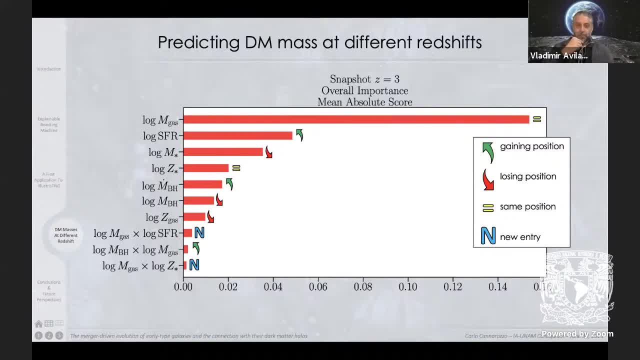 Yeah, Thank you, Because this is the impact we see in our own galaxy. I mean, I would say that in in our own galaxy, the evolution of early type galaxies. we are now in a position to study very hot topics in the field. 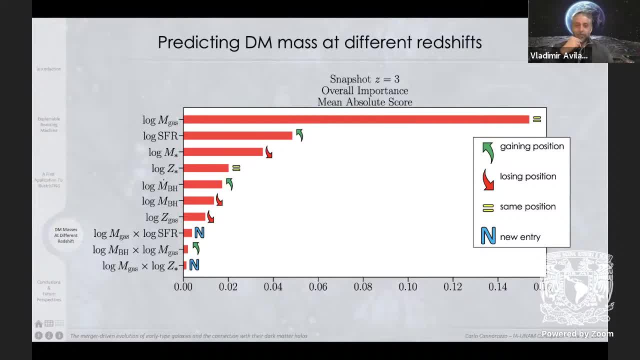 So hot and debatable that probably we are not in agreement with some of results, for example, regarding the role of dry mergers in the evolution of early type galaxies. In and in two papers that we are now preparing, we find that the role of dry 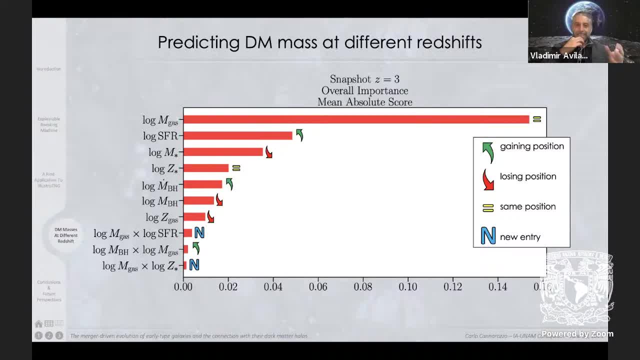 study in the inner regions of these elliptical galaxies, putting 1.5 effective ready and probably you and the Oyarzun et al papers are taking into account larger ready where dry marriage, of course, are more relevant. yeah, 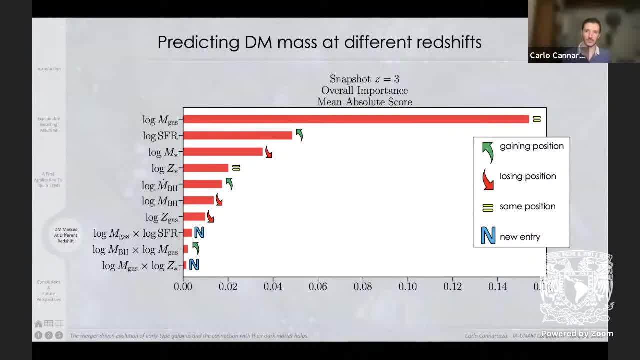 in the growth of these galaxies. So this was just a comment, because it's a very debatable and hot topic. Yeah, yeah, of course I have a question about the evolution of the loss-to-dispersion-stellar-mass relation. 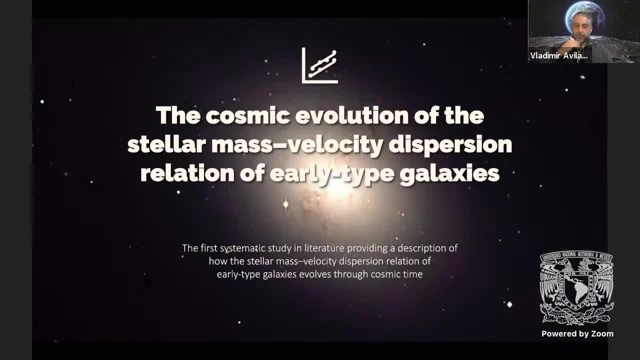 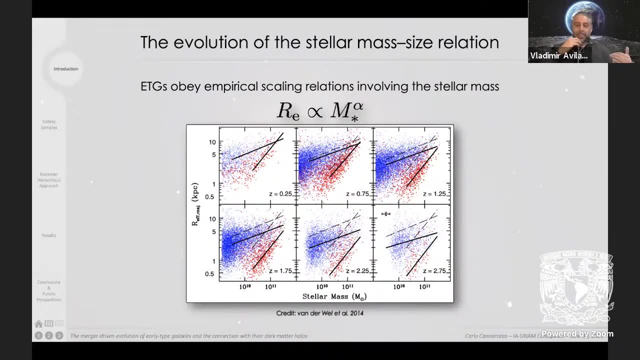 I'm wondering if you consider that your results could be affected by biases typical of using surveys at different red sheets to infer galaxy evolutionary trends, for example, the progenitor bias. Do you know this? Are you taking into account this in your study? 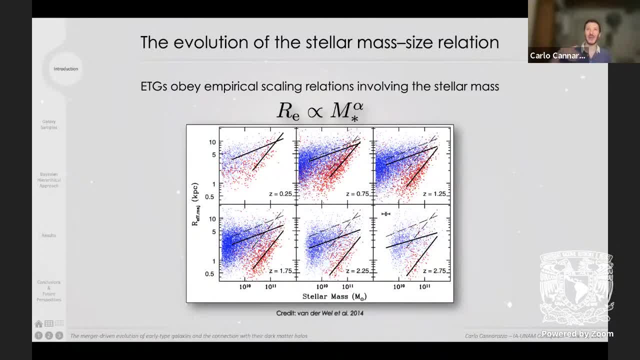 Not so far. That is why, as I said before, I would like to conduct also a comparison between observation and simulation and to quantify how the effect of the progenitor bias also evolves through cosmic time. But what I can say is that in the final results, 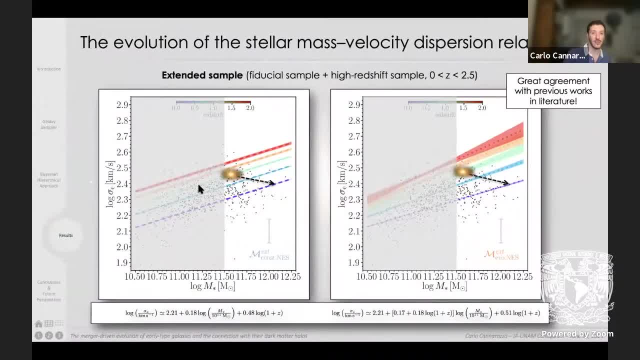 that I show here, qualitatively speaking. I thought to you that I say to you that from redshift one, I think, I suppose that this galaxy moves in this direction to reach the function of form at redshift zero. 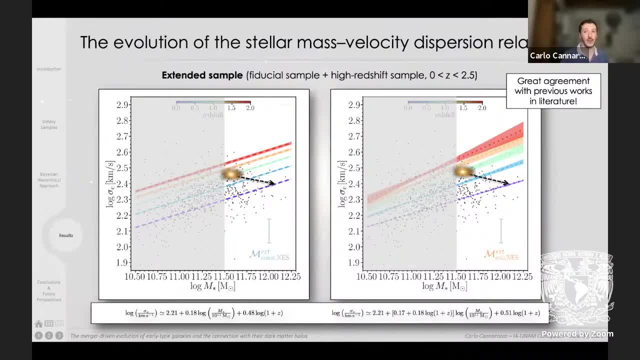 And according to works like Lopez-Sanz-Juan, the progenitor bias should not affect so much below redshift one. So, according to this work, what I can say is that, at least for the fiducial sample, so as this, the progenitor bias and legacy galaxies. 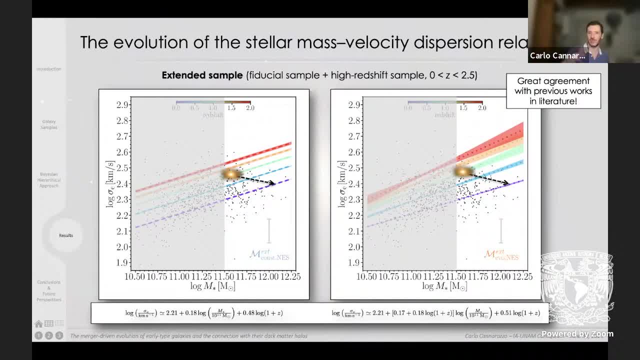 that are, which I redshifted these around. the redshift one: we should not have relevant effects on progenitor bias, But it's something that we already planned to analyze. the making use of cosmological simulation, because there we can address this more easy. 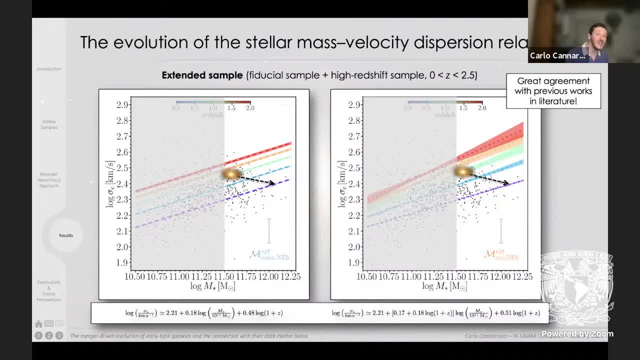 easier this question: if a galaxy is still you know, if a galaxy is still you know, if a galaxy is still, you know, an early type galaxy is a Tiger redshift or was, for instance, a star forming one? 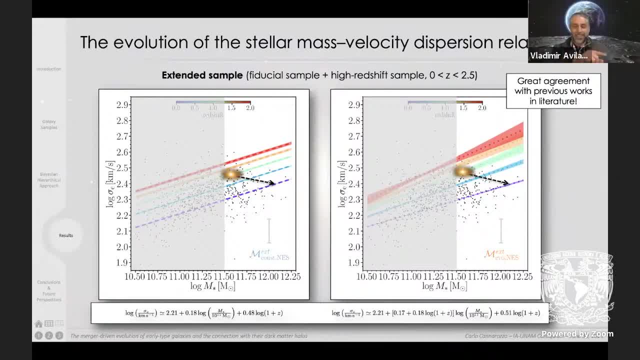 Okay, Thank you, And just a comment regarding the age profiles of the early type galaxies. our results with Pipe3D are in better agreement with Prospector that. there's a Prospector that you showed just to. Yeah, yeah, yeah, yeah. 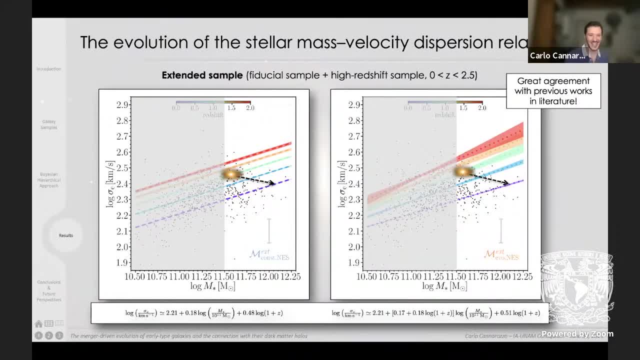 Yeah, I drove. yeah, I written before I. yes, The Prospector and Pipe3D estimates are in agreement between them, at least for age. Yeah, of course, Thank you, Thank you, Just a quick comment on this figure. 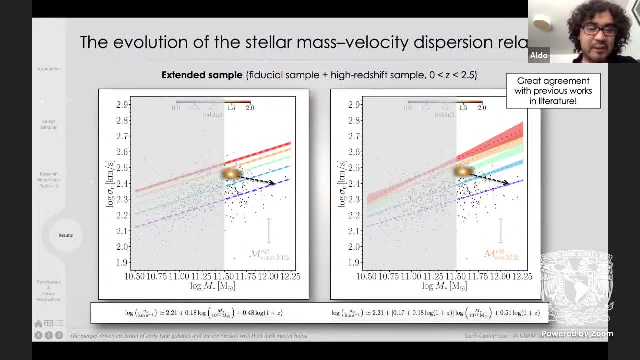 Actually, I also don't believe that he's affected by a progenitor bias, because you also see something very similar with the simulations. When you plot the maximum circular velocity of the helios versus the heliomass, you see the same trend in the evolution. 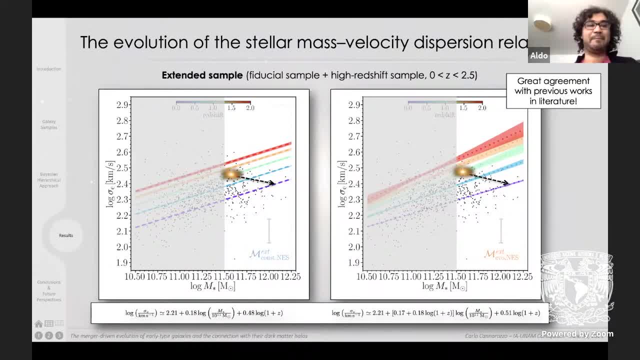 which is actually very encouraging. Yeah, Okay, That was my comment, Octavio. Thanks, Aldo Hi Carlo, Very nice talk. Thank you for the presentation. Just a quick comment on the question. The quick comment is for manga, for example. 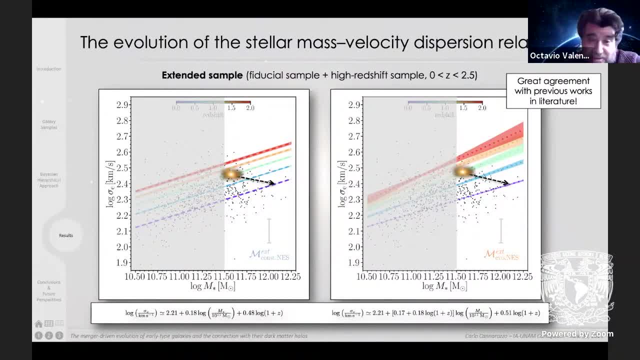 capturing velocity. anisotropy is hard. Also, I believe, for simulation, for illustrious. it's kind of difficult at the small scales to capture anisotropy. My question is if that has an effect in your comparison. it's very good that you say that it's very hard. 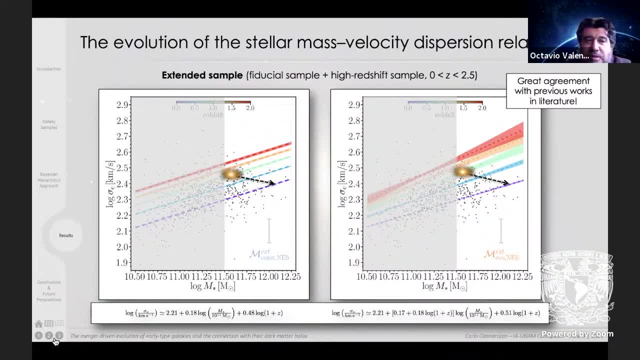 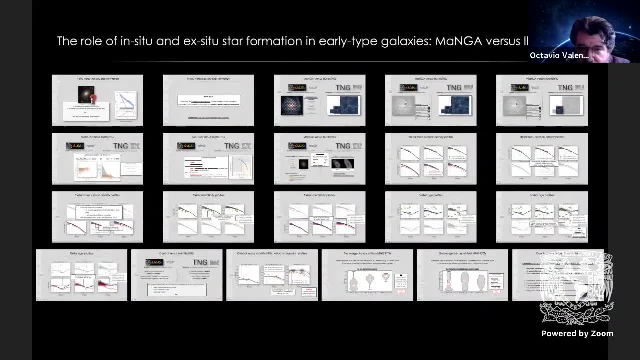 to compare observations and simulations. I'm pleased to see the careful work, but I'm not sure if both of them capture that and if that has consequences for your comparison. This is just a comment. My question is regarding the last part of the talk. 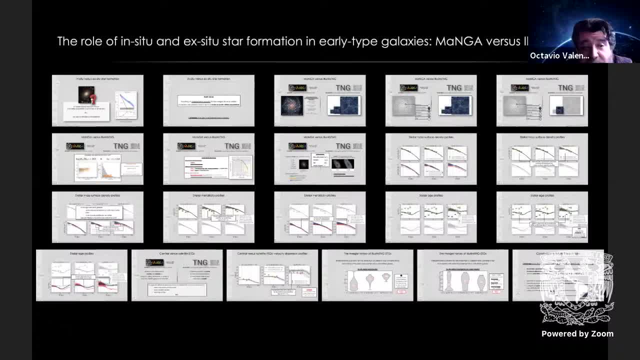 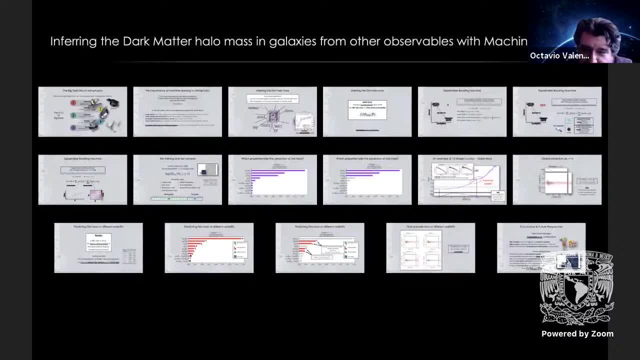 Very exciting. In my opinion, this is the future for this HFV technique. However, as any powerful toy, has to be used very carefully. probably you know the work of Calderon and Berling. They tried to do something similar with different techniques. 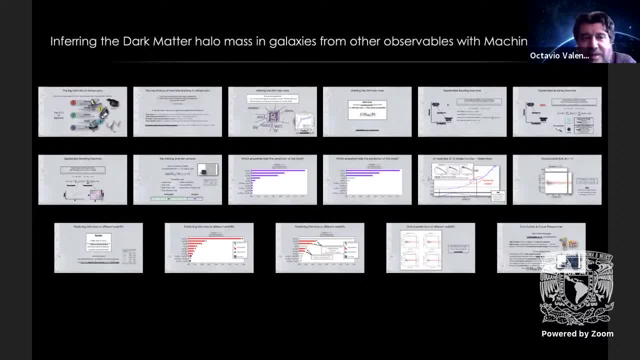 XGBoost random forest neural networks. Do you believe you obtain the same results or different, and how dependent is from the method, the results for this assigning of results, And how dependent is from the method of total mass or heliomass to the galaxies? 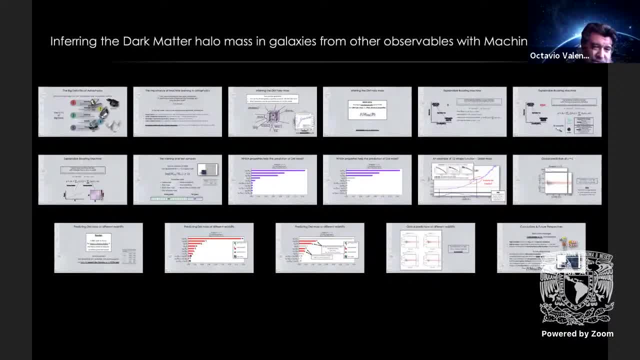 I guess this is one of the key things. when you know, this is there is currently an explosion of using these techniques for many things: photo, photo C and many other properties of galaxies. What do you think? Do you believe your results are consistent? 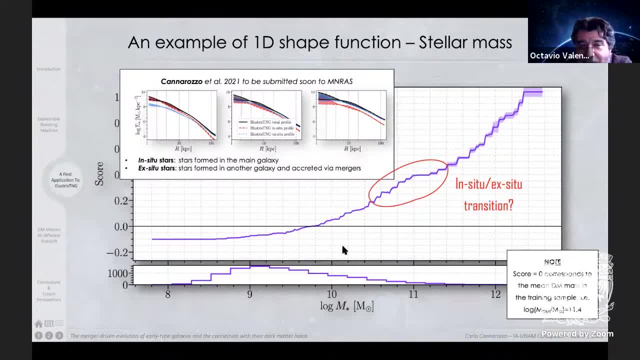 with other applications different. How dependent is from the method. Okay, Thanks, Octavio, for your question. Let me say before that this is my the first time that I'm conducting a work in both in the context of galaxy-helio connection. 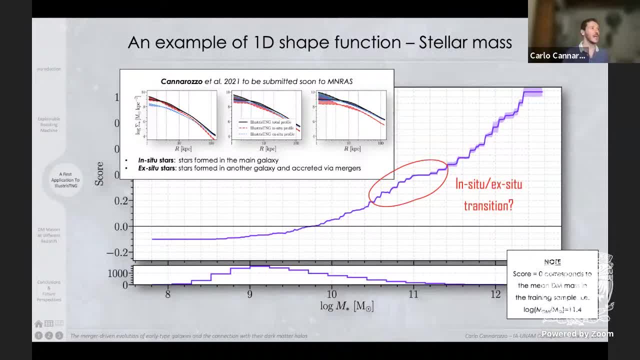 and in machine learning application in astrophysics, And it is very rewarding and it's opening my mind in this direction. I don't know these, the work you mentioned before, but what I can say in this direction is that, as a show before you mentioned, 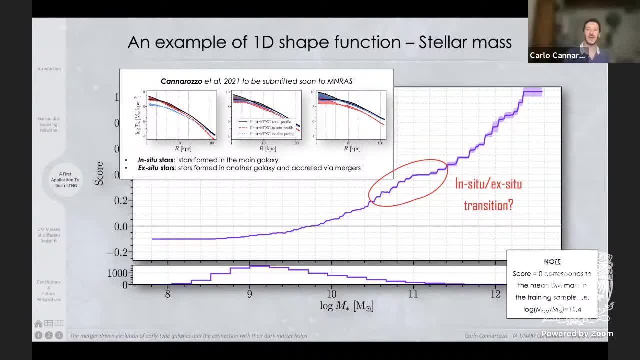 Yeah, What? Sorry, I don't know what's happened. Okay, Yeah, Among the most accurate methods of machine learning there are, as you say, the random forest or neural networks. What I would like to say is that, with respect to these kinds, 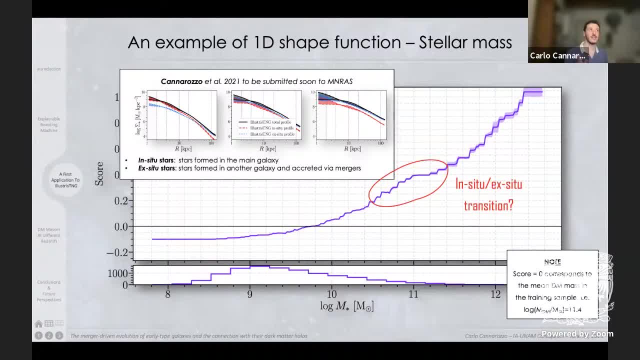 of very accurate models. BBM has comparable. this method has comparable performances in terms of accuracy, but it is very, very, very much more easy to be understood, because with random forest or neural network you cannot have information like these, for instance. 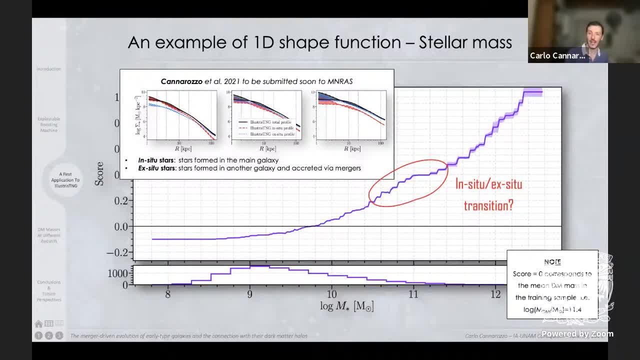 for the 1D shaped function of stellar mass that I showed you before, And this is. I think that is a very good thing because through this shape function and through this method, EBM in general, you are able to understand what's going on in each individual. 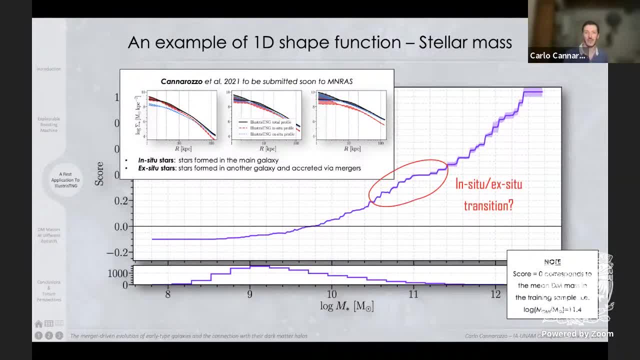 features you are using in my case, for instance, for retrieving the mass of dark matter. So, yes, I think that one should take care in using these kind of methods, but I trust EBM. We are still collaborating with the creators of EBM that are the 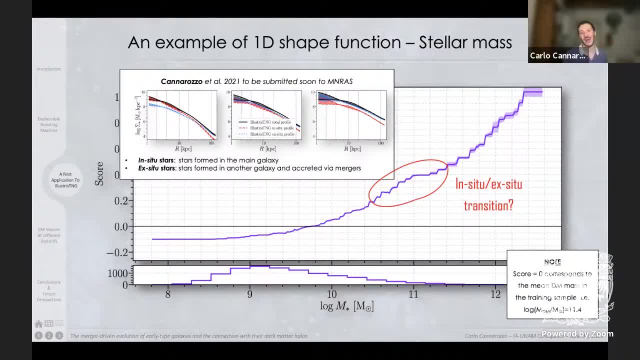 Microsoft researchers of Microsoft research, Rich Caruana and the others, and I think that this method is very promising in this direction. So I don't know, sorry, I don't know this work that you mentioned, but it's something that I can. 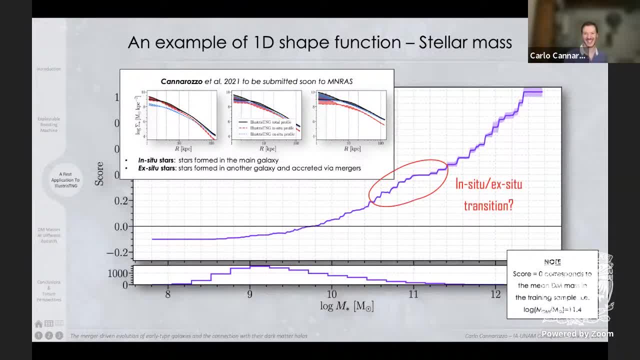 look at. If you can suggest me this reference later, it would be great. By sure, I will send you more questions and thank you for your explanation. And the last question is for Jorge. Yeah, actually I'll be fast because the question was answered, but congratulations for your work. 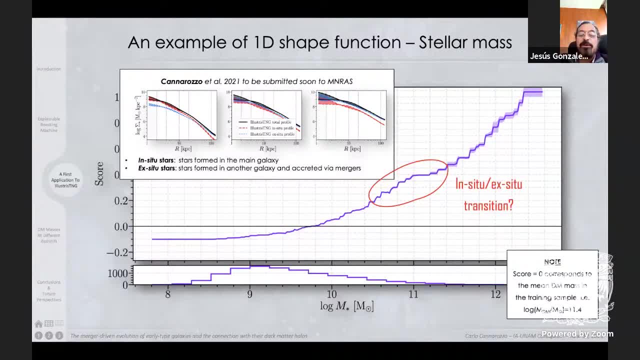 It's very nice and your presentation And, yes, for me, what was asked by Vladimir is the relevance between wet and dry mergers and its implication in the way that the mass sigma relation evolves. But it's a result. so congratulations, Carlos. Thank you very much, Thank you. 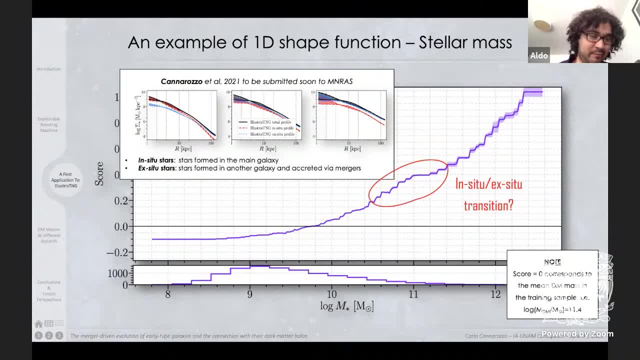 Jorge. Yeah, thank you. Thank you, Aldo. Another question for Carlos. Sorry about that, but I'm having a hard time trying to understand. We know from the nearby universe that there are many relations, many parameters that correlate with the stellar mass, For example. you know? 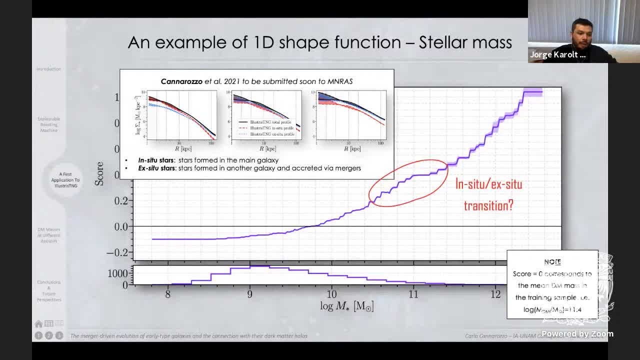 that there is this Star-Form H sequence. You know there is the mass-metallic interrelation. Do you know that it's a strong relation between the gas mass and the stellar mass density? So, and the stellar mass density as well, especially resource relations. My question is: how do you? 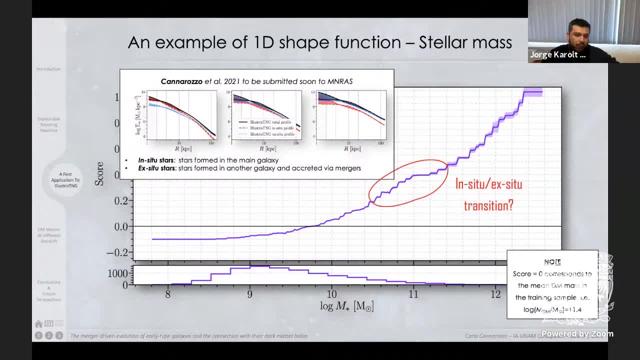 disentangle somehow this strong relation that you observe at the, in the local universe of this, when you try to understand and when you try to derive this mass halo- and this is going, something that you just mentioned it in your presentation of this topic. uh, gretzky is also doing this in. 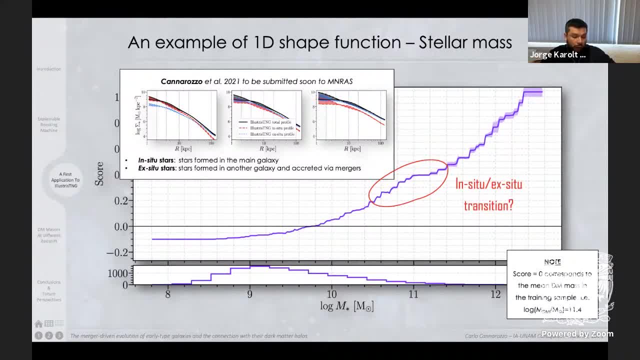 order to understand or derive the metallicity, the gas metallicity for galaxies? no, and it? that worries me because, uh, you know, there is a like- let's call it- cross relation. there's an interrelation between the stellar mass and many other properties and my question is again: how do you disentangle? 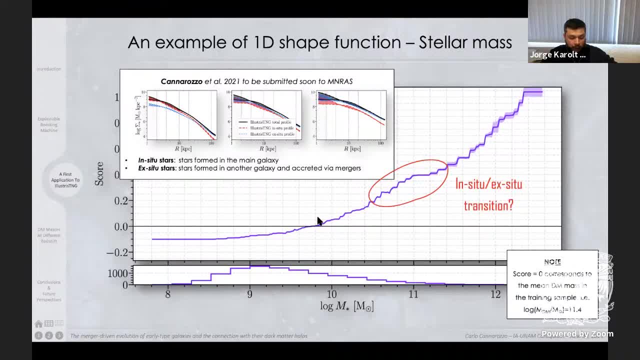 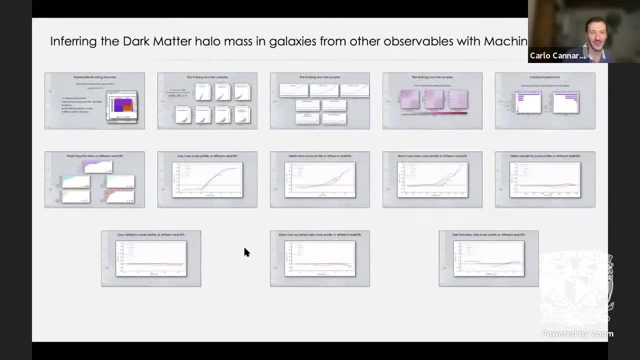 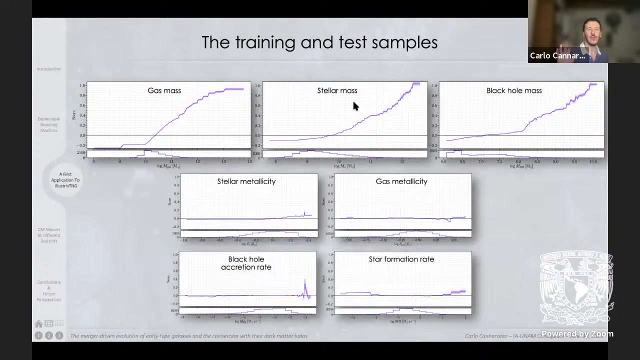 this different scaling relation that we observe in the local universe, uh, in this type of- uh, let's say- predictions from the machine learning, how do you- uh, you know- account for that? okay, if i understood your, your um, your comment, um, actually do you mean if, with this method, i'm able also to reveal 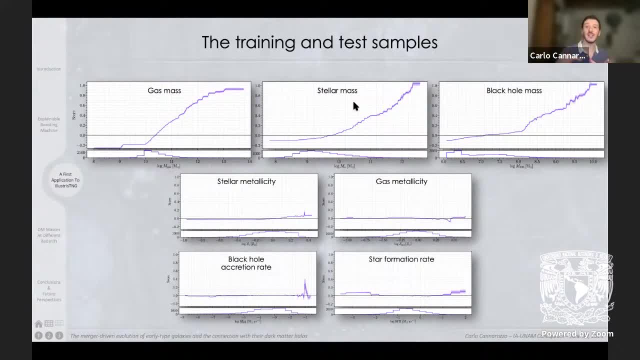 the possible cross correlation between, for instance, the stellar mass and the other quantities to retrieve the mass of dark matter, is it right? so my question is: i mean, you know that's as you're showing in this, in this slide, you you're having um many different calibrated parameters. 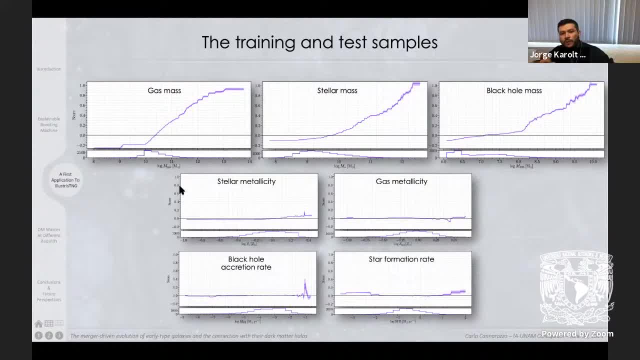 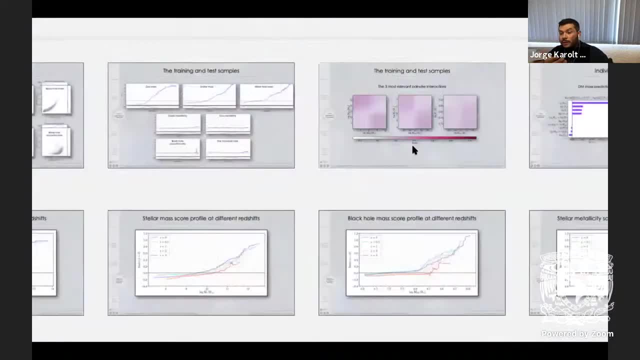 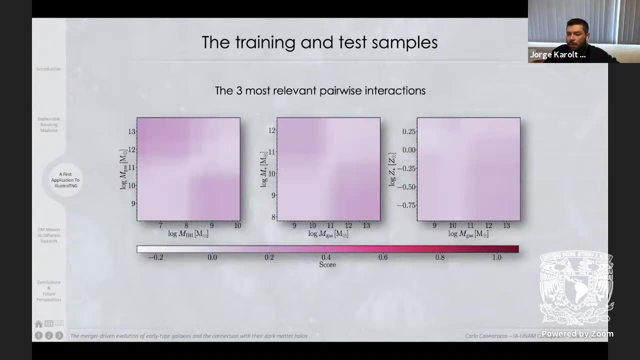 but, for example, if you, if you account for the, for the stellar mass, gas mass relation, right, so in that case, what will be the primary driver? will be the stellar mass or the gas mass. so that that's my question. if you use the same machinery that you are using for estimating mass, halo, okay, 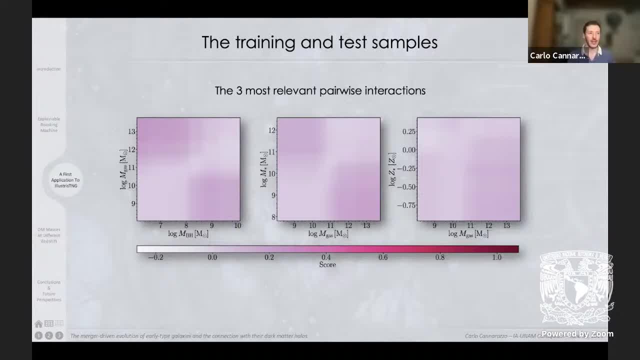 okay, um, the question is: uh, this method works, uh, as, uh, the quantity you want to infer, the mass of dark matter, aliens, you can express it as a summation of the one dimensional functions, the one that i just show you, and also the possible paywise interactions, what these paywise interactions are. 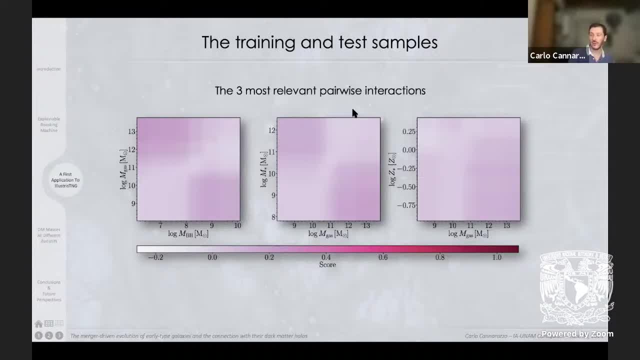 for instance, the three most relevant pay was interaction at a thread. shift zero found in the found by EBM are these three? Let's focus, for instance, on the central panel. We have on the y-axis the stellar mass and the gas mass. 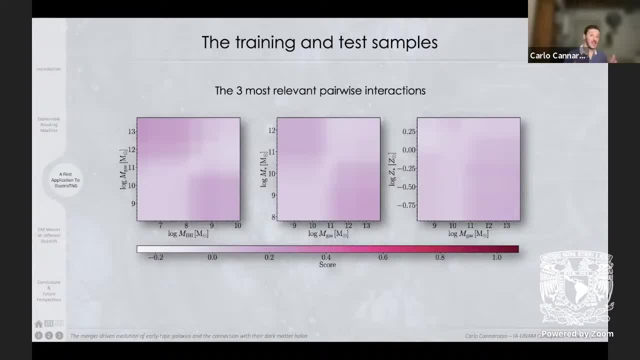 And we know, as you were saying, that there is still a 1D relation between the gas mass and the stellar mass. The next step, thanks to EBM, is that this relation that is still there between the stellar mass and stellar gas. 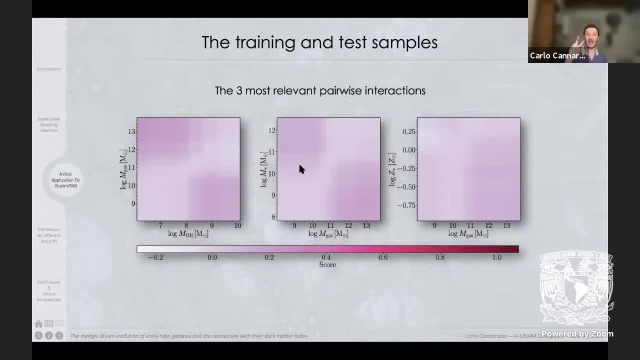 here can be visualized as a two-dimensional function And for instance here, as you can see, is the color. that's a function of the score that I mentioned to you before. In this case, the higher the mass, the lower the velocity. sorry, 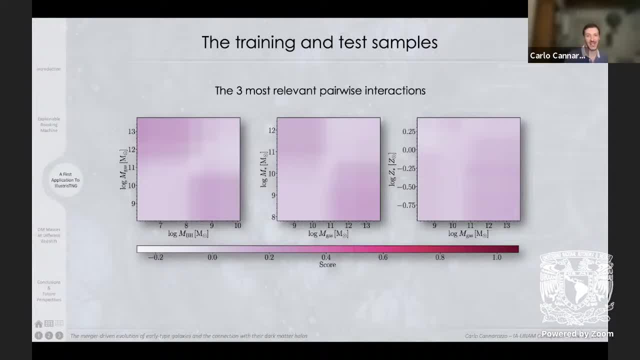 The lower the stellar mass and vice versa. And it basically can understood this in the sense that if you have still more gas, it means that you are not still on the much stars And, on the contrary, if you have more stellar, higher stellar component. 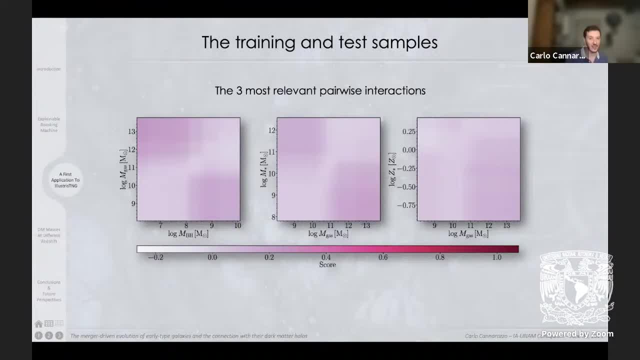 you have a lower stellar mass In this kind of systems. So we are still conceiving how to derive the functional form that, in case, would be a very much complex functional form because, as you can see, should take into account for n possible dimension. 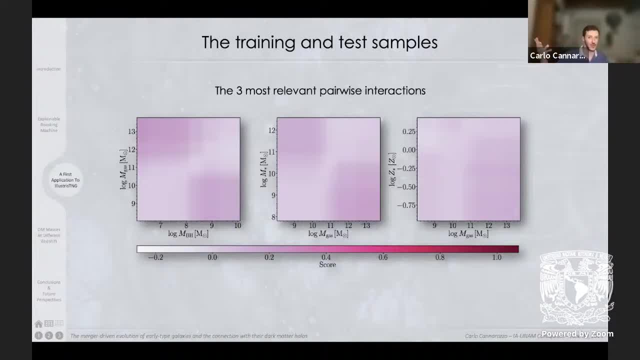 where n is the possible features and pay-wise interaction you are taking into account, But also the existing, you know, relations between, for instance, the stellar mass and dark matter of mass, or the other relation EBM is is able to take into account. 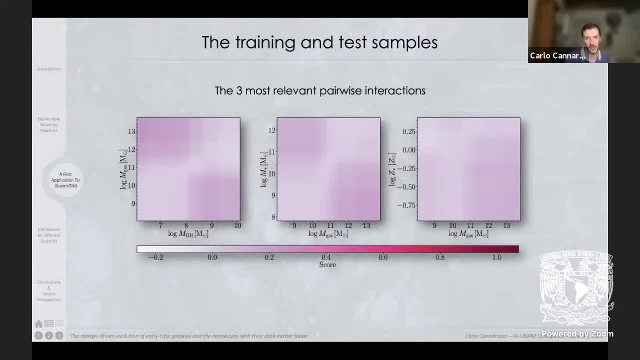 for these existing relation in the total difference of the previous data matter? And that's so. My final question will be: and taking into account So, did the system conducting learning, knows that the least relation between the judges you mentioned, gas, gas and mes? bereanance? 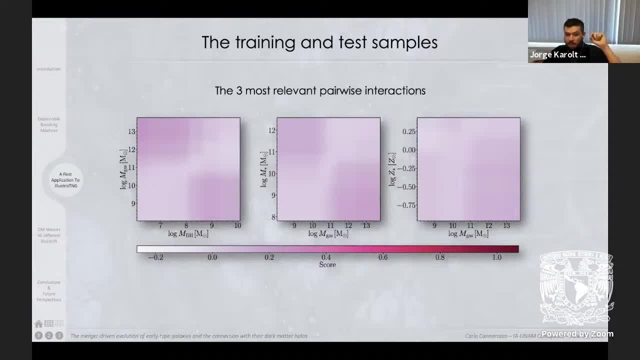 So, knowing that the machine learning predicts that the main driver for estimating the mass halo is the mass gas that the resolution showed before, Is that still? I mean that's still the case? Yeah, but I mean the plot I showed you before. 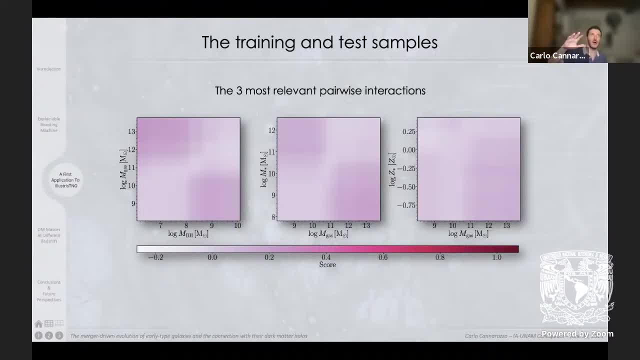 about the overall importance is telling, which is just a rank, which is the best, the second best, the third best, the n best estimators for deriving the dark matter mass. But in any case, all these one dimension, sorry, all these features and also, for instance, 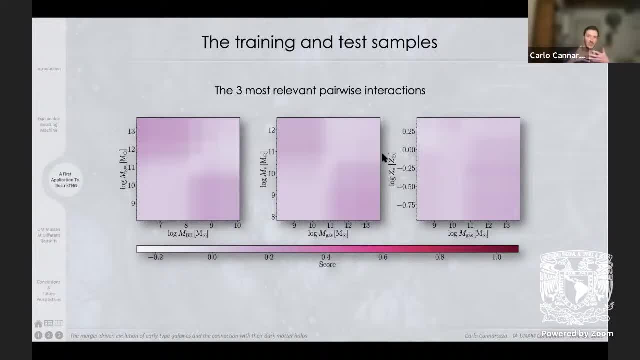 the three most interaction are co-working together for inferring more well-constrained the mass of dark matter. for instance, with respect to an inference made only, I don't know, in the dark matter, no only considering the stellar mass, Because in this case, if you 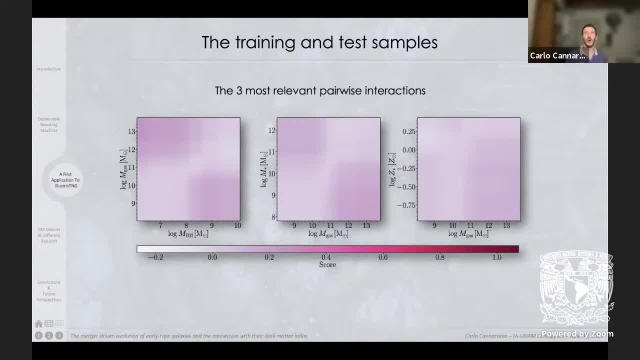 if I made the inference with these means of the third, only with the stellar mass you have, like the stellar to halo mass relation, right On the X is the stellar mass, the Y is the mass of dark matter, But in this case the function you are considering, 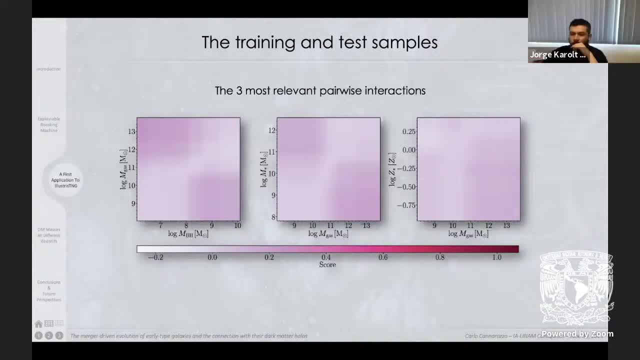 is a much more complex function, Considering at the same time all these features that you are considering and all the n pairwise interaction, where n in this case is a three, because the user- me- sat in this machine that I wanted to consider just the three most relevant pairwise interaction. 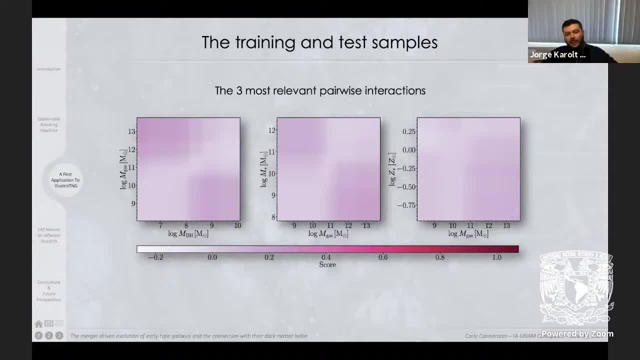 I think that it's a bit unfair. Thank you, Carlo. It's like a principal component analysis, but much more powerful and much more extensive. Yeah, Something like that, Yeah, and much more easier to be understood, I think. But the problem with that is something. 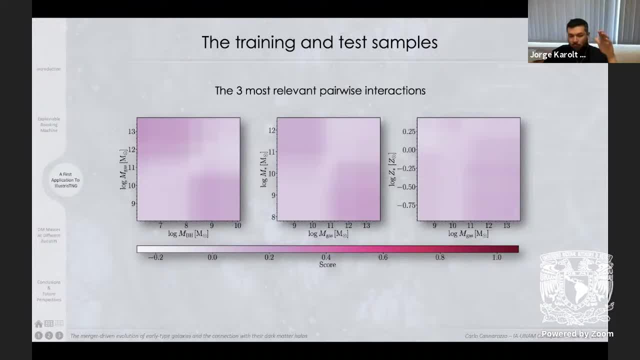 and the reason that I mentioned this is because I'm doing, we are doing- one of my PhD students. she's doing something very, very simple which is quantifying precisely something like this, which is what is correlating the most with metallicity. 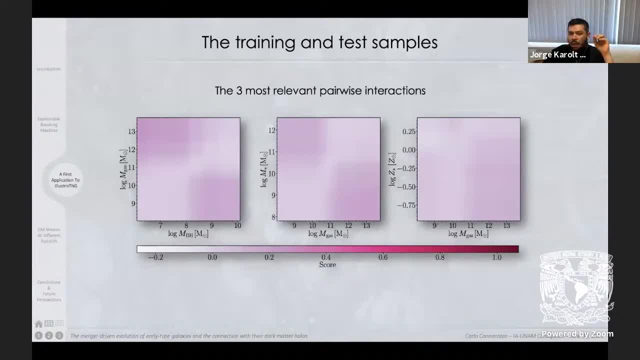 stellar ionized gas metallicity in nearby galaxies And you know you have a like you're showing you have that the star formation rate correlates the, of course, the stellar mass, many other parameters, the morphology and whatnot. 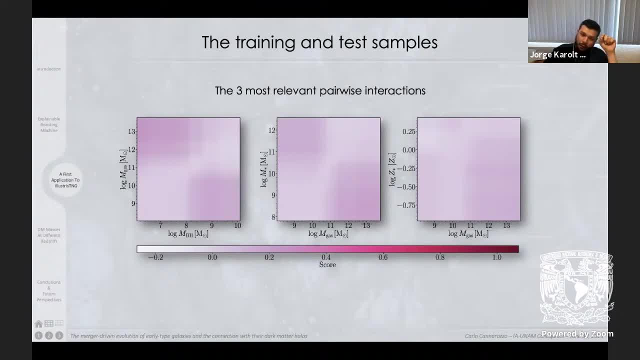 But when you remove this relation between the gas, the gas metallicity and the total stellar mass, all these possible correlations vanish basically. So you don't have any significant correlation between the metallicity, the residuals of the mass, metallicity relation, we are to say, and the star formation rate.